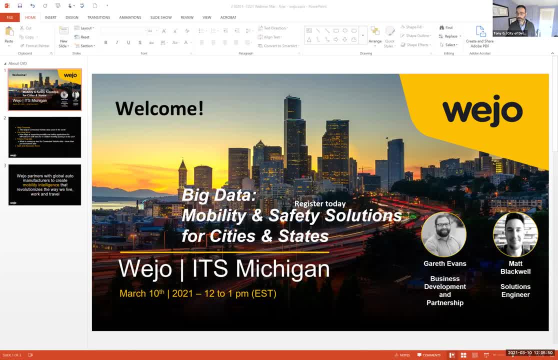 to answer them at the end. so please use the chat feature. Join the meeting. You can just click on the chat item on the bottom and type it in. If you don't see it, it may be under more, so you have to click the three buttons on the right and select. 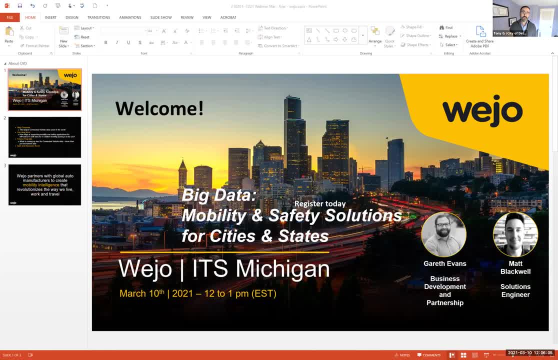 the chat. You can also use the chat from that drop-down menu. Besides that- we're super excited about it- I do want to encourage everyone who's attending to please follow us on social media. We're relatively active and we keep our members. 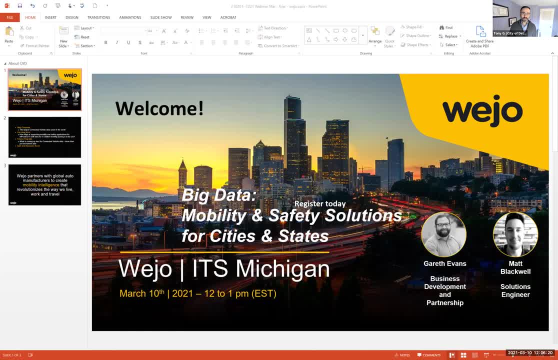 and our friends up to date on the latest details that are happening. We are on Twitter, LinkedIn as a group and also on YouTube. now, I'm not sure about the Instagram. We may be on Instagram, but that's still kind of in the works. 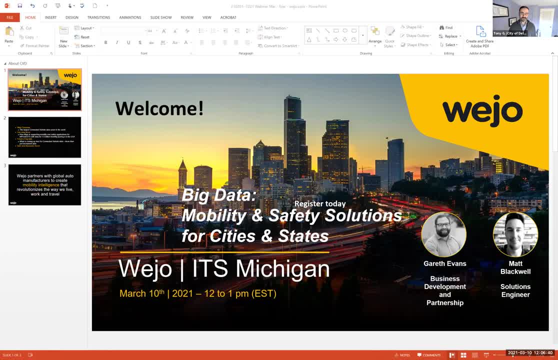 I do want to thank Jeff Feeney, Craig Victor, Belinda Beard- everyone who made this possible here today. I'm sure I may have missed a couple of names. This would not have been possible without them. So, with that said, I'm going to be introducing our two presenters, Garrett and Matt will. 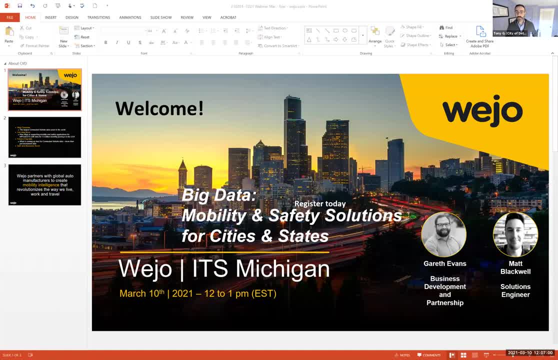 provide an overview of Weejo and how the largest data source of its kind is being used within traffic, Traffic and transportation for use cases in the US. They're going to be demonstrating new possibilities for data assets and insights or supplementing traditional data sources. 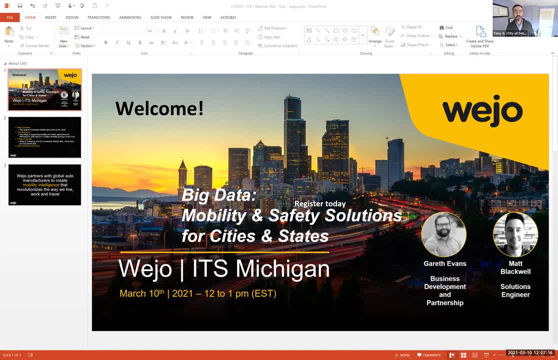 for future implications. Garrett is a VP of sales with data egress team. He has also spent time on the data ingestion side of business, working directly with OEMs to shape the type of connected vehicle data that is and will be available in the future We also have with. 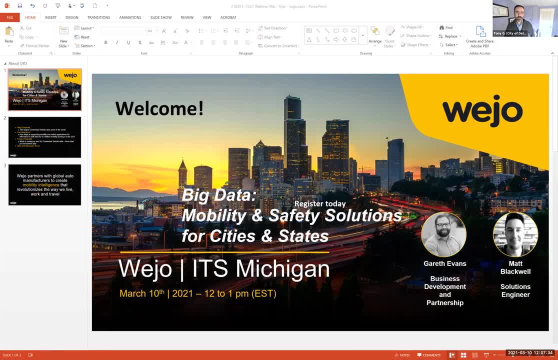 us today, Matt. He's a tenured Weejo employee and he had worked in a variety of roles across the business. He currently forms the solution engineering team, spanning multiple business functions from commercial to technology. His knowledge of applications and uses of connected vehicle. 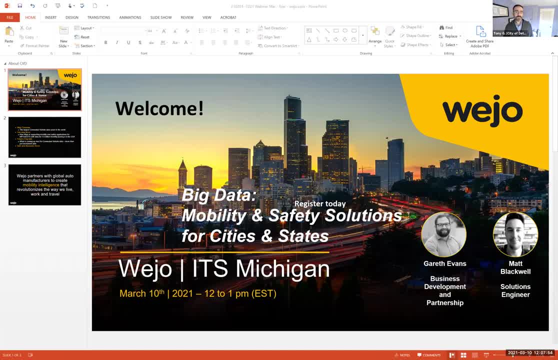 data means that he works very closely with both OEMs and clients within the Weejo pipeline. Thank you very much to both for agreeing to be to present to us here today. We do have a general items to you know, a few items to discuss, but I'll pass it on now to Garrett. 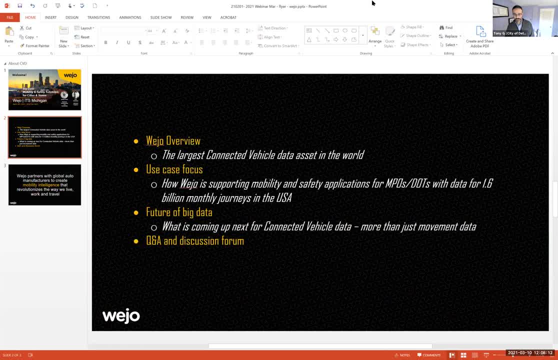 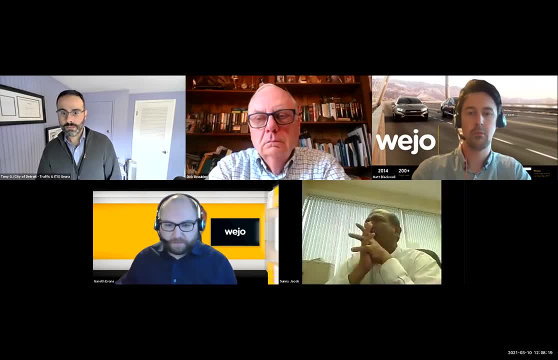 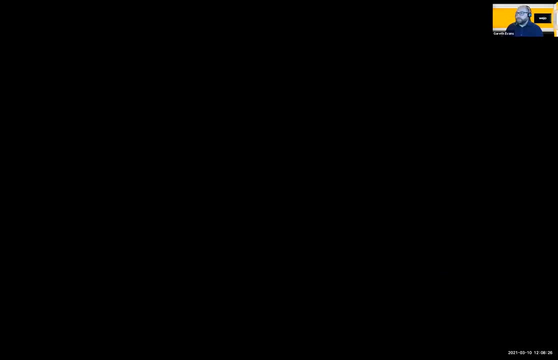 so you can take us through this Garrett to you. Thank you very much, Tony. I will just bring up my screen guys, so bear with me one second. So first of all can I just confirm that you can see that screen, Tony. I'm seeing that. 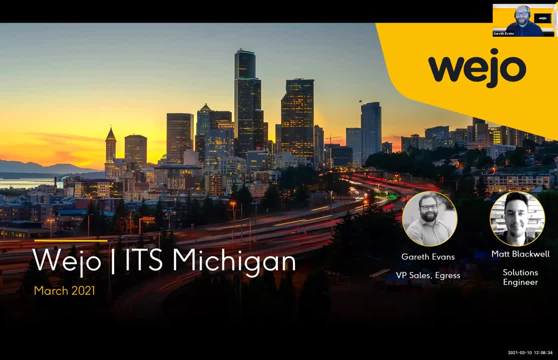 Okay, I'm seeing the nod by Matt, So thank you very much for that. Thank you very much for the kind introduction And it's great to see such a big audience for this. So you know, we really do appreciate. you know there was quite late notice of this actual webinar that. 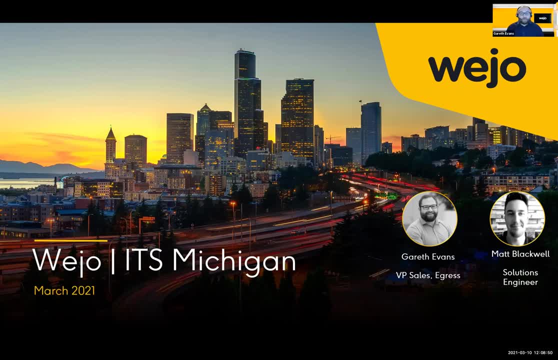 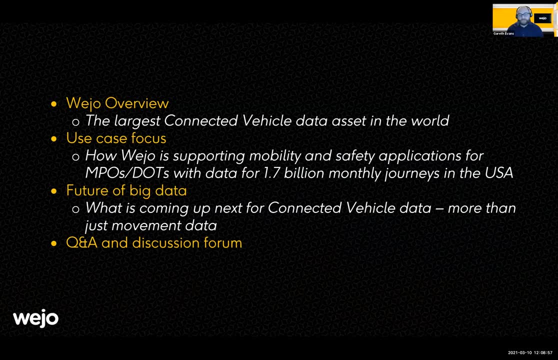 we're doing So. it's great to see such a big crowd. As Tony mentioned, the way that we formatted this session is to give you an overview of Weejo. Who are we, Why are we having this conversation, What do we do and why? We're then going to look into more of a user-friendly 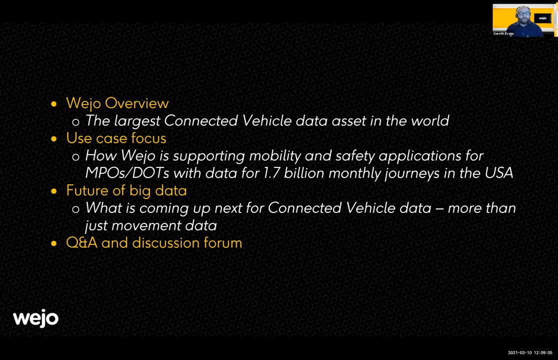 use case focus. So we very much want you to understand and realize where the power of big data, whether it be Weejo or other providers in the market, can actually facilitate the various use cases, And hopefully you know you will always come to Weejo for those use. 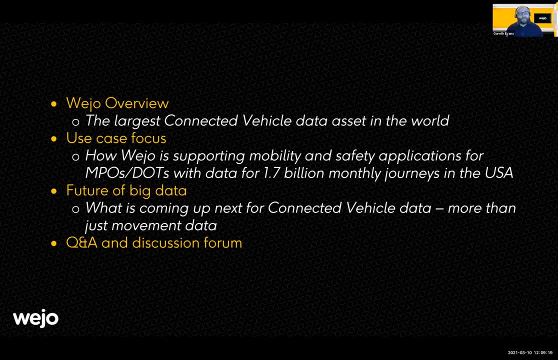 cases, But then also the future of big data. So what are Weejo doing and what are we looking for in the next few years and how can that data be applied? And a big part of these sessions is very much the Q&A and that discussion forum. So a few weeks ago me and Matt actually delivered. 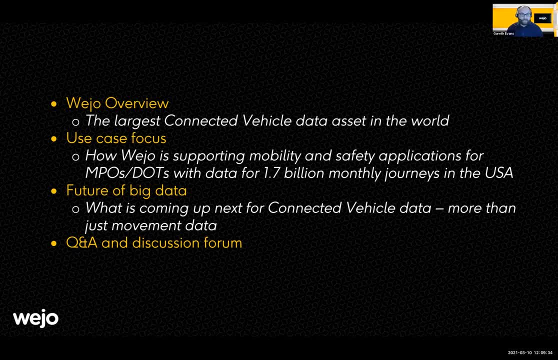 a very similar presentation to ITS Midwest And the majority of that session was very much a Q&A session, So people can really learn and understand the power of Weejo data and how it can be utilized across various use cases, across various different markets and sectors. 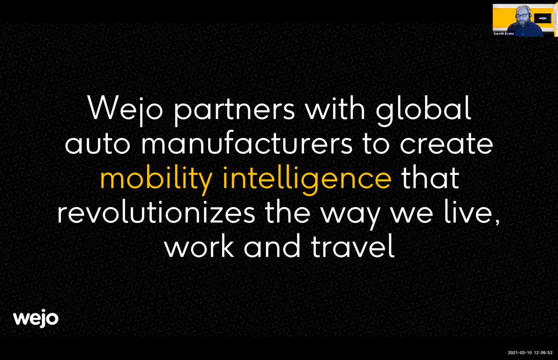 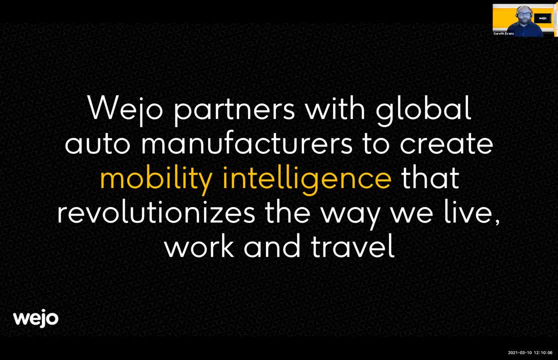 the side of the roads. So we don't have hardware, We don't have the software that's embedded in those vehicles. Where Weejo obtains the connected vehicle data is through exclusive partnerships with the global car manufacturers, who I'll refer to as the OEMs. as we go through this, 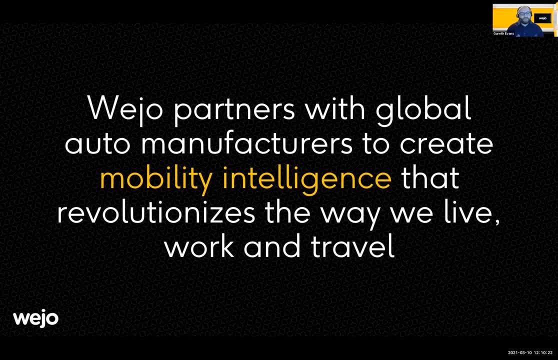 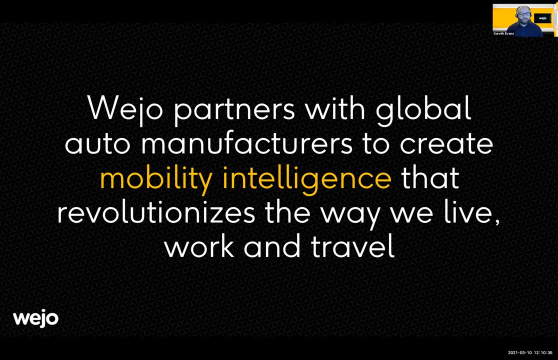 go for this presentation And it's through these exclusive agreements across the various OEMs that gives us the power of this data And where Weejo sits within that landscape is essentially the facilitator from a global capacity to bring all of these car providers together, turn the data into. 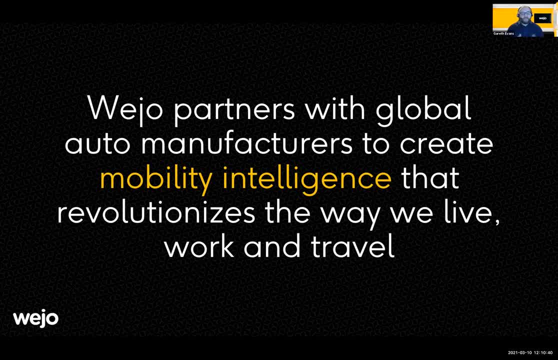 a single common data model. So people like yourselves, when they're trying to access data, you don't have to go through several different sources to obtain this connected vehicle information. So I'll start off with some big numbers And, as I go through the next few slides, 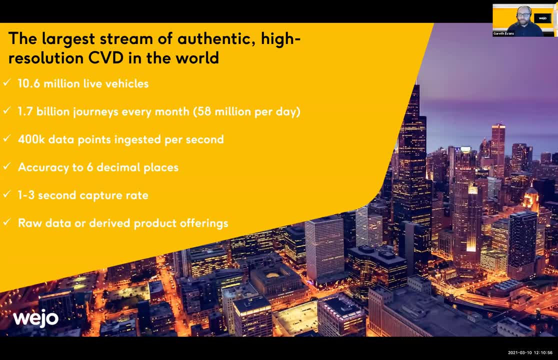 I'll start to break down some of these big numbers. So at the moment currently live in the het facility in London with mostly 1.6 million of our use cases of diversity, over 1.6 million vehicles, And that equates to roughly about 1.7 billion journeys every single month. 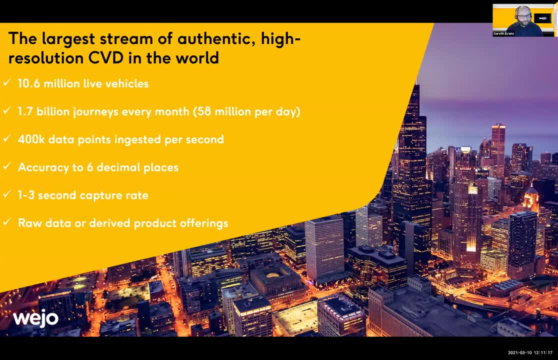 At our peak we see about 400,000 data points ingested per second. The data accuracy is down to six decimal places. So for context, that's roughly about three meters square, So we are able to get down to lane level, also parking bay level accuracy, so we have use cases that're. 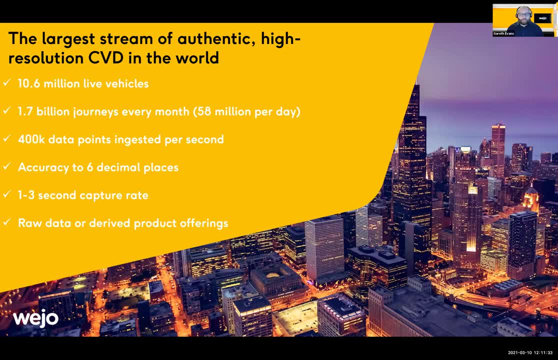 of use as well. The data that we capture from the vehicles is every one to three seconds- and again I'll allude to this in a bit more detail in a few more slides- and we have a combination of what we call our raw data and our derivative data products, and then, just for some further context, guys. so 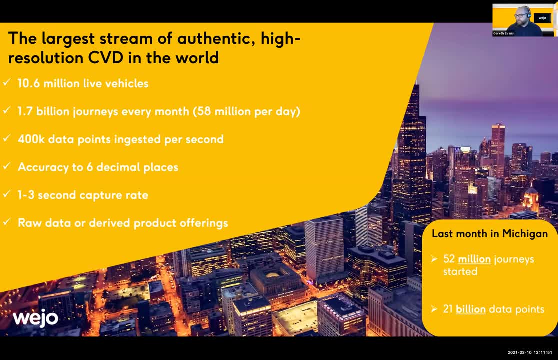 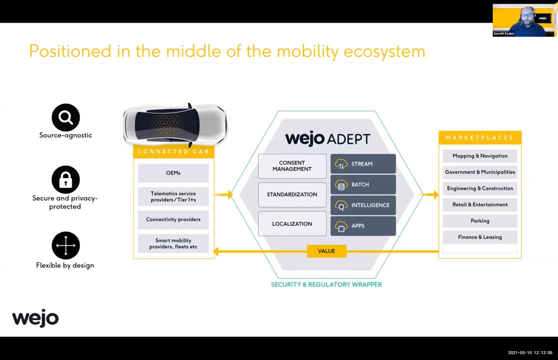 last month in Michigan, we saw data for 52 million journeys that actually started in the states and that was roughly about 21 billion data points last month alone. So in terms of where WeJo is actually positioned and how we operate, we collect the data from OEMs and tier one providers, but 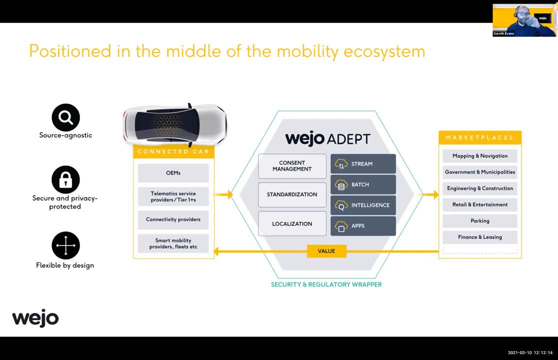 excuse me, guys, one second, sorry about that. and so the connected enabled vehicles and the tier one providers. we obtain that data that is then provided to us by the OEMs and tier one providers, and we obtain that data that is then provided to us by the OEMs and tier one providers, and we obtain that data that is then. 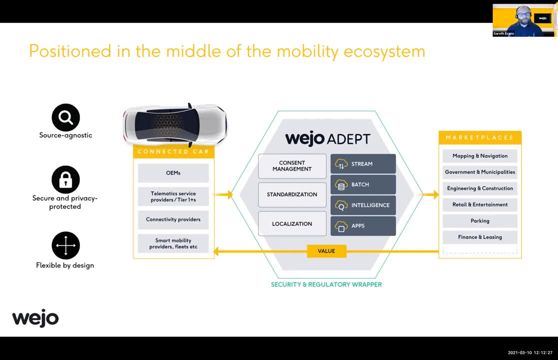 processed through our ADEPT platform. so this is WeJo's proprietary data platform, whereby we cleanse and harmonize that data and then facilitate the marketplaces. and the marketplaces vary, so we work directly with state entities, city entities, at all various levels, but then we also work very closely with various different private and public sectors. so our use 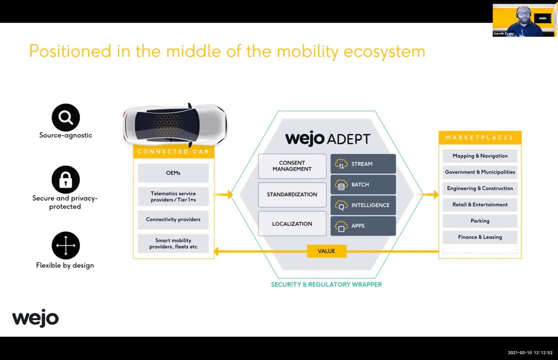 cases can range from looking at traffic and safety initiatives from the DOT perspective to mapping and digestion companies all the way over to the retail sector whereby side location, and we're helping from an origin and destination perspective to understand the actual demographics of the people coming into the areas and where they're coming from. So we absolutely span. 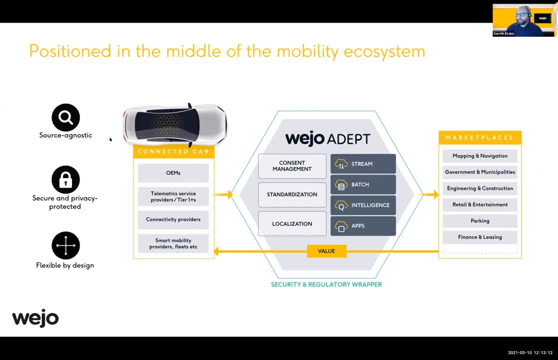 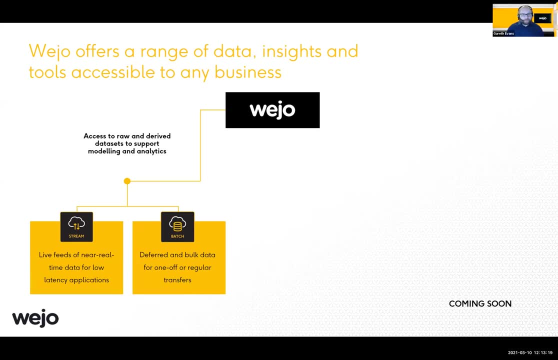 across an array of use cases. So, as I mentioned, we receive the data every one to three seconds. We do have the capability to ingest that data, run it through our data critical centers, systems andTOCK. we do have the capability to ingest that data. slip through our DSMs, as well as the reason why we're meeting with. 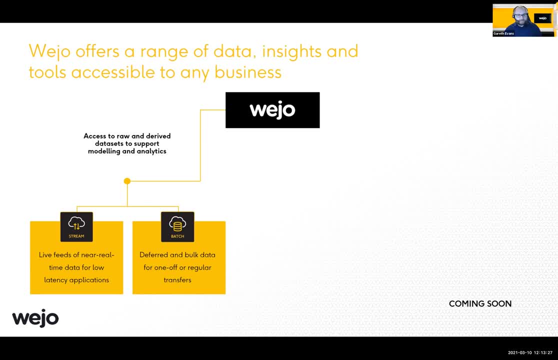 our adept platform and have that data available to end users in what we describe as a live feed, and this is actually available in less than 60 seconds. so that is data from the vehicle into the wejo platform, into the hands of the end user within 60 seconds. we absolutely appreciate. 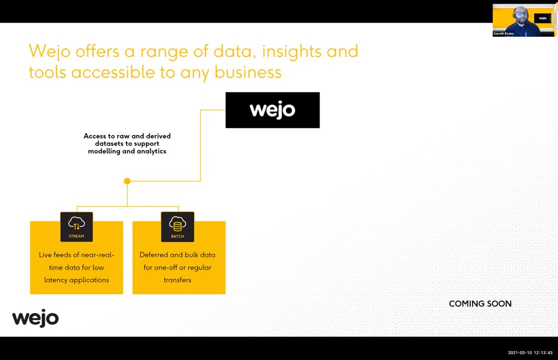 that. you know that sounds great, but not everyone needs or has the capacity to ingest data on that scale. so what we also do is we can provide derivative bulks of data, um, whereby we can go back up to up to now, about 22 months. matt. matt can shake his head or nod: if i'm, i've got that. 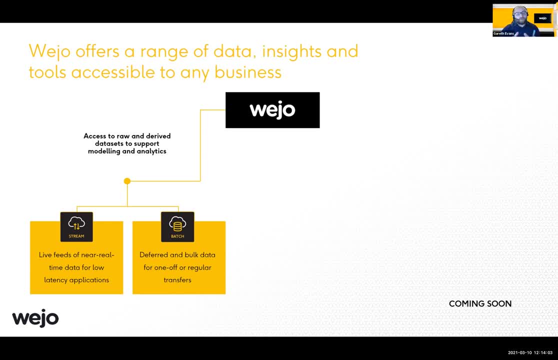 figure wrong, but we can go back and what we describe is we can absolutely look at. you know what was happening during covid, but we can also look past. you know back further than that. so around about um may 2019 with all of our data. there's no restrictions on the. 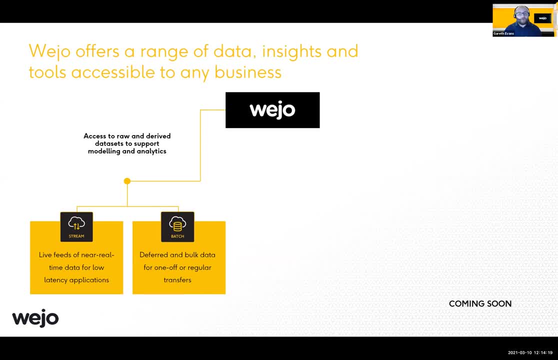 scale of the data that we provide. so we can provide derivative bulks of data and we can scale um in terms of being able to transport and offload that to people. so if someone was looking at one section of road and they only wanted one hour of one section of road, in theory 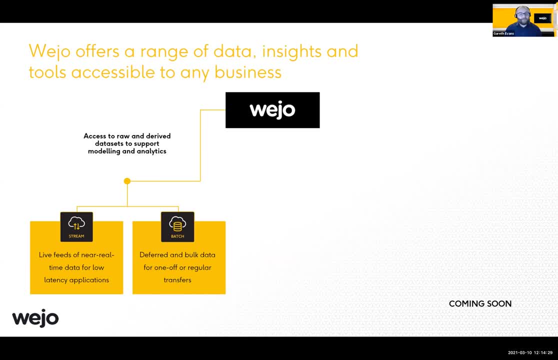 we could absolutely provide that. if someone was looking for the data for the entirety of the united states for the last two years, we could also provide that as well. so there's no limitations in terms of our um, our bulk data. but again, we appreciate that all this data is great and 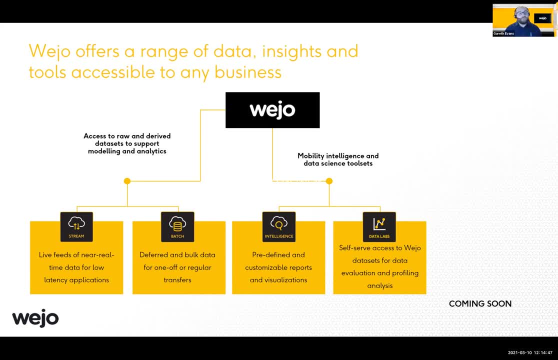 big data is absolutely fantastic, but it means absolutely nothing if you can't utilize it. so, as well as our big data assets, we also have defined products and customizable reports that fall underneath our mobility intelligence suite, which again, i'll go into in a bit more detail, but essentially these: 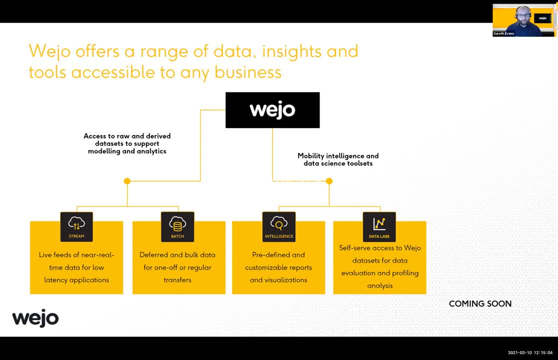 are derivative data products which are much easier to ingest. so, rather than worrying about billions and trillions of data points, we can formulate more condensed um, aggregate to these data and provide them in an easier to digest format. we do also have various platforms where people can view our data and experiment with it, and almost 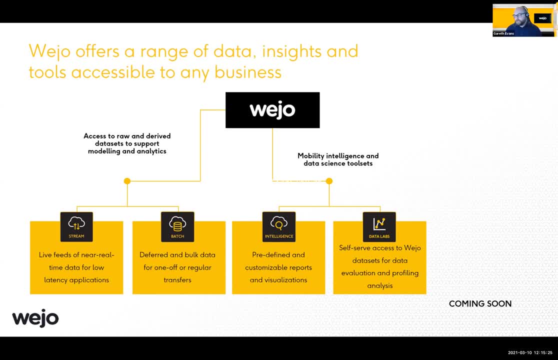 give it a test drive, as it were, before you go into the big data platforms such as our data labs environment. so there's full transparency of how dense our data is for the various locations and the various use cases you'd like to explore before there's any licensing of the data. 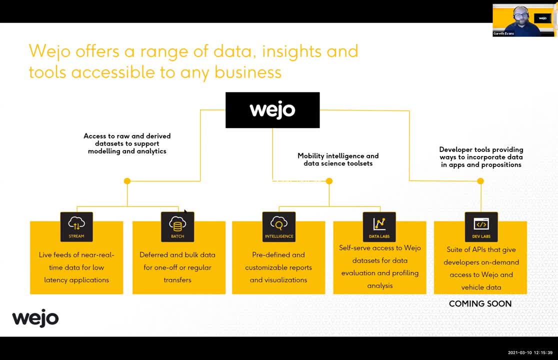 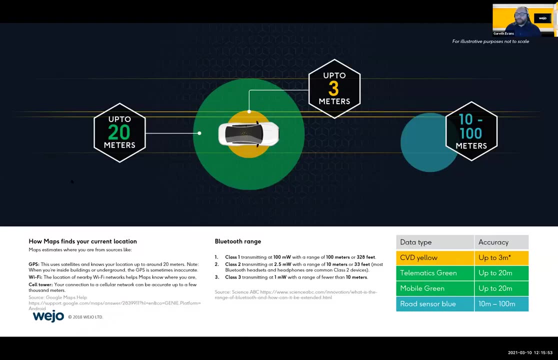 we are also in the final stages of developing our suite of apis, where we'll have more on-demand access of our data. so we're probably looking at about q2 to q3 when this is available. if you do have any questions, feel free to add them to the chat. so a big question that we get asked is: well, you know, in terms of the 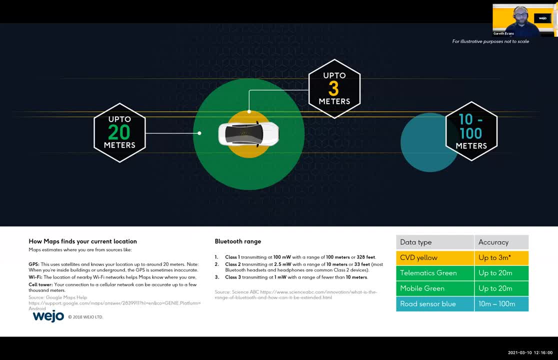 data accuracy. how do you get down to six decimal place accuracy compared to other types of telematic providers? um, ultimately, you know the, the, the technology in this vehicles. it's embedded at the factory level floor, so that means the parabolic aerial and sim gives us a much greater 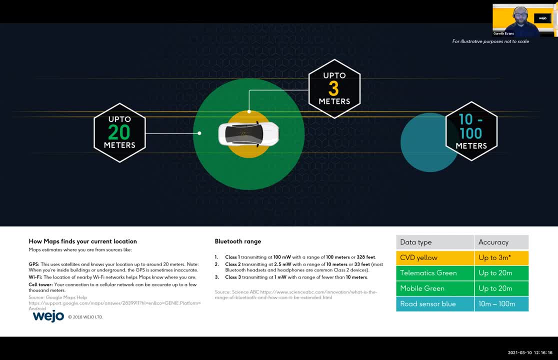 accuracy with our data versus the types you know for- on onboard devices or aftermarket devices or mobile phones, for example. essentially, the power that is generated from these units and the more advanced technologies that can fit with these vehicles allows us for much greater accuracy, and so what we also are very aware of is, you know, 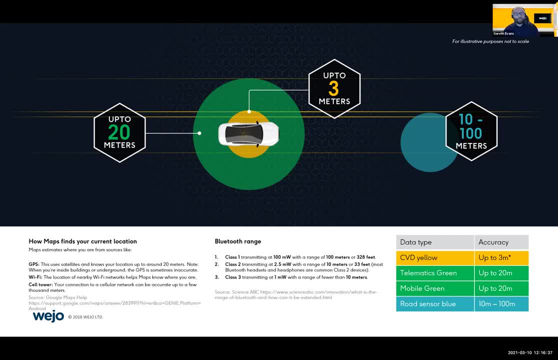 when it comes to either roadside data or roadside cabinets, and they're collecting that data. you know, ultimately, this: you know that level of granularity and that level of accuracy is absolutely fantastic. the challenge that you have with those is you only know where, though, you're near the information. 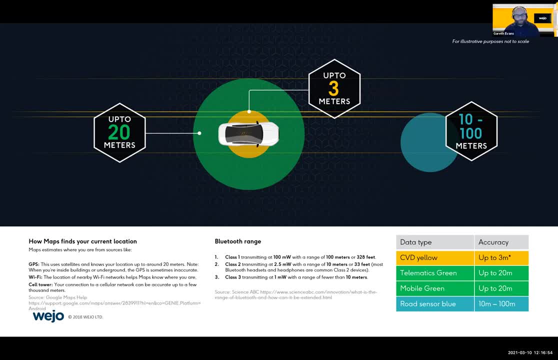 where those are located. so, whether you've got a um, you know a curbside data point collection, whether it's cctv footage, they are fantastic, but you only know the data that those are actually looking at. and what we do, they can do- is provide more of that contextual picture. 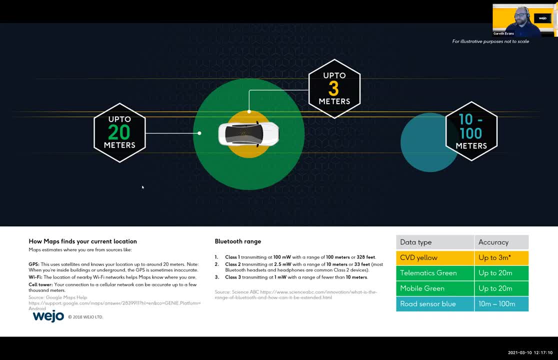 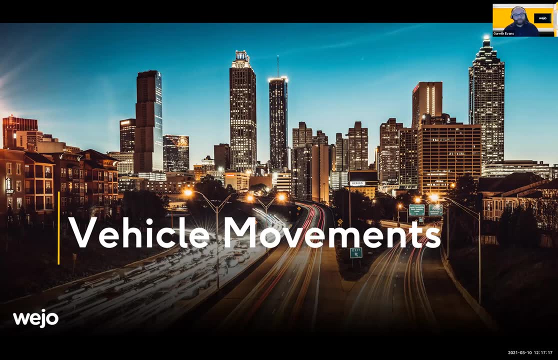 and i'll explain what i mean by that in a few more slides. so we describe our, our data at wejo and wejocom as flavors. so the two flavors of data that we have is our vehicle movement and our vehicle events. so first of all, i'll take you through the movements. 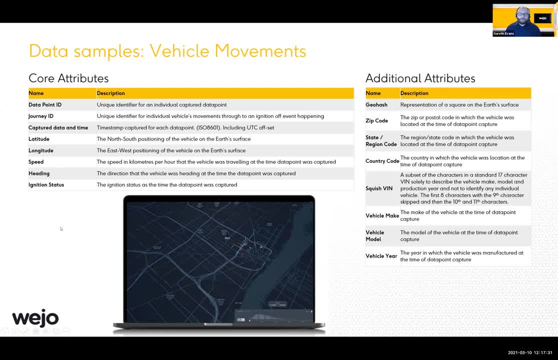 so, in terms of the, the data that we collect every one to three seconds, um is everything that you can see on the screen here. so, as i mentioned, we get longest in latitude, down to six, most all places, but, very importantly, we also get the speed and the heading of the vehicle as well. 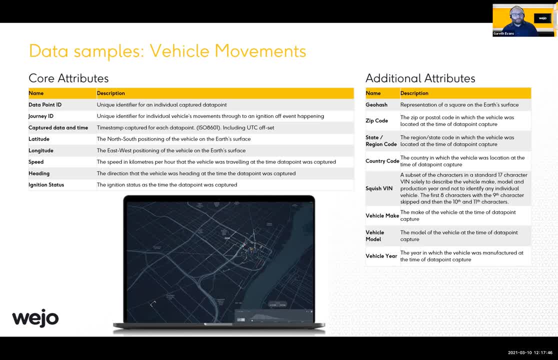 so what this allows us to do is to make sure we're in those data points, we have the origin and destination and we can actually look at these trajectories of these vehicles during the journey from the origin to destination. the reason that we are very clear and we know the origin and destination of these vehicles: 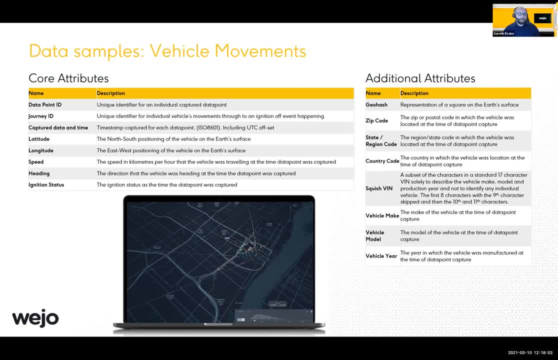 is, we get the ignition status, so we categorically know when the vehicle has started and when it's ended. so then there's no ambiguity from that data. there's no guesswork with the data that wejo provides. we are not making assumptions. is it 17 people on a bus where we think? 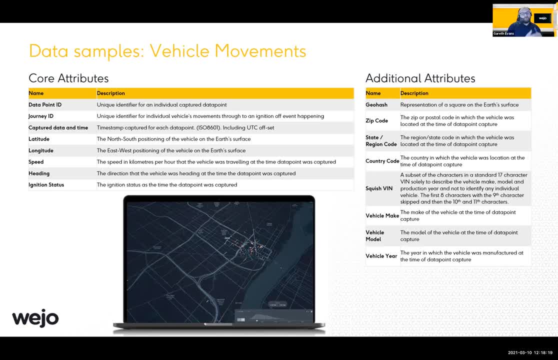 yeah, we're not thinking is. is someone that's on a road bike who's going 10 miles an hour is slow moving traffic. we don't have to worry about this. the data that we have is categorically a vehicle, and we know the origin and destination element from that as well. a key question that we 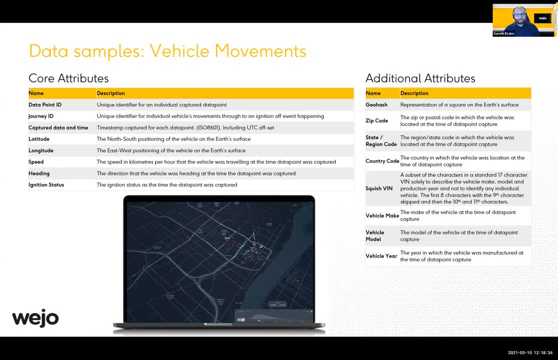 do get asked is um the level of privacy and you know how do we obtain this data from the oems? um a key element of what? what we do- and i'm sure this will come from the questions- is we are limited and know of the actual user of these vehicles, so wejo can only get down to the make, model and year. 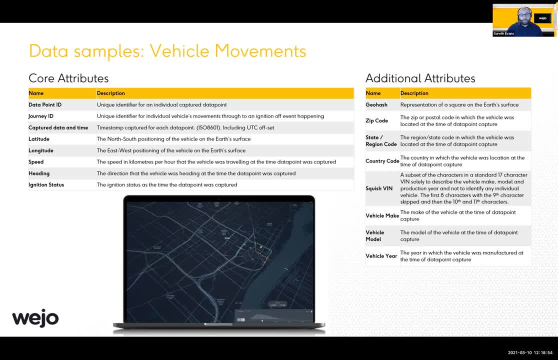 of the vehicles. we categorically do not know the end users and we're not a part of that discussion. so the data that wejo obtains is only data that has been granted access by the owner of that vehicle to that car manufacturer and then subsequently to wejo. um i'm i always like to. 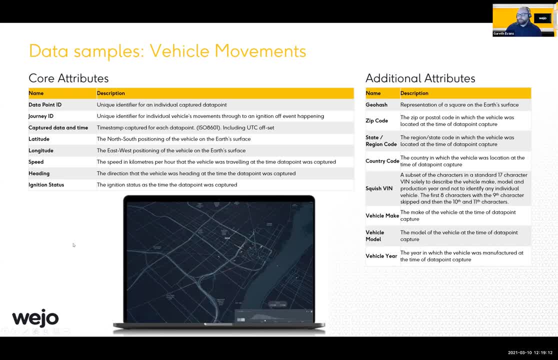 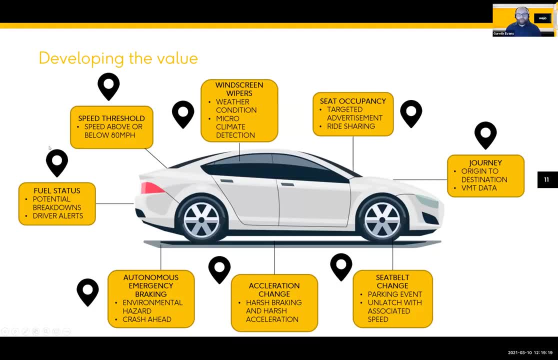 elaborate on that because i'm sure it's a question that might come up. and then the other um that we have is, as i mentioned, is our driving events. so this is almost another name of the, the, the sensors that are in the vehicles or the events that actually occur within these vehicles. 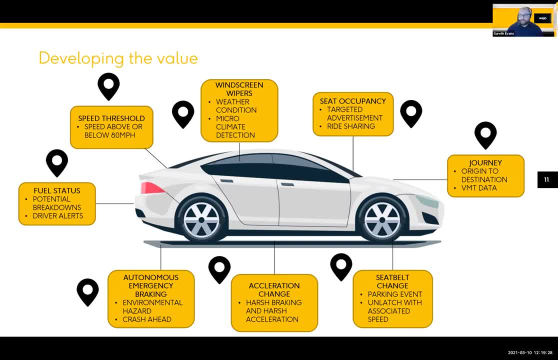 as well, so i won't. i won't name everything that you can see on the screen here, but you know we have key indicators so we can start to go into different exciting realms of use cases. so, whether it be that weather and climate, or knowing the automatic windscreen wipers coming on the external, 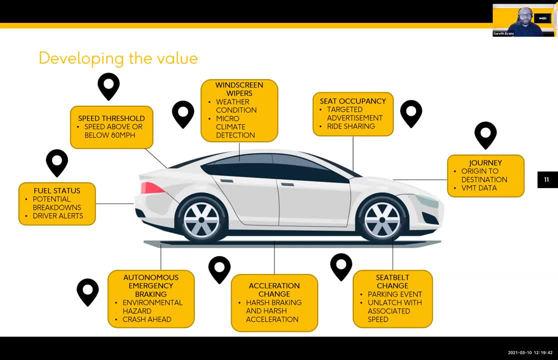 temperature. if we're looking at um seat occupancy- so we get front seat occupancy and seat belt status drivers, which has been widely used in toll lane analysis and diamond road analysis- we can start to look at a safety perspective. So looking at autonomous emergency braking, or actually the harsh braking and harsh acceleration. 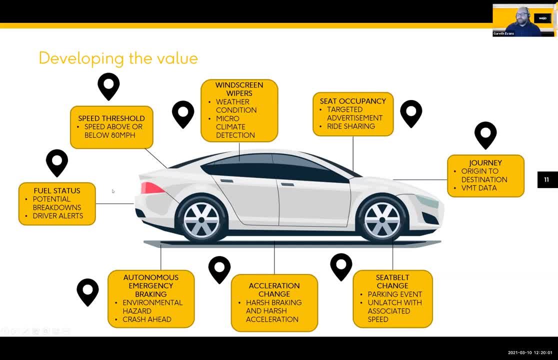 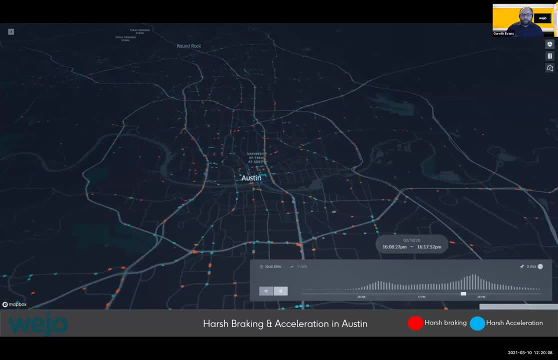 that's occurring in the vehicles, And it's that last point that I'll just pick up on in this clip here. So this is actually data from our vehicles whereby, to the millisecond timestamp, to six decimal place accuracy, we can actually see events occurring in the city of Austin over. 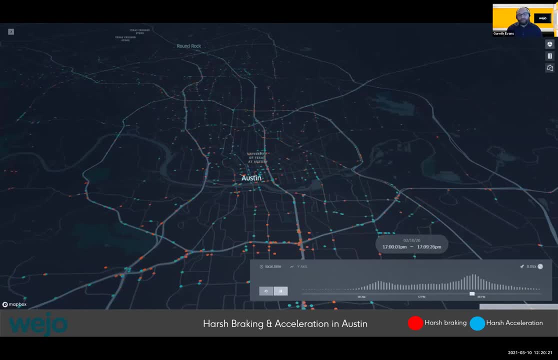 the course of the day of events, of a harsh braking and harsh acceleration. So this is why I mentioned before that sometimes our data can help provide a much more conceptual picture of what's going on from the traffic in that area. So, as an example, did the city of Austin know, on this road alone, every single day there's 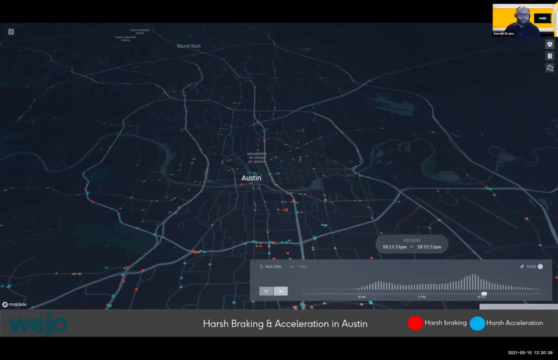 180 instances of people slamming their brakes on- Potentially not Maybe- at this intersection. they did because they've got some CCTV, The footage right there that intersection. but how are they looking conceptually at the rest of the city? If they have got expensive infrastructure that they put in place, how are they forming their 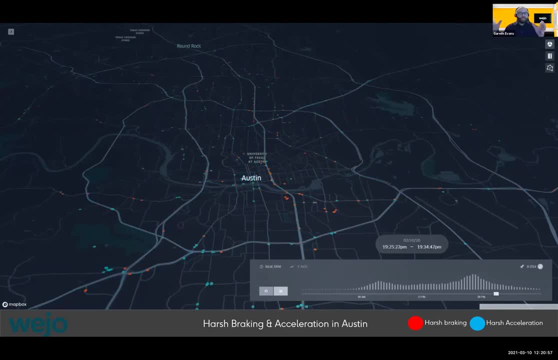 decisions where to put these either roadside monitors, the CCTV footage actually in the cities. So in some cases, we Joe's data is absolutely being used in isolation And in other instances we Joe data is actually helping and supplementing the data for the. 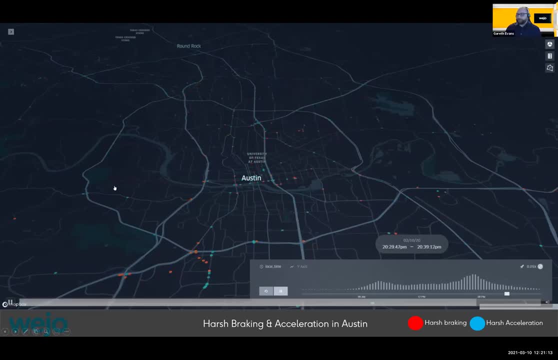 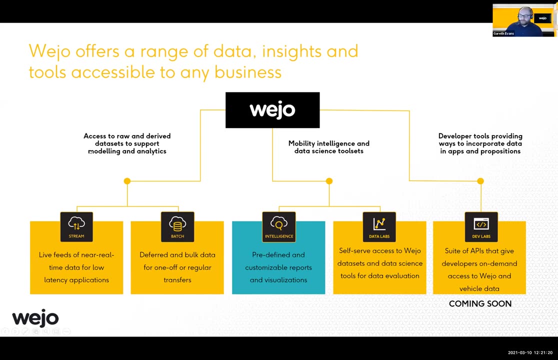 towns, the cities, the agencies, et cetera. And then, finally, I'll just touch on our derivative data points, sorry, derivative products. So, as I mentioned, we're we very much understand that ingesting all these billions and trillions. 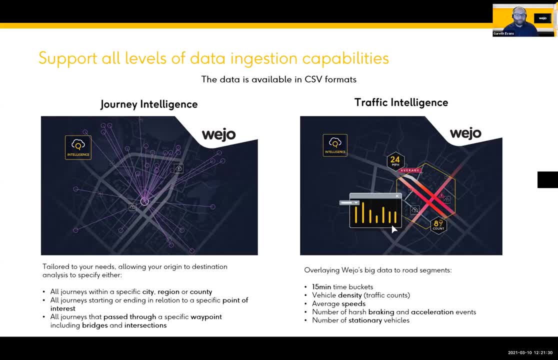 rows of data is great. If you can't use it it's no good to anyone. So we are developing on a wider suite of derived products, but to that I just highlight on this call is our journey intelligence product, which is very much our origin- to destination. 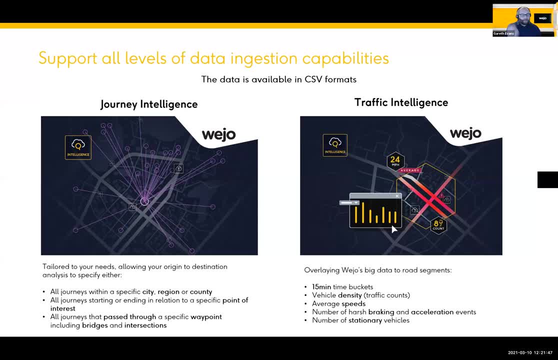 It's an analysis product whereby we can look at two points or maybe a pass through filter on a road segment, and we can provide an easy to digest format of data whereby our traffic intelligence what we have done this. we've used our data as that foundation, but we've overlaid a weed, Joe. 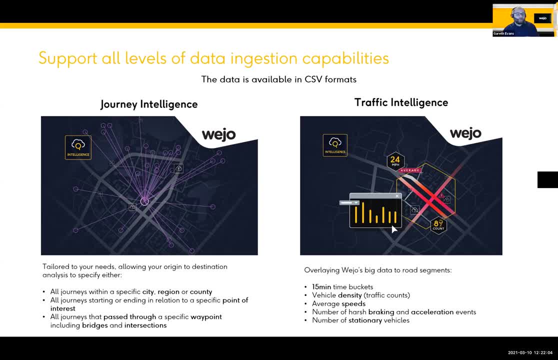 segmentation model, using um, overlaying it on the open street map segmentation model, Cause we know it's widely used and we've broken this down by 15 minute chunks of time, Um and in those road segments, at 50 minutes Of time we can start to look at the numbers of vehicles, the average speeds, the um, instances of harsh. 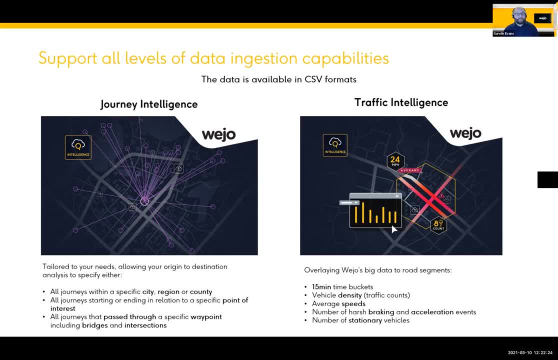 braking and the instances of, of of harsh acceleration, and also the state uh, the stationary traffic as well. So what this allows users to do is ingest that as a CSV format um plug that into the ArcGIS or the um the. 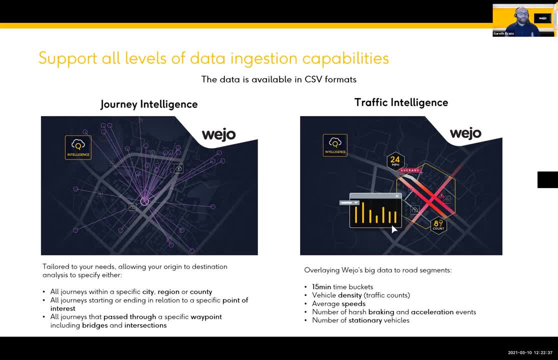 power BI tools, whatever it might be, but it's much easier to ingest. It's not to do absolute fine level of data at 6,000 point accuracy. Well, it's a, A derivative product whereby people are using this especially. we've seen really big uptake on this in the last 12 months, you know, due to people not being able to get out on the, on the, on the roadside, due to COVID and then restrictions that they've had. 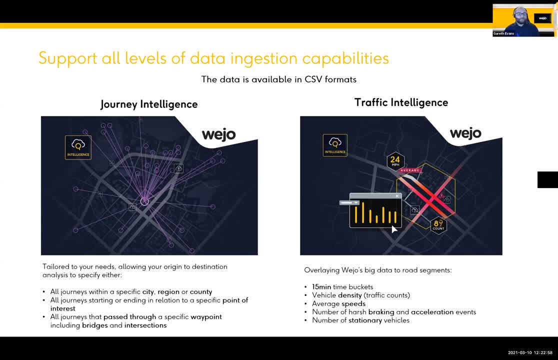 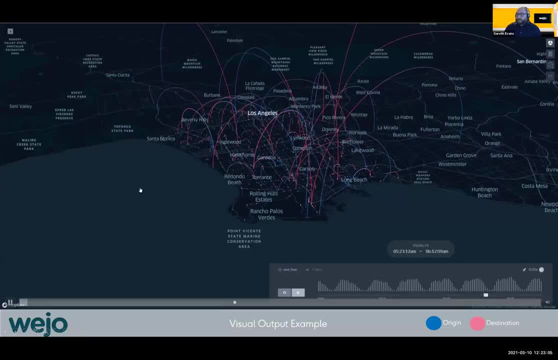 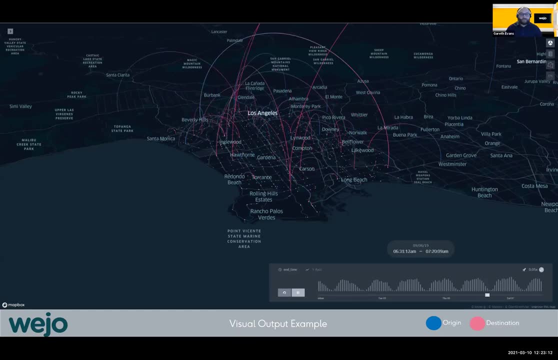 And this has been an absolute um lifesaver in some instances, whereby people can get this data in that they just couldn't obtain before that. And again, this is just, you know, an example of output um whereby you know, plugging in our um journey intelligence. 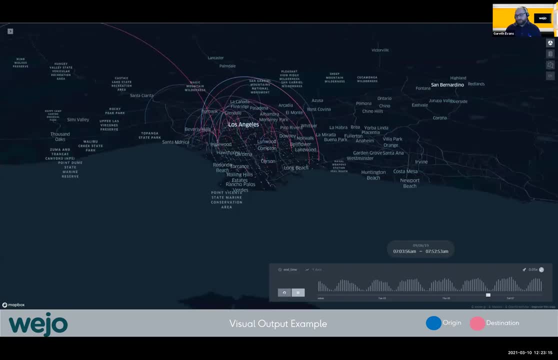 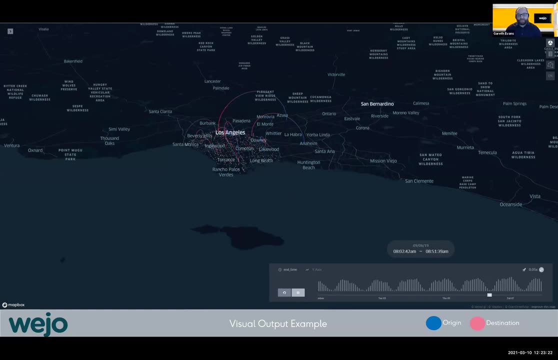 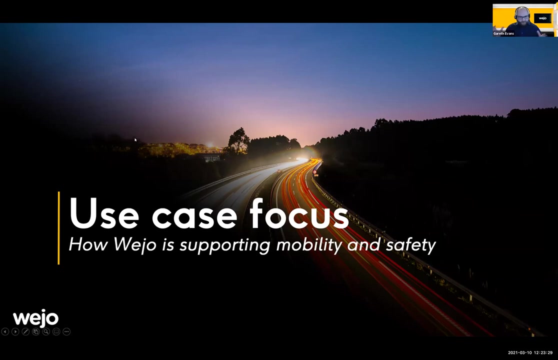 Uh data into a visualization tool. So this is run on a three uh on a, on a free software called Kepler And this, just you know, indicates just how we can start to look at that origin destination perspective. So that is the Ouija overview. that tells the story about what we do and how do we do it. 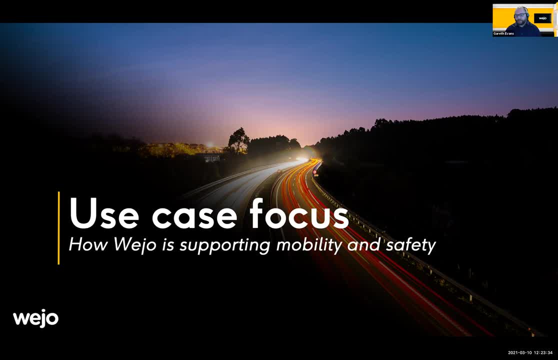 And, um, I'm very happy to hand over to Matt that will go into more depth of the various different use cases, uh, for mobility and safety. That's Gareth Yep. Pleasure to be here. Good to speak to everybody. 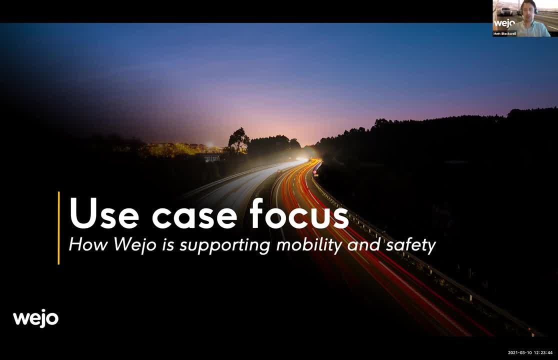 Um, thank you. So you know, we speak to a lot of agencies, um, and a lot of major municipalities who typically will break their applications down into kind of one of one of probably typically two spaces. You've either got the operation side of things and the planning side of things, but obviously, within those applications you've then got specific use cases. 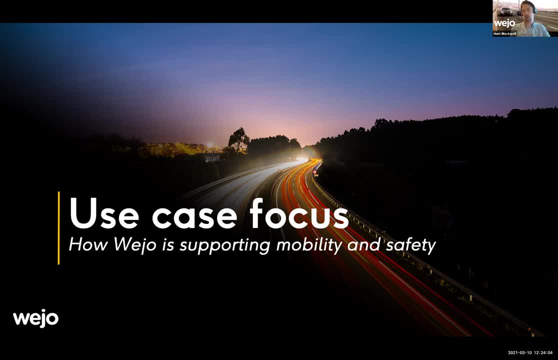 Now, those use cases could be something like signal timing, optimization, turn count ratios. that you know it's not an exhaustive list. What we've brought together here is just a few examples. Um of you know the the actual data visualized, um, as we've already seen, 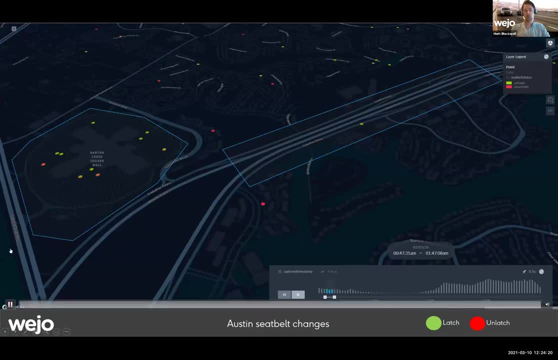 So this first one here represents, um, you know, something that's very, very close to a lot of agencies, which is around the kind of vision zero initiative. So what this is essentially looking at is uh seatbelts, uh usage, or seatbelt latch and unlatch along the kind of major, um arterial roads. 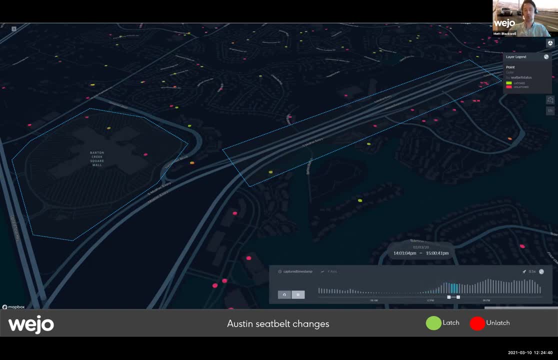 And also because of the fact that we couple the seatbelt usage with the speed of the vehicle. You know we can Actually look at. people are having instances of unbuckling their seatbelts at quite high speeds. um, in some cases, 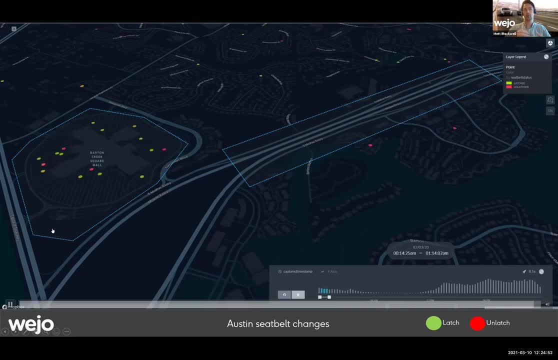 And again, we're very cognizant of the fact that a lot of cities will have to conduct um kind of yearly uh counts of seatbelt usage, Typically, that's, you know, done by I. so we can actually start to look at drive uh driver seatbelt usage here. 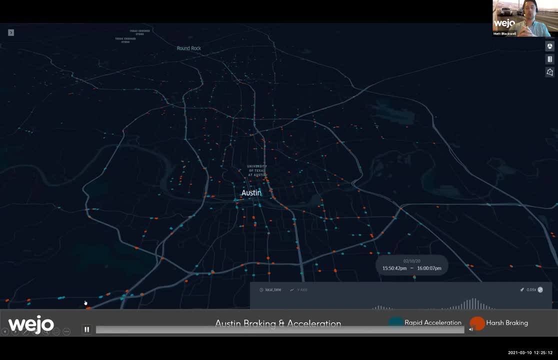 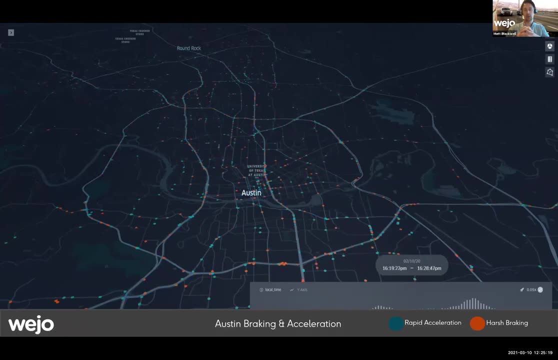 And this is all. or you know the visual that Gareth has already already Showed, But probably just to add a little bit more context around this. you know the hard braking and rapid acceleration events that we see from the vehicles. these aren't simply hard. you know tapping of the brake or tapping of the gas. 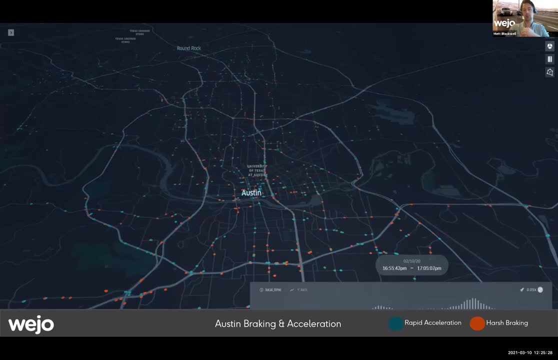 These are real kind of hard coded thresholds in the vehicle. So for context, this is either plus or minus 2.67 meters per second squared If you want to get really technical with it. but that event is actually triggered within the vehicle and we've actually done a lot of work with the likes of 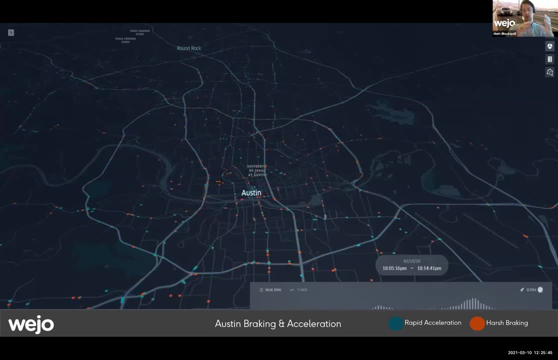 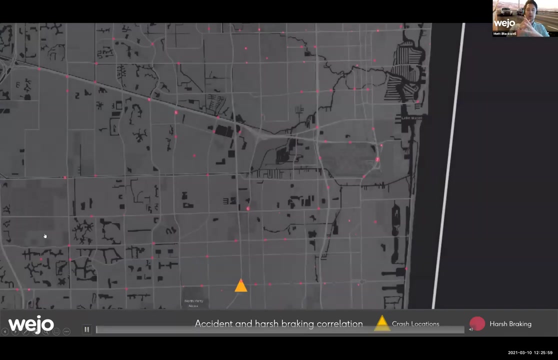 Um, Purdue university, where they've actually seen correlation of about 147 hard braking events is conducive to their having been an accident or going to be an accident. I don't encourage anybody to to look at those studies that have been done. Now you know again, when we start to look at um- the safety element, we are very, very passionate as a business around that mantra of data for good. 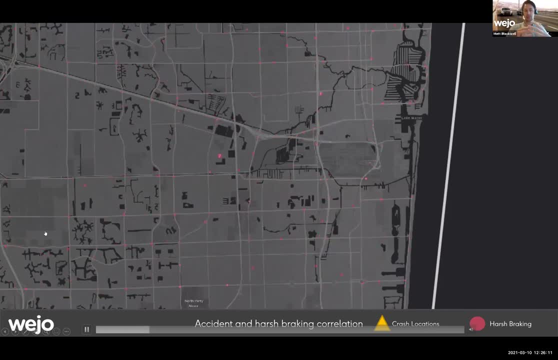 So actually using data for influencing any kind of safety models Or being, you know, playing even a small part in reducing the amount of fatalities is important to us. So what we've done here is we've actually overlaid um existing crash data. 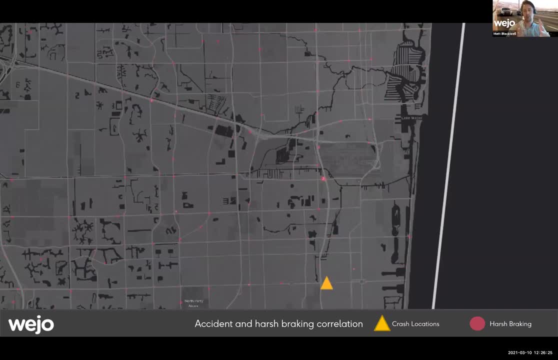 I think this was was from RITUS, with the hard braking events. So the red circles that you're seeing are the number of hard braking events over a 24 hour period, And then the triangles are the number of crashes that have actually occurred. 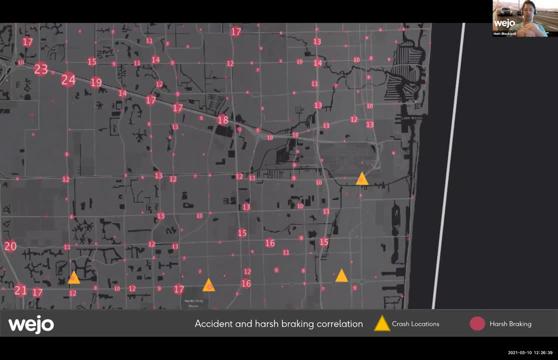 But typically, again, when you start to look at crash data- because that's collected by the attending officer, it's not always Particularly accurate in terms of you know the time period that it when it when it when the incident was supposed to have occurred. that can be, you know, actually the crash occurred half a mile down the road. 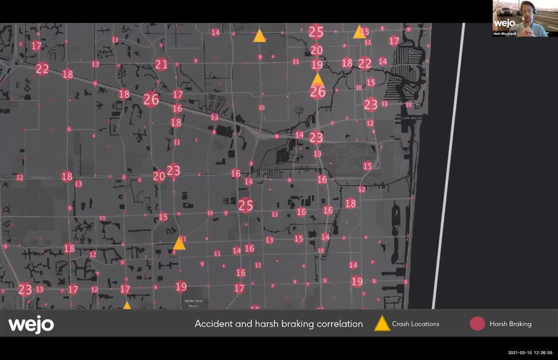 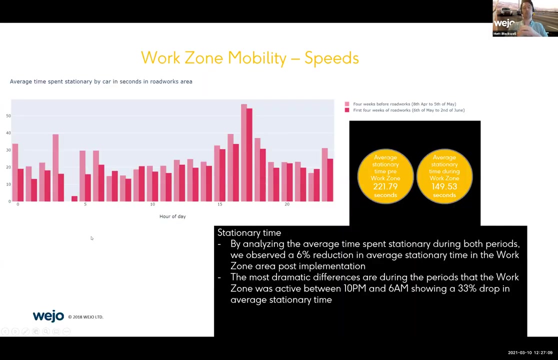 But because these data points that we're collecting are accurate down to that- that six decimal place accuracy- you can probably start to see actually there is real concentrations of hard braking events at specific intersections. And then this is just a couple of examples of work that we've done around work zone mobility. 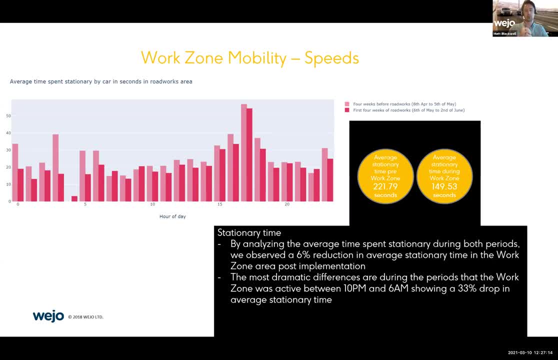 So this, This was um a particularly small work zone in in the Florida area where we were actually able to use connected vehicle data to look at. okay, what did the general speeds look like And what did the the average time spent stationary look like prior to the roadworks taking place, versus that first four weeks? 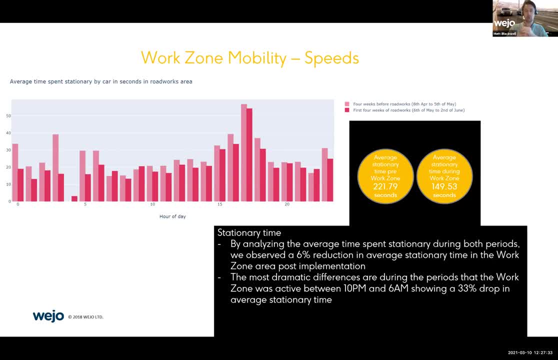 Now, actually, contrary to popular belief, we saw a huge drop in the amount of average stationary time seen by vehicles when the roadworks were actually in place, And that's extremely important for a lot of the, And that's extremely important for a lot of the. 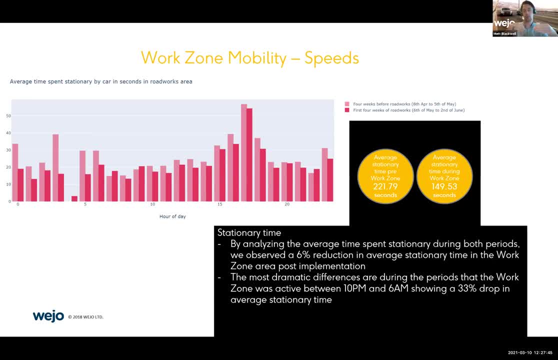 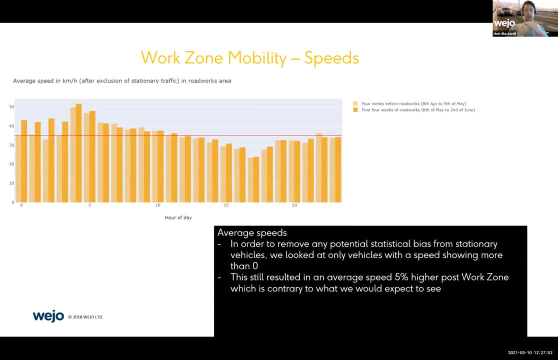 Civil engineering firms who have to validate the work that they're doing, to make sure, actually, that it's been properly planned out And you know, if we move on to the onto the next slide. again, this is looking at the average speed in kilometers. 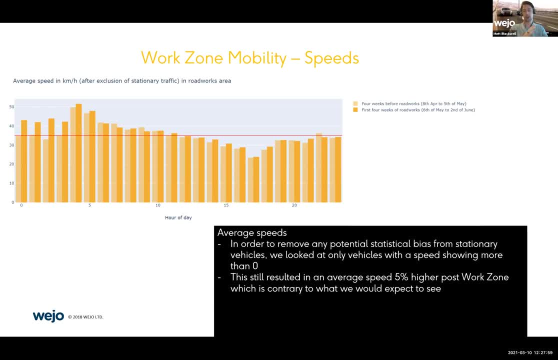 So we're looking. you know the average speed in kilometers before any roadworks took place is actually a lot, you know, in some cases quite a bit slower When we start to look at the early hours of the morning. Now, there's obviously various reasons for that. 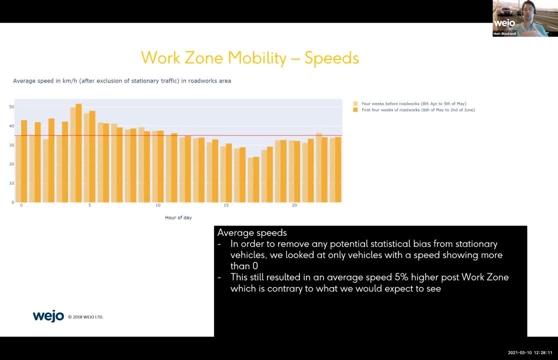 People potentially are looking to avoid that particular road Could be Reduced traffic. But again, when you start to look at the general management of that work zone, this is not reliant on any roadside units or any aftermarket devices. This is actually speeds that are being generated by the vehicles themselves. 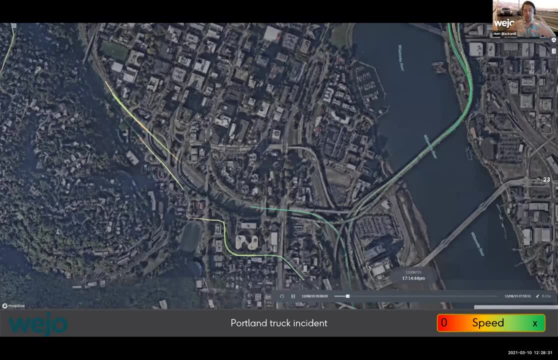 And this- I think this is the kind of final example- We you know, one thing we are very, very open about is the fact that we can actually generate this data in near real time. So Clarifying near real time, that is, from the vehicle through the platform and to the end user in under 60 seconds, is our official SLA. 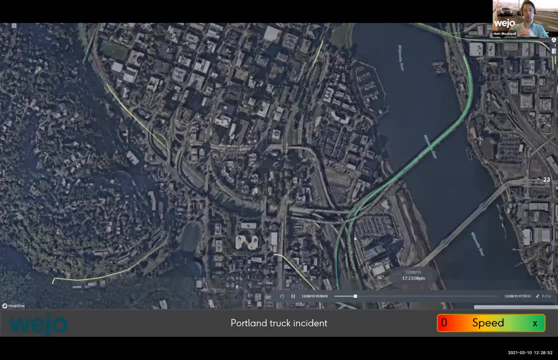 But this is an example of an actual incident in Portland. Now what you'll hopefully see in the kind of middle of the screen is fairly free flow in traffic from east to west. but you'll start to see now the journeys quickly slow down and actually start to stop in some cases. 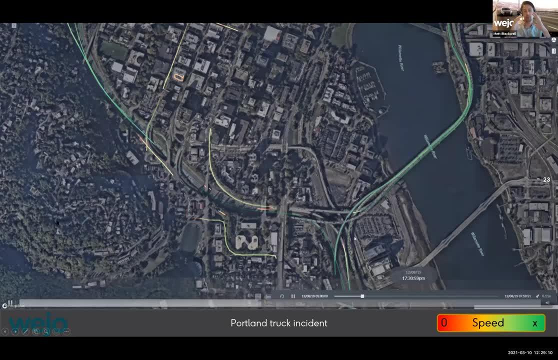 Now this was actually a major upturned Truck which Caused mayhem and for hours and hours we were actually starting to see vehicles backing up off the actual freeway, the interstate, onto, on and off ramps. And that's a real problem, for when you start to look at secondary crashes, you know high speed collisions, but we have the ability to actually be able to visualize that congestion and and speeds in in near real time. 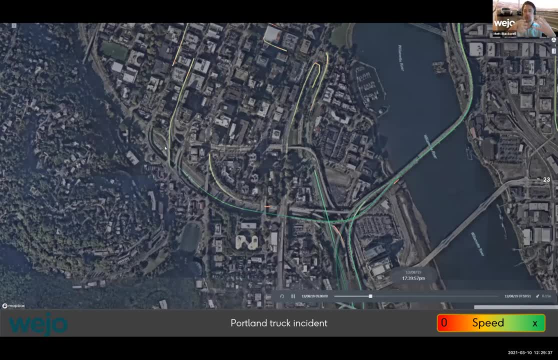 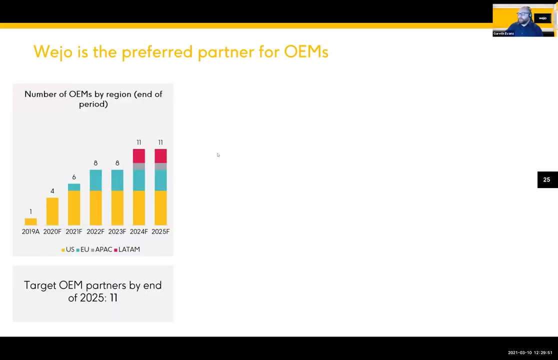 So when you start to look at the applications around traffic management centers, we're seeing real kind of benefits and uptake there bypass 못. So when we start to look ahead, both in the in the shorter term and longer term of of where we Joe is going and the application of of connected vehicle data, and have our support in 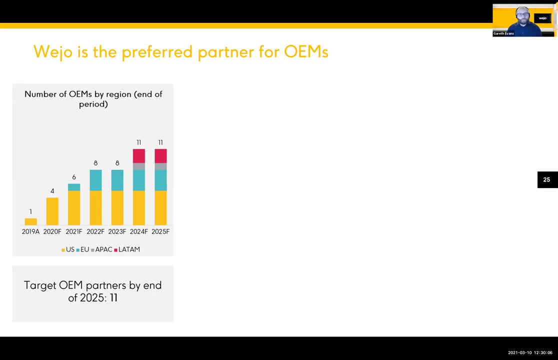 i'm gonna just touch on on how we Joe is operating this space and our future Objections on what we're looking to do. then i'll pass over to uh, pass over to matt. so in terms of the number of oems, in terms of the car, 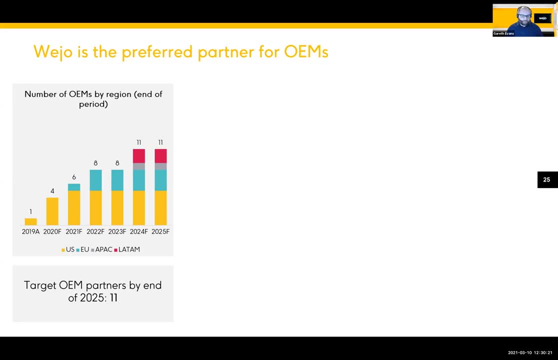 manufacturers by region. um, you know we have very- um, i'd say, lofty goals in terms of where we're looking to to achieve this. what's really interesting is that you know, over the course of the last several years, the relationships that we've we've had with the global car manufacturers. 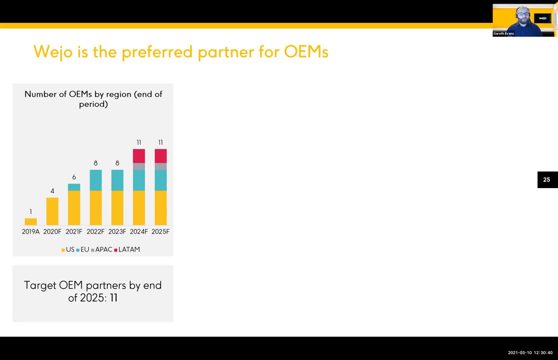 is. it hasn't been one way, it has not been ouija reaching out. it's very much a collaborative effort and we are seen as that preferred partner for those oems and there's it's a very challenging landscape as each oems is in a different phase of their connected vehicle journey and what we 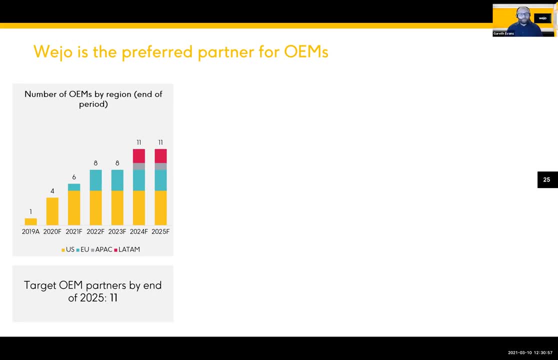 do offers. uh, the support for these guys um is is we have two sides of what we do. we do very much how our data can help and facilitate the people like yourself, but we very much support the oems in their connection to the car manufacturers. so we're very much looking at that and we're looking at 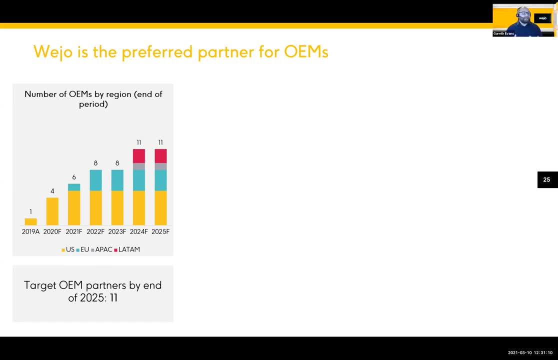 that and we're very much looking at that, and we're looking at that and we're looking at vehicle journey and how to obtain the, the necessary and the and the vital information from these vehicles which people like yourself are looking for. and so you know, we're already on. 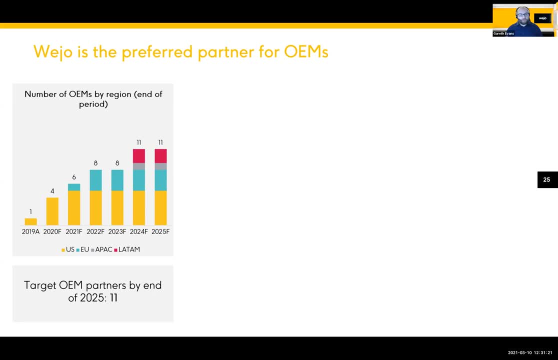 target and actually we're exceeding expectations in terms of our onboarding process for for new oems, from both the us perspective, but then also from a global perspective as well. um, and with that becomes even an even greater level of connected vehicles that we're seeing on our platform. ultimately, every. 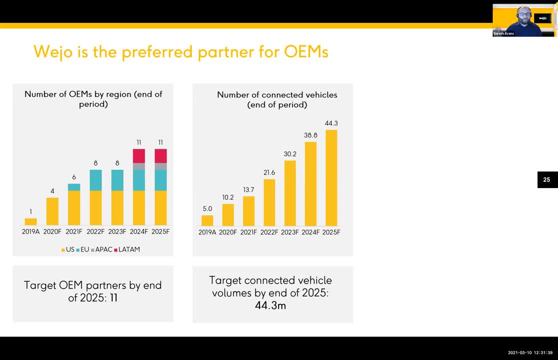 single vehicle that we're seeing on our platform. ultimately, every single vehicle that we're seeing on our platform. ultimately, every single day, our, our numbers will increase as new vehicles leave the factory floor, they're purchased and the older models of vehicles start to leave the roadways. but that happens with the oems that we've 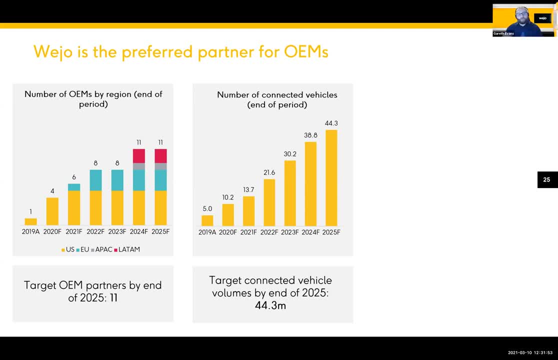 got, but then with the additional oems that we're bringing on board as well, this is where we see that really progressive jump in the number of connected vehicles that we have on our platform as well, and then what's really exciting is the, is the, the level of detail and the and the various 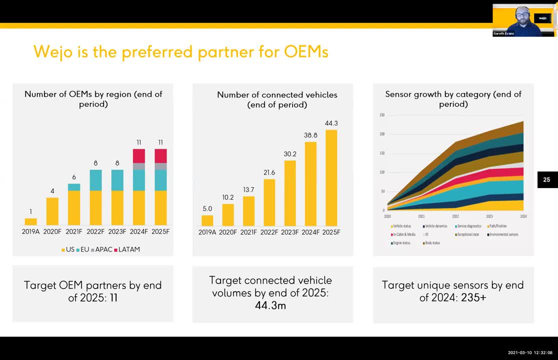 and the various different sensors and the information that we're going to be able to, we're going to be able to obtain from these connected vehicles. so, yeah, we are. we're very much looking at the realm. as i mentioned, we work across numerous new use cases, so, whether that be safety, 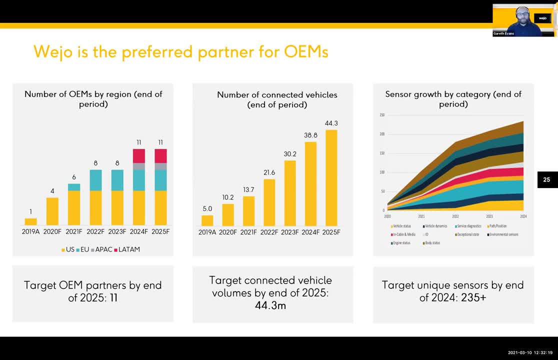 and if we can start to take suspension information from the vehicles and we can start to take engine diagnostics, well then, all the way to in-cabin as well. so the incoming media really starting to understand and how people can facilitate uh, v2v and vita um b2x, um opportunities in those. 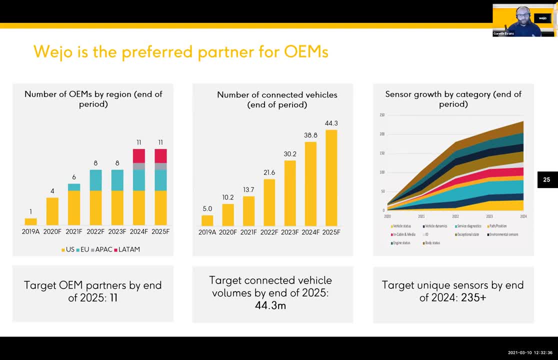 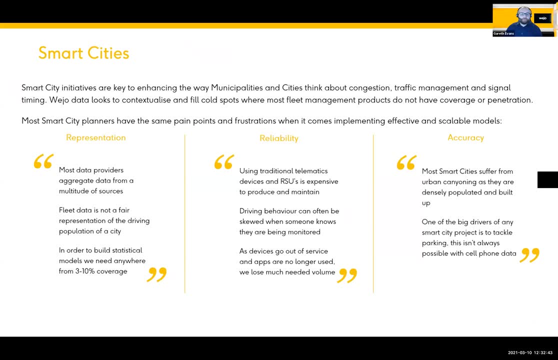 vehicles. so these are all conversations that we have with people like yourself, but really, but very much internally, with the OEMs as well. So, yeah, I think, when we kind of start to move on to smart cities, I think it's fair to say that the term smart cities is. 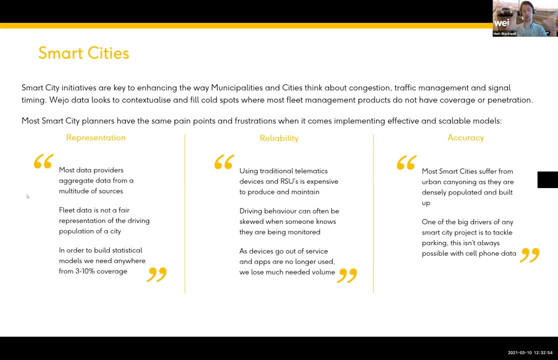 it's a very wide term. when you know, when you speak, we speak to some municipalities, some agencies, down to private companies. everybody is developing, you know, a smart city solution. Now, a lot of the feedback that we have around smart city initiatives- 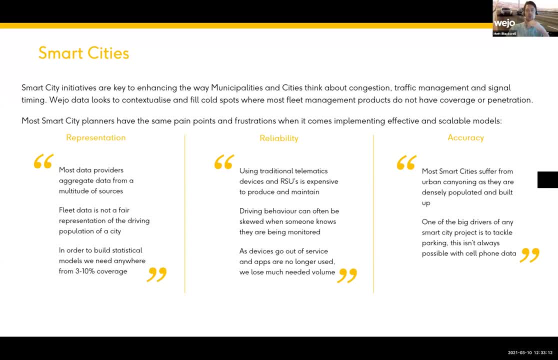 tends to come into kind of three buckets, if you like, which is around the kind of representation, the reliability and the accuracy of the data that's relied on for a lot of these smart city initiatives. So I'm not going to go through all of them, but you know. 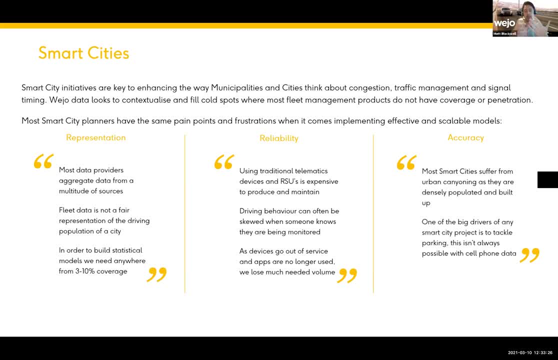 there's a lot of these smart city initiatives that are reliant on fleet data. Now, the problem you have with fleet data is it typically will come from a lot of larger heavy goods vehicles which typically don't- they don't drive in inner city areas. 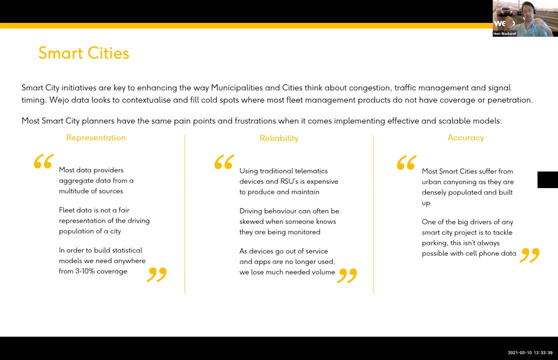 They will take. they will, you know, make their journeys along the main kind of interstates for freeways and arterial roads, And also there's a big question around statistical significance. So you know, there are aggregators out there that will aggregate multiple fleet data. 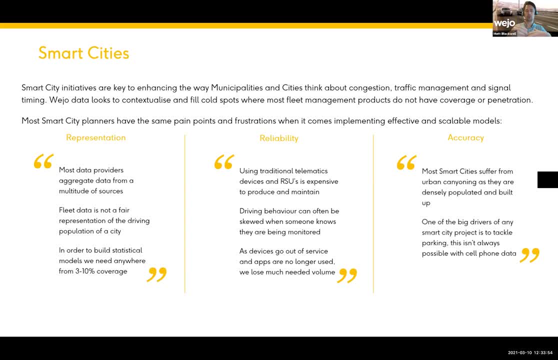 together to provide that output. But at that point you start to blur the lines on actually how reliable and how accurate is the data of representing the? you know, the true driving population. The other piece as well on this is actually when we start to look at driving behavior, you know. 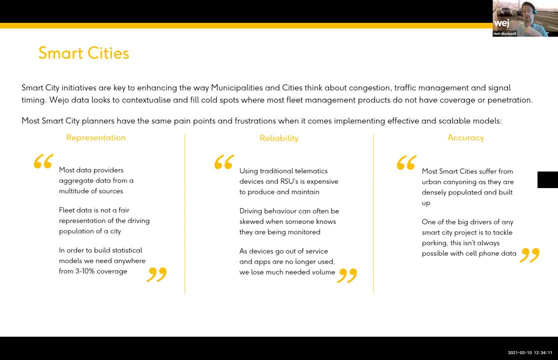 again you start to look at that fleet behavior. It's A to B, A to B, occasionally A to C, Because 95, 96% of the vehicles that we have within our fleet are privately owned vehicles. That is actually a benefit for us because it typifies that commuter. 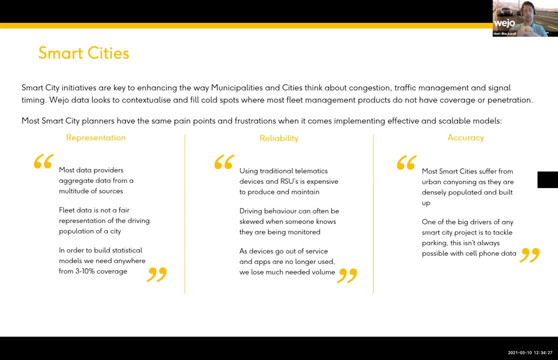 behavior And also typically with a lot of aftermarket devices like OBD2 devices and dongles. if it's anything like me, the second that person knows they're being monitored, they will change their driving behavior. We don't have that with a connected vehicle. 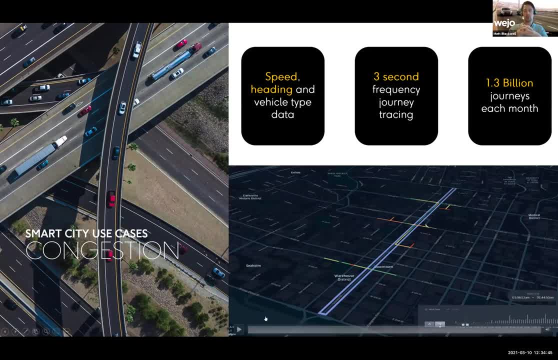 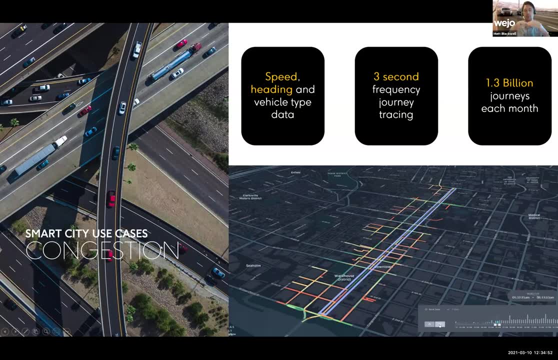 So just to touch on a couple of last kind of use cases, here, you know, we start to look at something like congestion and actually how can we influence congestion through the data? So the fact that we have the speed and the heading at a very basic level, 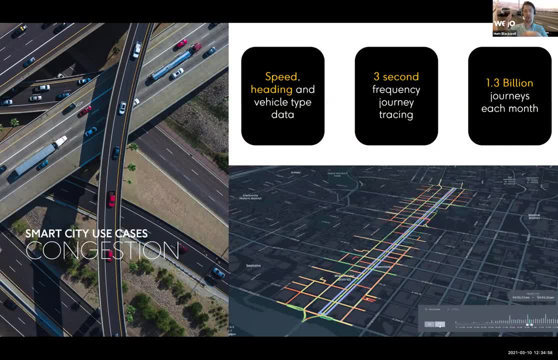 with the GPS coordinates you can actually start to look at bi-directional roads. How is that road behaving on a north to south or south to north comparison? That's a big question And the visual that you can see here. this is just a one-way street. 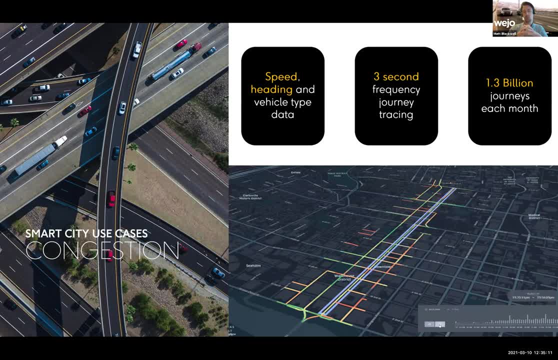 Love Arca Street in Texas, And we've actually visualized this with our traffic intelligence product. So say we were to close down that one-way street. what impact does that have on surrounding roads that join onto that street? You know so, the 1.3 billion journeys. 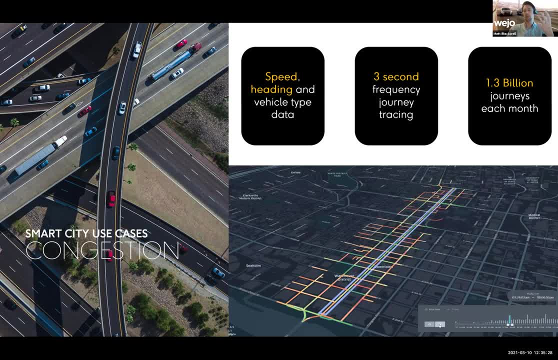 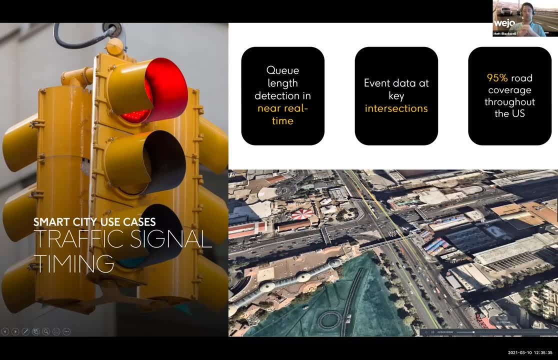 1.2 billion journeys that we look at each month. all of that feeds into these aggregate products. And then you know one kind of supposed real final use case which is certainly close to me- and it's what I've done a lot of work on- is 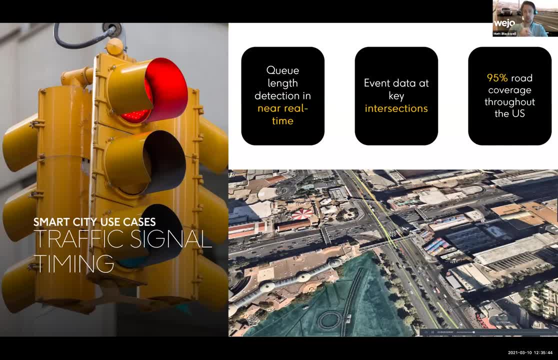 around actual traffic signal timing. So this is just a visual of the Las Vegas strip here And at this point there is nothing particularly out of the ordinary that you can see. but what I would suggest is that just to the left of the visual, that 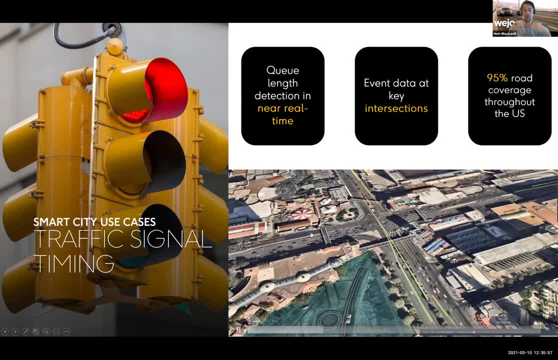 you see, you see those red dots on the road. Now that's vehicles within the Wijo fleet that are still transmitting their latitude, longitude, their speed every three seconds. So we can actually start to use the data to look at. okay. 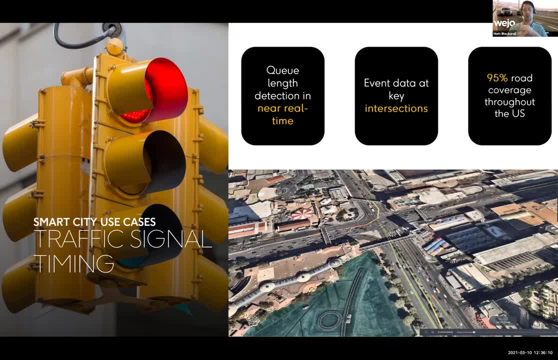 can we understand what is the at least the queue length at that particular intersection? Because the thing is we start to look at traffic signal time and it's reliant on a lot of induction loop data, So actually that those induction loops typically tend to be you know. 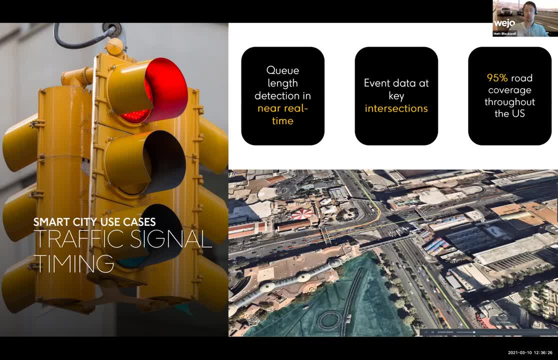 20 yards back from the lights. Actually, if we see a Wijo vehicle 200 yards back stationary in the middle of the road, potentially, yes, it's broken down, but because of the volume that we have, you know that that over 10 million vehicles. 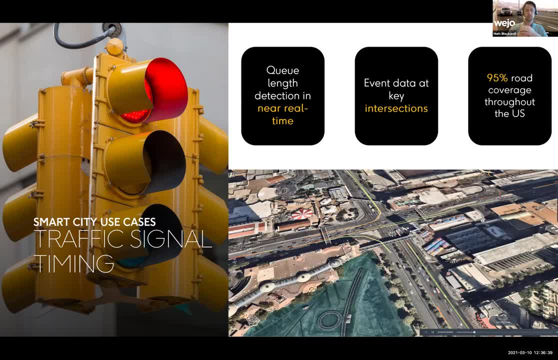 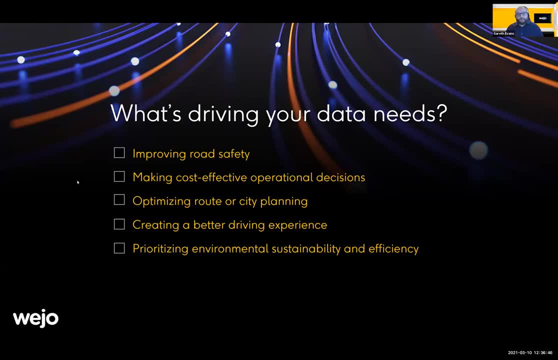 we can actually start to influence those models. So, yeah, So, on that note, guys, we've we've shared, you know, Wijo and some of the use cases that we specifically work on. We wanted to have some targeted use cases. 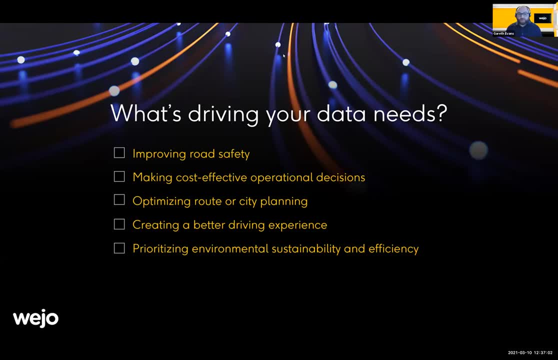 which hopefully resonate with you guys. But now is very much. you know, it's an open forum, Open opportunity whereby, if you have any questions for myself and Matt- apologies, I've not been able to look at the, the chat, as I've as I've been, as I've been going through- 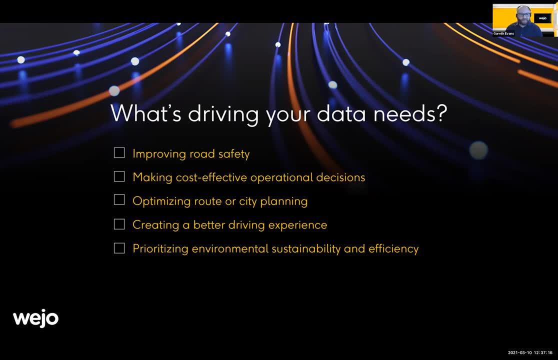 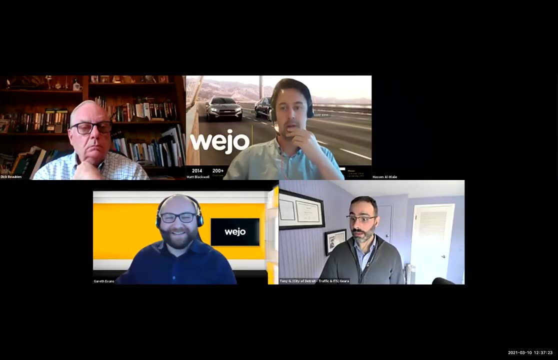 So hopefully we've got some lots of questions that we've got, you know, the rest of the session to to facilitate those 17.. Great, I'm happy. I think you're on mute, Tony. Tony, I am. 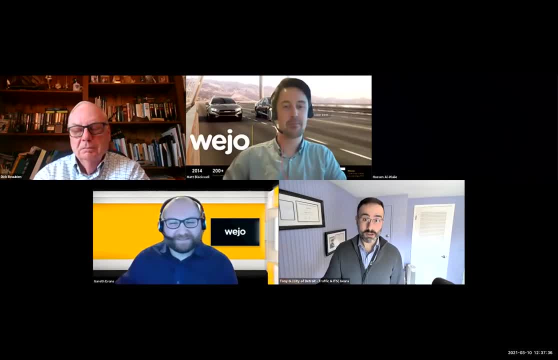 Oh yeah, So I was just saying: thank you very much. Great presentation. We do have a lot of questions, but I'll do is I'll go through them one by one And hopefully, either Garrett or Matt, you guys, can take care of them. 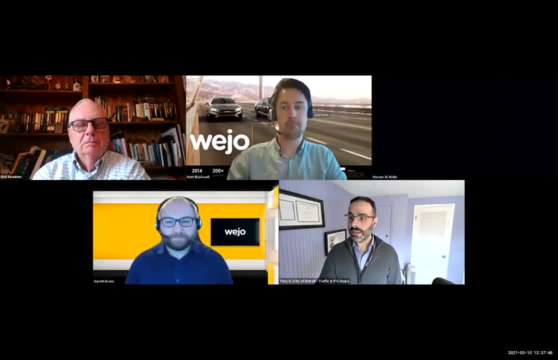 Yeah, no problem. Does that sound good to you? Yeah, absolutely All right. So let's start with the first question on here. It came from one of our city of Detroit employees. What do you mean by saying destination, as the map is showing moving target? 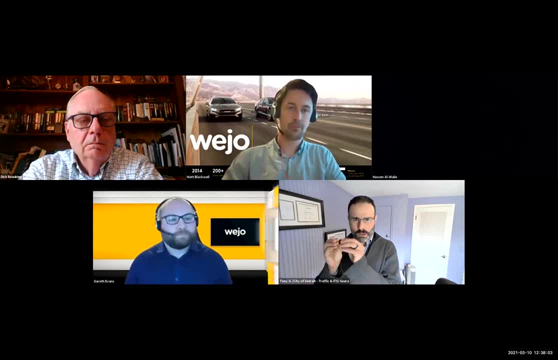 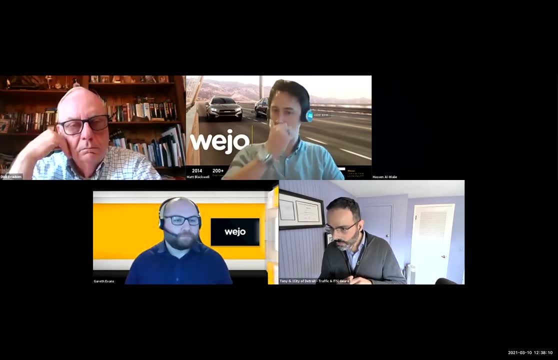 vehicles. I believe that was one of the maps where You were showing where the vehicles were going from, two with an arch going on top, and he wasn't sure about what it's. what it meant by destination? Yeah, surely So, absolutely. 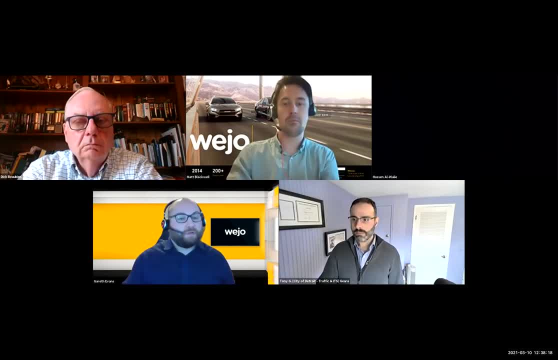 So essentially what we're able to do with the data, because we have the ignition on and an aggression off, but then we get the data points in between. in some use cases, people only want to understand where the vehicle originated from, or maybe it passed through a certain road. 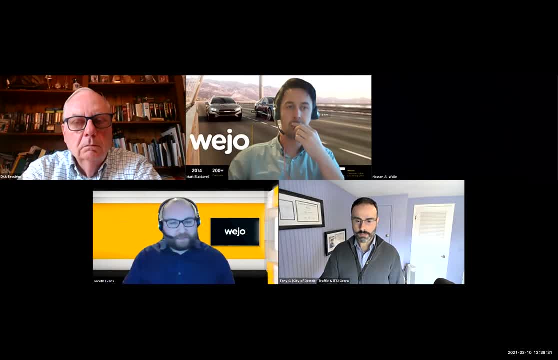 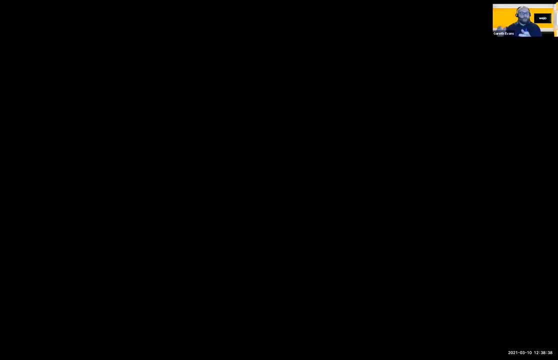 So, if we have a section, one of the use cases that we've looked at many, many times, me and Matt- is Disneyland as the example, So you know understanding where people actually originated from. So the end point was Disneyland, but where did they actually start from? 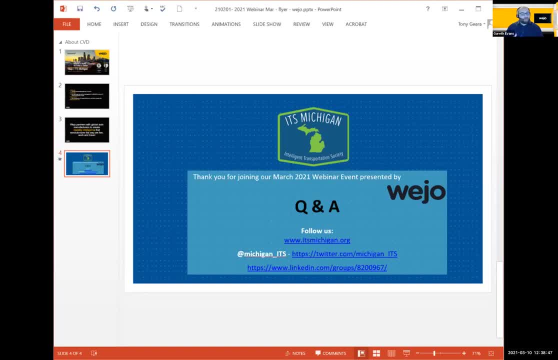 And where was that origin, The actual, the journey they took in this specific use case, for the client that we're working with, wasn't so much important. It was more a case of where, where would these people come from? So what we're able to do from an origin and destination perspective is, if people do not, 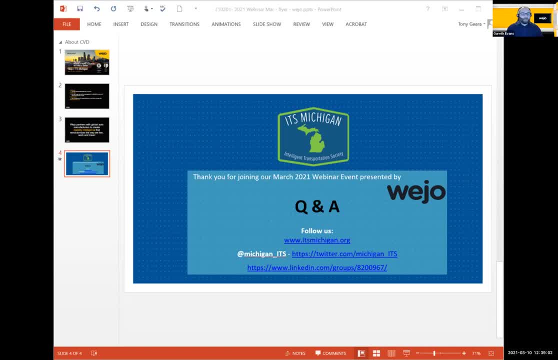 need that in between data points, we can cut those out from the Start. the journey start and the journey end. Okay, Excellent. So we have another question on that, one that came from me, and what is the format that we can obtain the outcomes of the data? 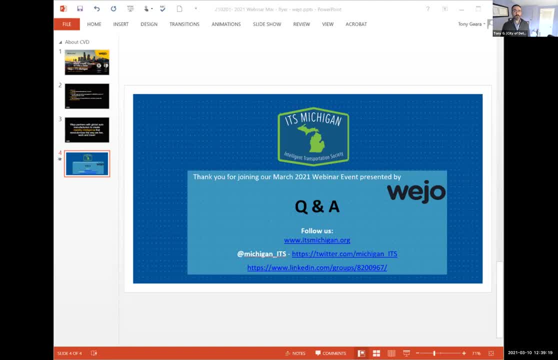 Is it just reports? Is there a Wejo platform or you know how? as a as an entity, as a private agency or as a public agency? what does this data look like? Yeah, I'll leave that one to you, Matt. 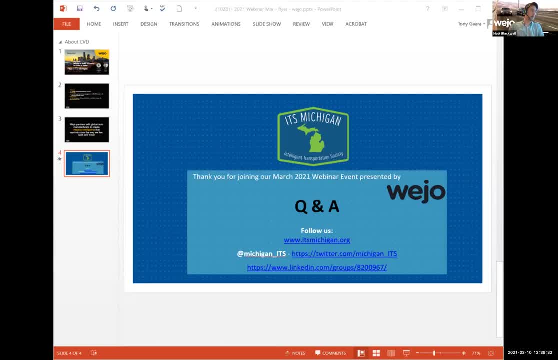 Sure, No problem. Yeah, So there is a variety of outputs We can. we can look at the providing the data in now for big data agencies as an example. they have the infrastructure to support what we'll term as as kind of raw source. 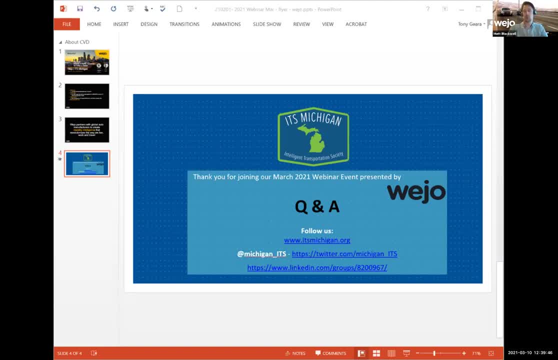 data Now, without going necessarily too technical, you know that raw source data will typically be in something like a JSON format, very ingestible for you know, a lot of GIS products. Now, as we mentioned before, we also have the ability to provide the data in an aggregate. 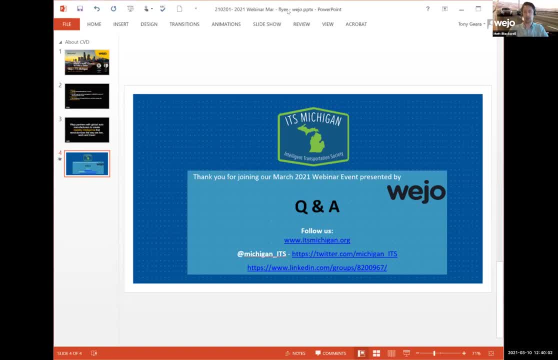 format, So aggregate being a flat CSV file that will provide you With those metrics, such as average speed, again visualized very, very easily, And a lot of the commonly held GIS tools like arc GIS. we are working on building out a front. 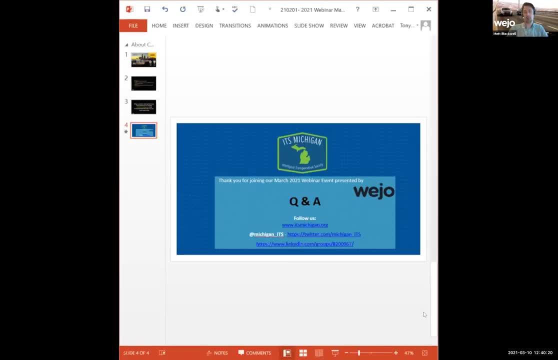 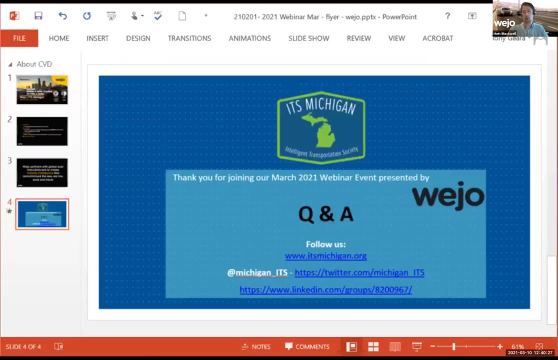 end UI as well. So that's going to be probably launched in middle of Q2, which is going to start to actually give some initial outputs and a UI that we're conscious a lot of traffic engineers will typically work with. So the initial output for that is probably going to be looking to be something like a: 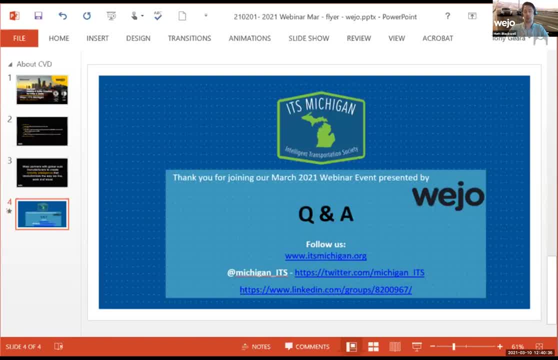 turn count tool with a view to us then plug in our intelligence products into that as well. So you know we we cater for a multitude of of infrastructures and capabilities, whether that be CSV files, the raw source data, or a UI that can be interacted with. 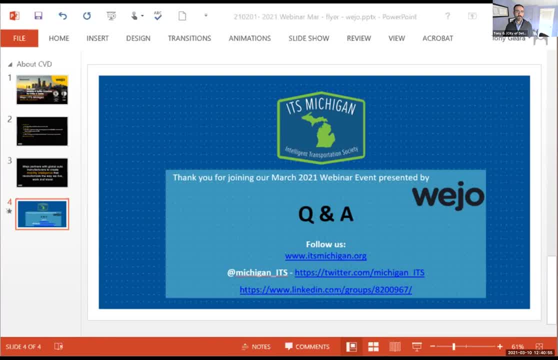 Excellent, Thank you. So the next question came from Hassan, I believe with Dan law- any plans on working with OBUs and RSUs? If so, who does the RSU fits? How does the RSU fit in which equation? So how have you guys thought about? do RSUs provide any valuable data in this case? 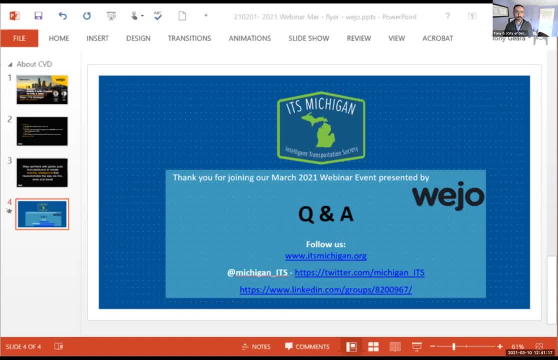 And how can they fit in to your data? Yeah, happy to say that one, Gareth. Yeah, so, absolutely So. we have spoken to a few RSU manufacturers on the basis that actually there is a real requirement. you know, with a lot of RSUs, they will capture. 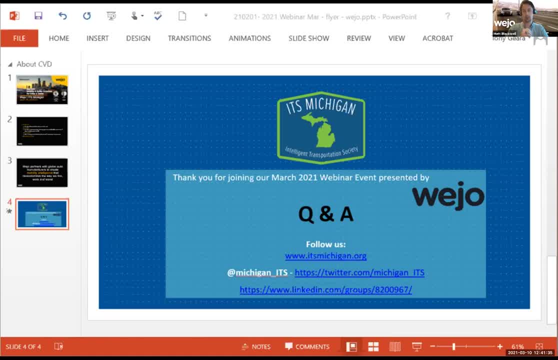 You know data, Yeah, Pointing point in time and pointing road data, which is, which is great for looking at a hundred percent of vehicles past a particular point, but with a lot of the RSU manufacturers, what they don't know is actually where are we going to put our additional roadside units? 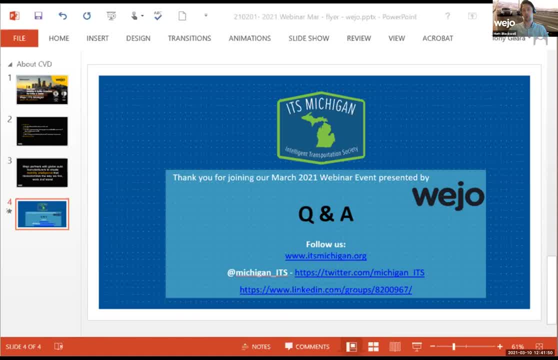 So if we're seeing a particular bottleneck through the Wijo data, you know, if we look at even a five mile corridor, whether it's an RSU on one side, on an RSU at the other. there's no visibility of what is happening in between that. 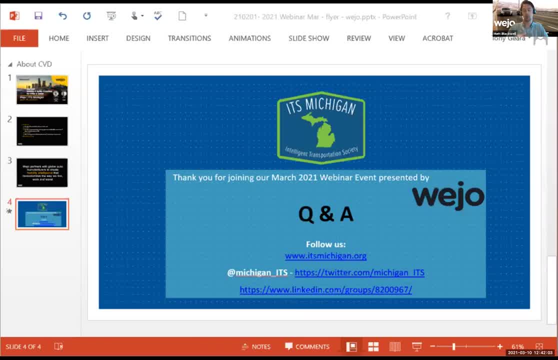 So actually we're being able to influence those models with RSUs, So we're not going to put a Rumble strip here. We might want to put a feedback sign at this particular point And also, as well, you know RSU companies. they provide us with the ability to provide ground truth into our own data as well. 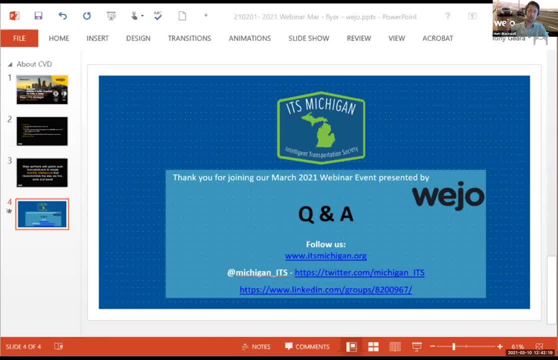 So you know, because we can actually say, okay, we know what a hundred percent of ADT is past that particular point. We do, data represents 12% or whatever that figure might be, And, if I'm not mistaken, Matt, just based on our previous discussions, we can also use our data. 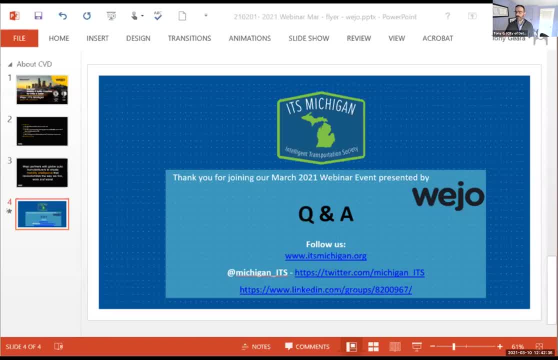 So we can use our data to be able to do something similar as well. Right In terms of, like my vision in our case, or any other counter that the state or city uses Exactly. Okay, great. So the next question is: how is the data provided by area, city, state? 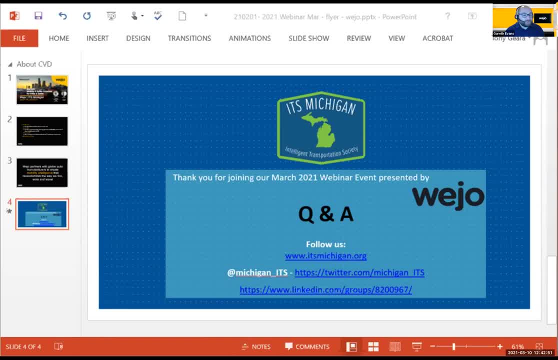 I think it's just a general quick question. Yeah, So there's no restriction in terms of how we can provide the data from a geographical perspective. All the data that we have at the moment is the entirety of the US, So in every single state. 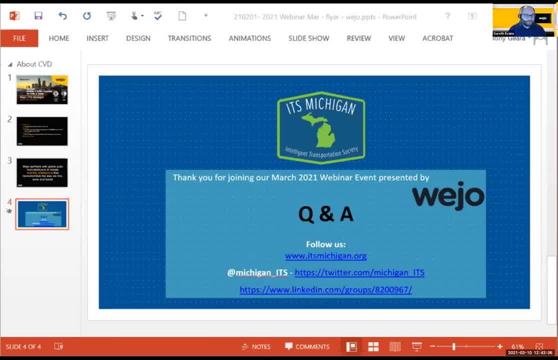 So you know, if someone wanted our raw data for the entirety of the USA, you can have that at the timescale of your choosing. If you only wanted a few intersections of road for our journey intelligence product, you could have that as well. 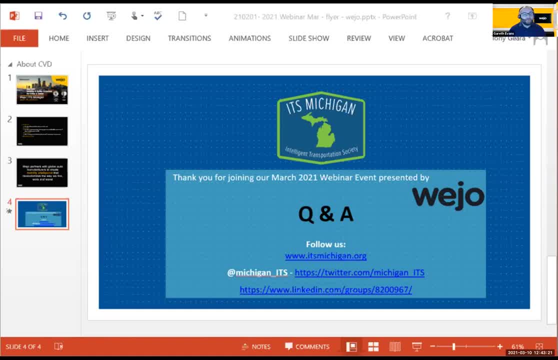 So it's absolutely dependent case by case and we can accommodate accordingly. All right, great Thank you. And so the next question is from John Abraham, from uh uh. once the data Reaches the public sphere, the public agencies, is there a concern that attorneys will be reaching out to get the info via the FOIAs? freedom of information act? 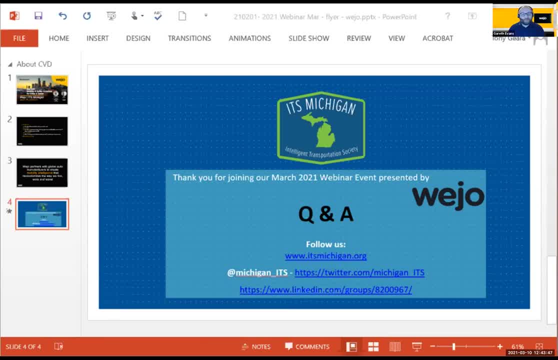 So that's, that's a great question. I wish my uh, my legal counsel's on board, but what I can say is that the uh, the data that we have, and ultimately our data, is, you know, uh, first and foremost used for good. 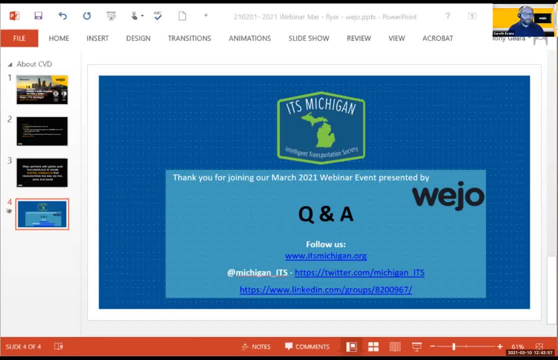 So we do have limitations of what our data can be used for and the restrictions that are in place. Um, so we we do have, You know, robust licensing agreements. um, that is agreed upon between us and our licensors, which is the OEM, and there there will be- and there are- restricted use cases where our data can be applied. 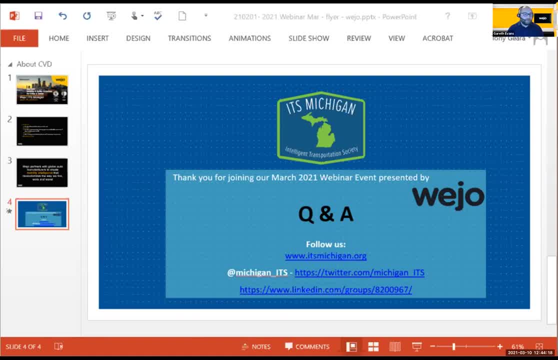 Um, so, you know, we, we work with our clients, um, you know, openly on that. but yeah, there, there is. there is, you know, let's say, gray or or areas that our data just won't, won't supply in. 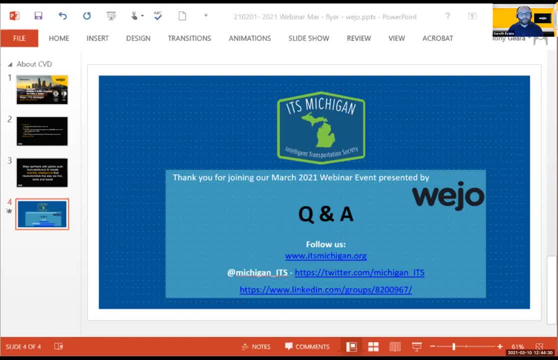 Um, any further than that, I think I'd need my legal counsel, unless, Matt, you can, uh, um, you can, jump in. No, I think the only thing I'd add onto that is: you know, as a, as a business, we are very cognizant of things like CCPA. um, you know more recently, um, you know, I think Virginia have passed more recently that their own kind of version of CCPA. 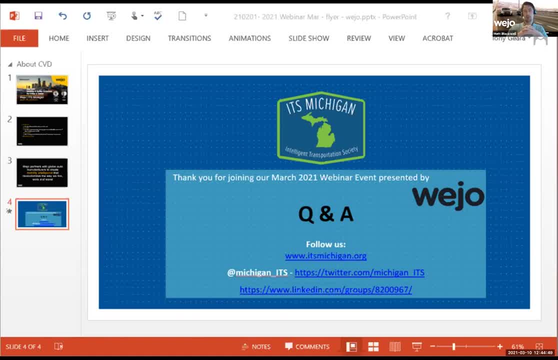 Um. so you know, all of the data that we house is it's anonymized and it's aggregated. So you know, we we don't have the ability to to reverse engineer that data, Um, even if, even if we wanted to, and as, as Gareth has mentioned, you know, we have strict um data sharing agreements in place. 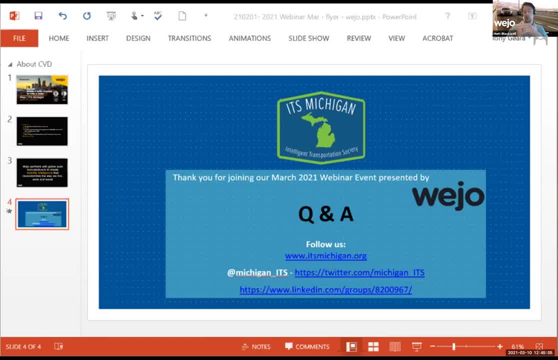 With the OEMs and also with our- with our- end clients as well, around usage of permitted usage of the data. So you guys bring up some really good topics and I maybe- uh, John, if you want to unmute yourself- it would be interesting to to understand what kind of information would they be requesting in the case of a crash. 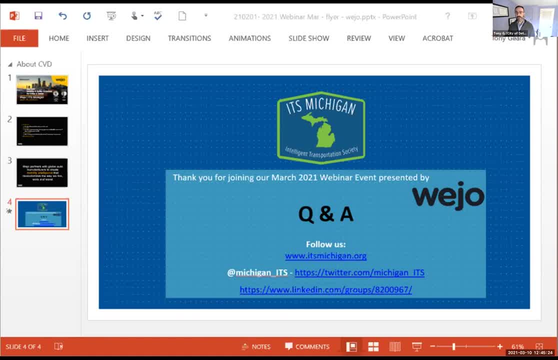 They may be asking for signal timing. They may be asking for some of that, the video that's available, but in this particular case I don't think there's anything that could be litigated or used for litigation. Uh, but if you can, 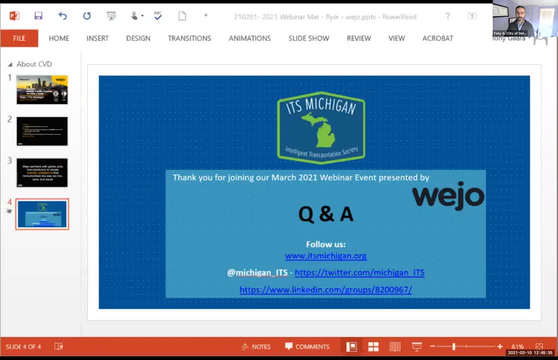 If you could shed a little bit more light on that? uh, please feel free to do so. So, uh, my question was based on your example. you talked about a truck crash and the circumstances that led to that truck crashing. uh, you know, in your example, in in Austin. 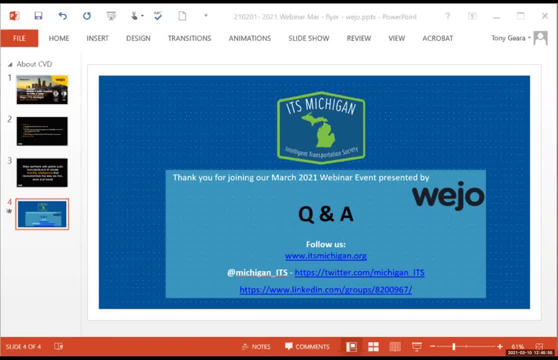 So that would be information. if that is public, then people, I mean if, if the lawyers know that, Hey, uh, there is this information that Is available, they may use it. I mean they may want it and they may first come, come up to the public agency with the with the FOIA request saying, Hey, we need that particular data, um, similar to what you presented on the trucks. 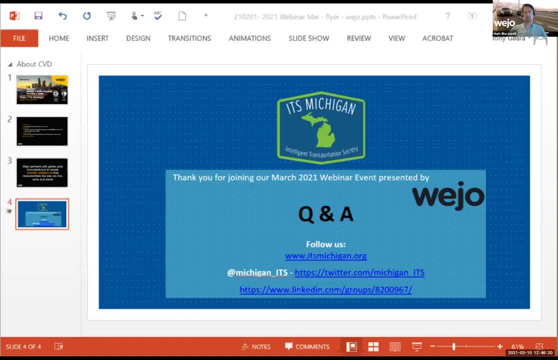 Yeah, And, and you know, FOIA is something that we do take very seriously internally. I think you know the one thing to probably notice: that particular um overturned truck. we are not categorically saying that we have the root cause to that particular incident. 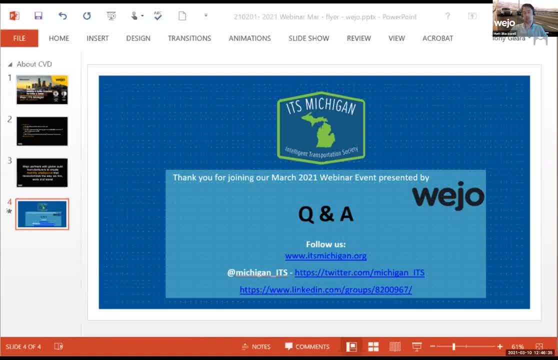 Yes, We have context around it in the, you know, in the form of of anonymized, anonymized data, Um, but yeah, I, I I take the point in terms of: you know, it's entirely possible that down the line that FOIA could come to the forefront in terms of the because of the granularity of data that we have. 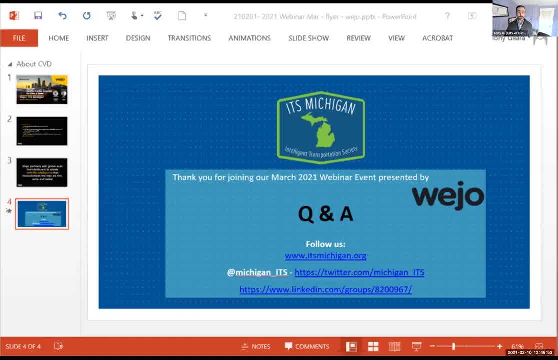 All right, So good stuff. And so, Hassan, if you'd allow me, I'm going through your question. I'll come back to you, to your second question. I'm going to go to Yasna's question. Who's asking about 10 million, 10 million vehicles that you had mentioned? 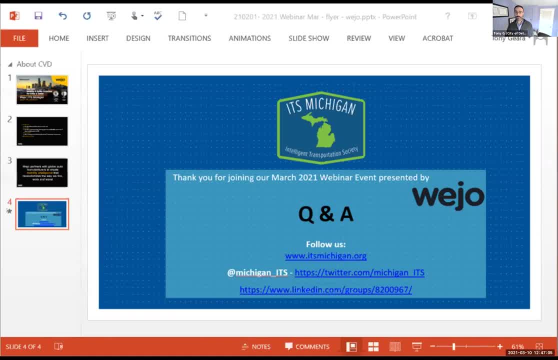 Is that worldwide? How many vehicles in Michigan? do you have those numbers? Yes, So um, in terms of all the data and all the information that I've shared, uh, everything has related purely to the USA. So we have 10.6 million vehicles in the USA, 1.6 billion journeys on a monthly basis. 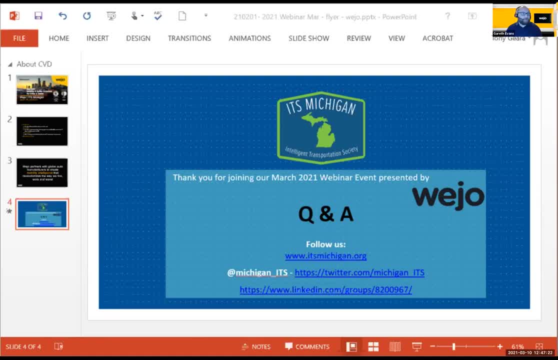 Uh, and this is all USA at the moment. So we do have, um, let's say, data outside the USA, in the building which will be, uh, live, it will be egressing, live soon, Uh, but at the moment, all online. 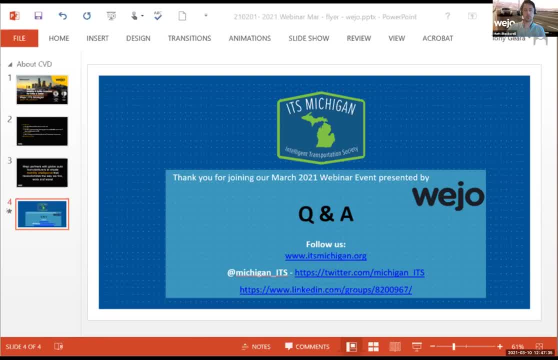 Yeah Yeah, Live data is the U? S and I can probably put a little bit of context around the the question around Michigan itself. Um, so I think we we shared some figures at the top of the presentation around. you know, we saw around 51 million journeys last month. um started within within Michigan. 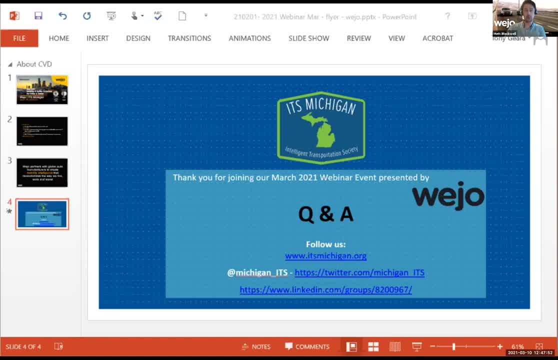 You know, if we start, if we start to look at some of the aggregate tables that we produce each month somewhere like Detroit, for example, we saw around 150,000 distinct vehicles, uh within Detroit, around 4 million journeys. 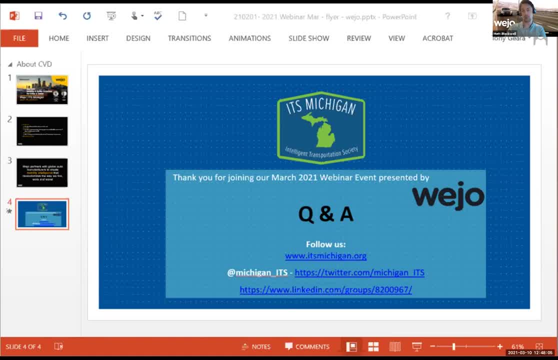 And just over a billion um data points. hopefully that kind of puts a little bit more context around it. Is that for Detroit last month, Correct? Oh, great, Great. I just want to put that slide back up there while I ask the next question. 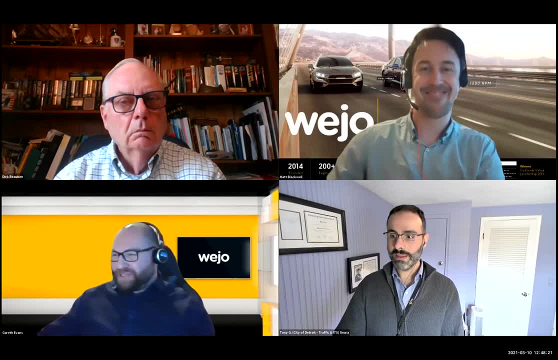 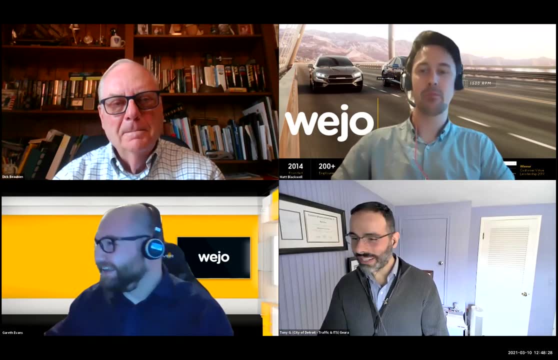 Uh, I think you I'm, I'm, I'm working, I'm working on it. Tony, I have a tendency to put you guys on the spot, but I'll ask the next question while you guys are on that up. 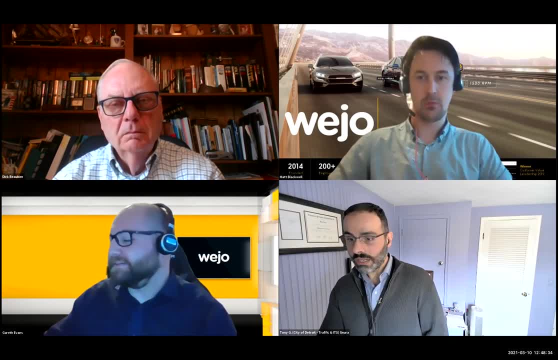 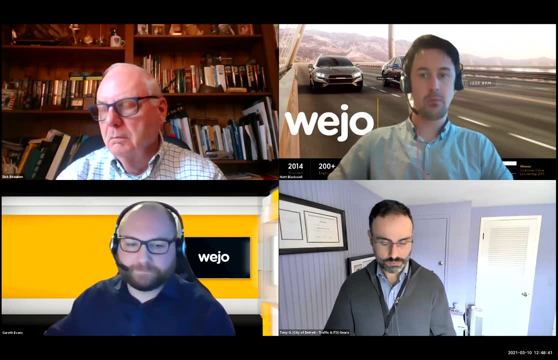 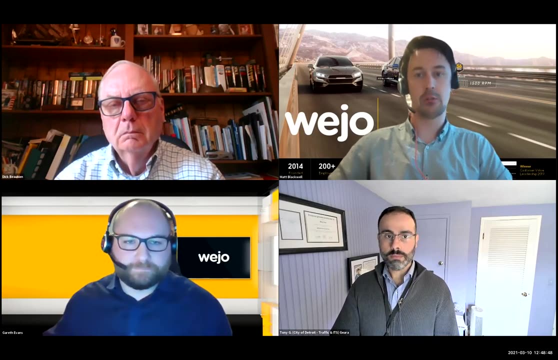 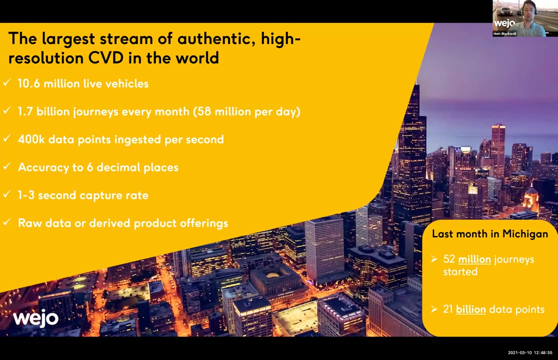 Has rego been in contact? Yeah, so I think from from memory you know we we have had conversations with both uh planning and operations um side of things at at MDOT. um, again, very conscious that you know there's a lot of data sets that are currently being used there. 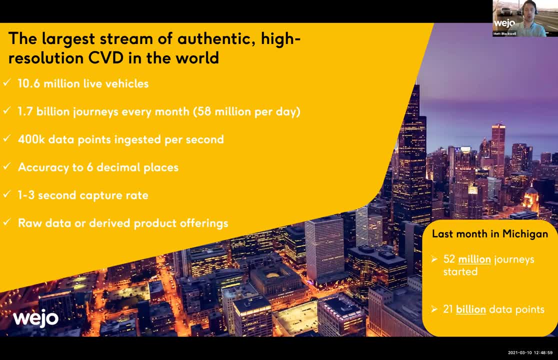 Not just, as you say, for for specific projects, but actually statewide. Um, you know, the one thing we would say Is we're always open to, to additional conversations with, with key stakeholders um, within that. So if there's anybody that you know, you think would be, you know, interested to inject into the conversation, then always welcome. 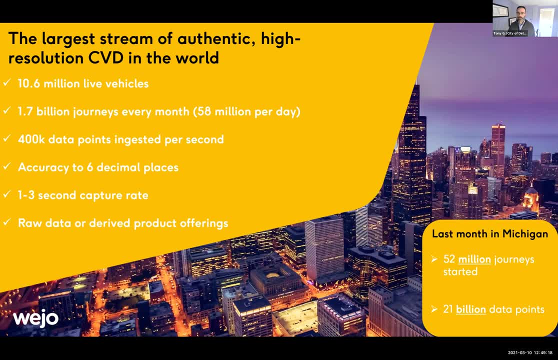 Yeah, absolutely. Um, I know from, from our end, we've had plenty of discussions with, uh, some talk MDOT and everyone keeps on saying we need, we need this, but it hasn't been that um, someone just to push the ball so it can start rolling down the hill. uh, from our perspective again, 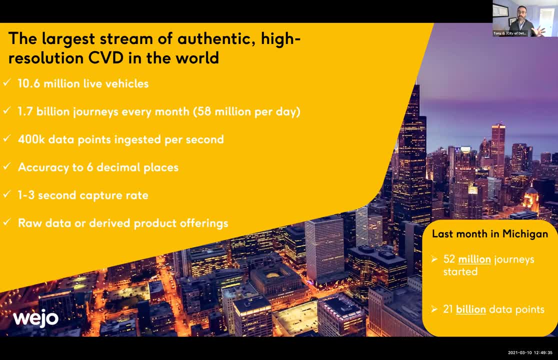 So, like you said, we're, we're, we're really excited to be able to, to share what we're doing with these, uh, these, these, uh these partnerships across the city and uh, you know, uh, we know, what's happening in between. 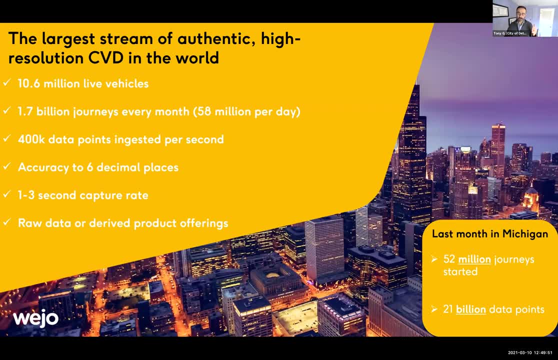 We know what's happening at those big intersections around the city, but we don't know what's happening in between, and it would be super powerful if we can come and fill in the gaps. So use those ground truth checks as our um, you know- calibrators, but then be able to kind of transmit that to other roads, because we have a lot of decision-making that goes within that. 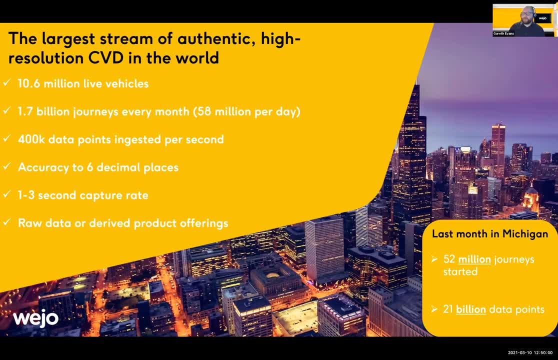 So It would be super helpful on a city level for sure. Yeah, I had to really These numbers. Yeah, US information and we can share some further details after the call. I'm happy to share that for you, Tony, to disseminate that to the audience about the latest figures that we see at WeJo. 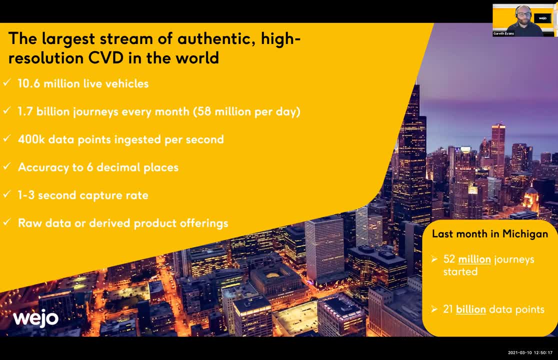 and then we can break those down specifically for your states as well. Great, and with that said, I'll go back to the rest of the questions. but would you be able to share the slides, maybe with an updated slide for Michigan, and then I can share that? 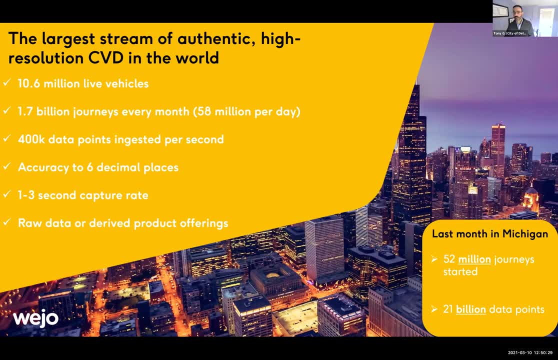 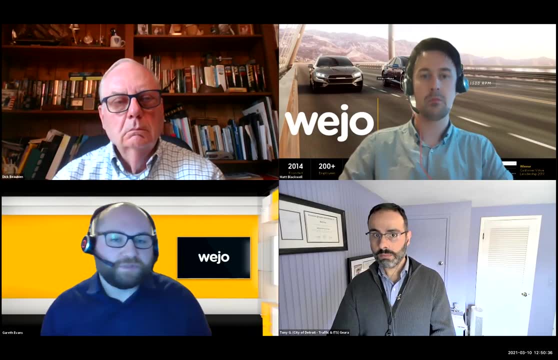 Yes, that's no problem. Okay, great, great. So were you about to say something, Garrett, earlier when I interrupted, I think it was just a really interesting point when you mentioned around planning. So a lot of the conversations that me and Matt have had, especially when we start to look at 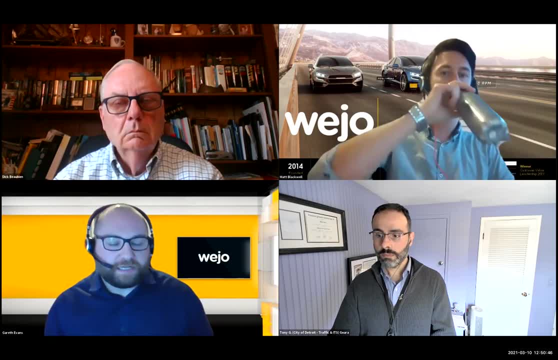 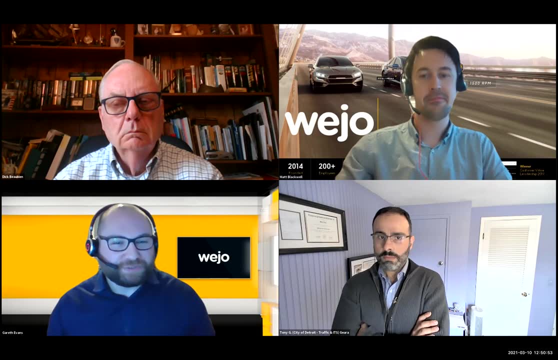 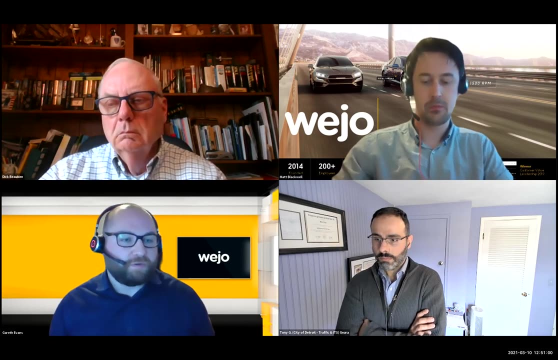 various different cities at all scales. it's really interesting how much of that planning is based on- let's politely- very old data. So there's decisions being made of either manual traffic counts on a few sections of road that were made 10 years ago. 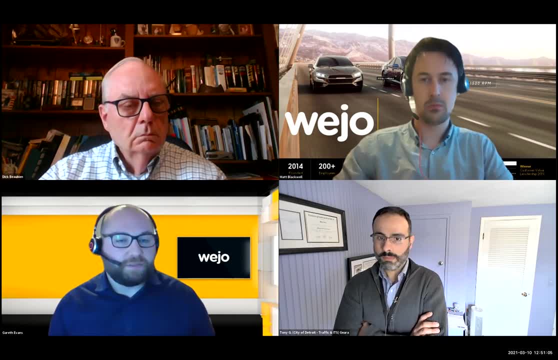 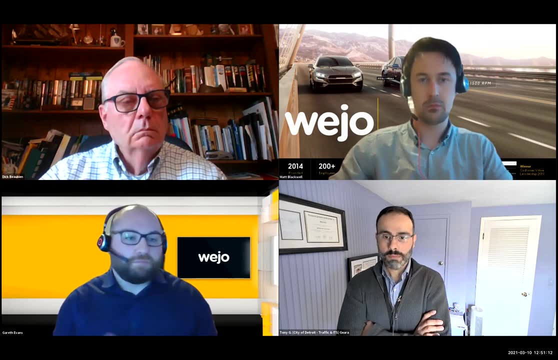 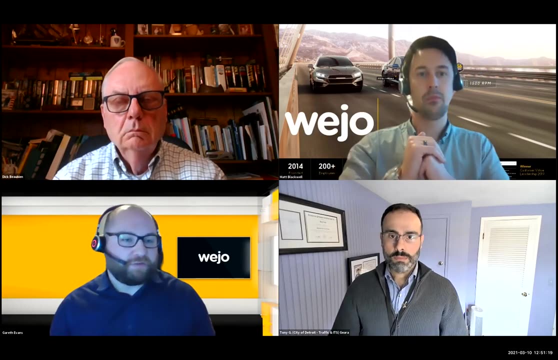 So what we've absolutely seen from our derivative products is the fact that they can get up-to-date data over the last two years essentially delivered to them as soon as they need it. I always like to use the example is if you only needed data for rush hour traffic every Monday. 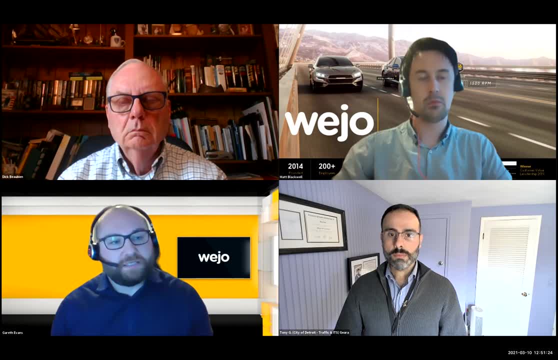 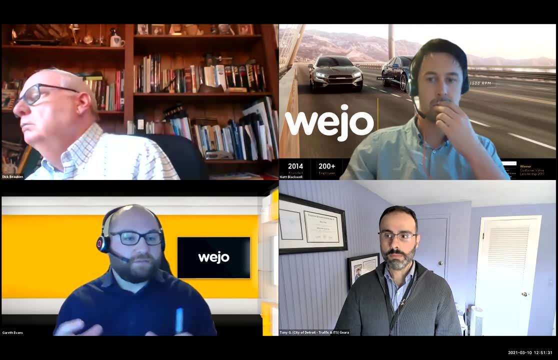 for the last two years. effectively, we could just provide you that if that's what you needed. So this is where the really good option that we have with our data is. we're not defined on scale of geography, but we're also not defined. 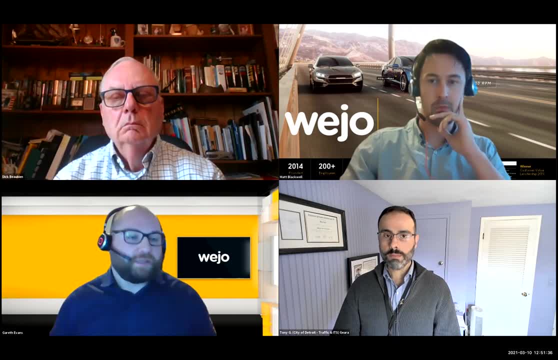 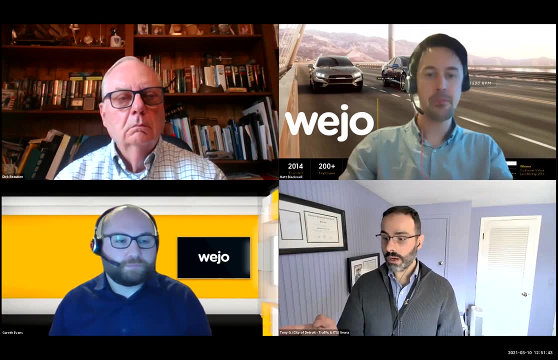 on scale of time either, So if there's only certain days, we can extract that data and supply that as well. Excellent, Thank you. I do want to also mention that, although our webinar does end at one o'clock, Garrett and Matt. 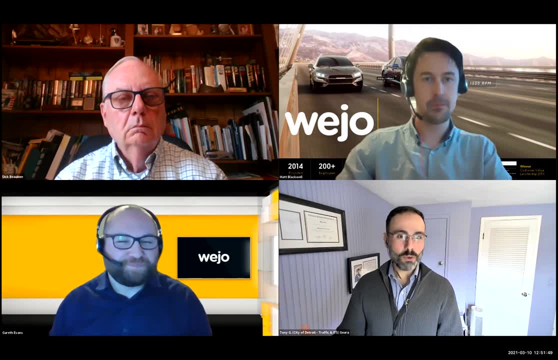 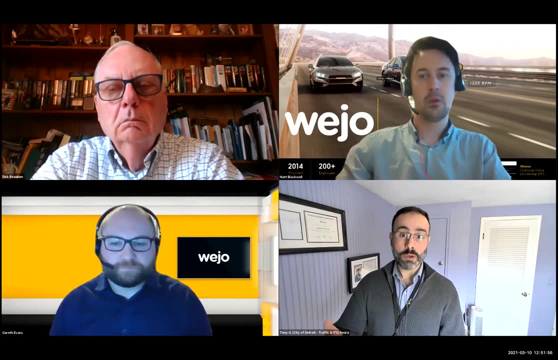 did commit to staying a little bit over if needed. So if the questions do go over, we will continue to answer them as we go along, And if you need to drop off, that's fine. The video recording will be available on YouTube in the next week or so. So going back to the questions again, some great 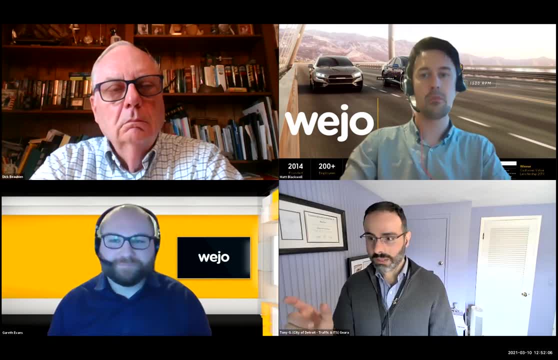 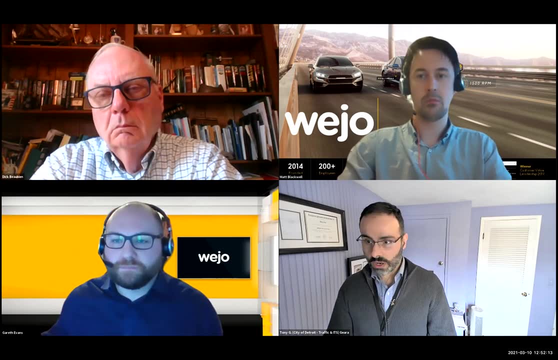 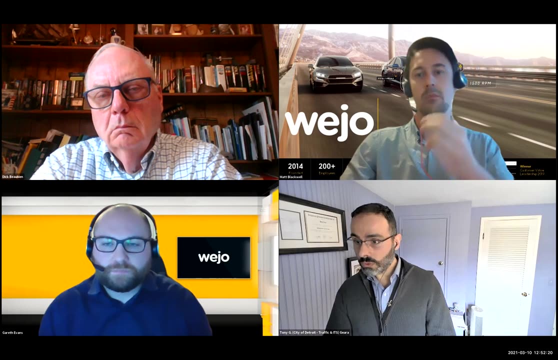 questions going on here. there's a rather long question, but I think it kind of hits on a very important item from Richard. Can you enlighten us more on the Journey Intelligence product, For example? are you able to infer trip types, example rideshare deliveries, et cetera, Or also do you? 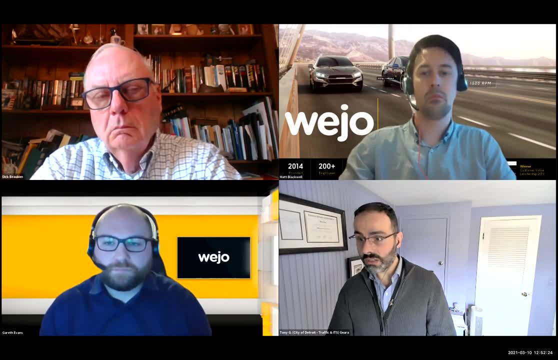 have documentation on the method and assumption for the various insights you're generating. A typical example is how you detect the data, And for those who don't have it yet, we can ask you: how do you know what data you're looking for? And then we can tell you if there're different information. 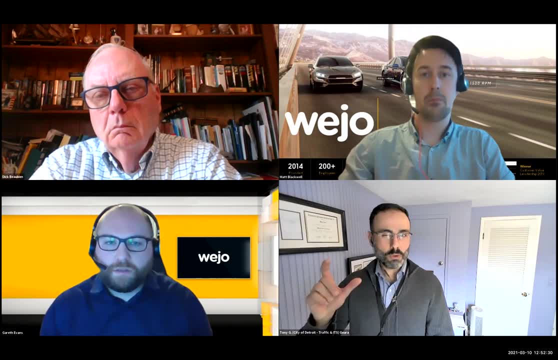 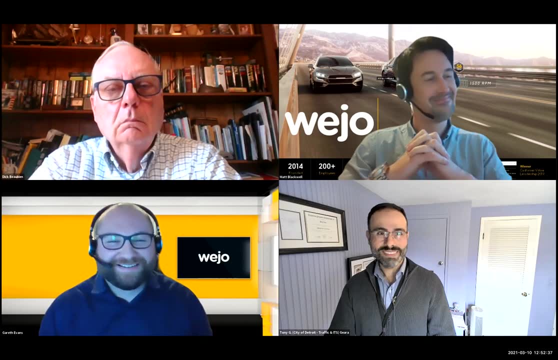 or different sources of data that you're looking for, so that you know how to get it, and then we can how you define harsh breaks. so there's two parts to it. maybe we can start with the first one about the journey intelligence product. yeah, matt, you look poised there to go. yeah, i mean interesting. 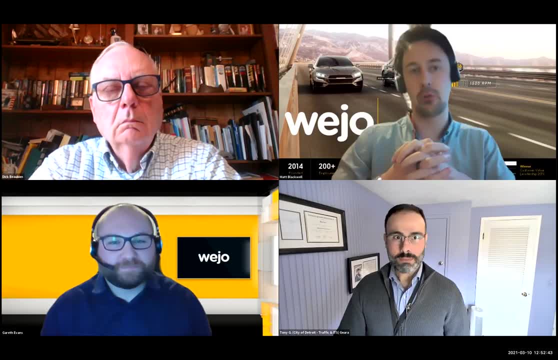 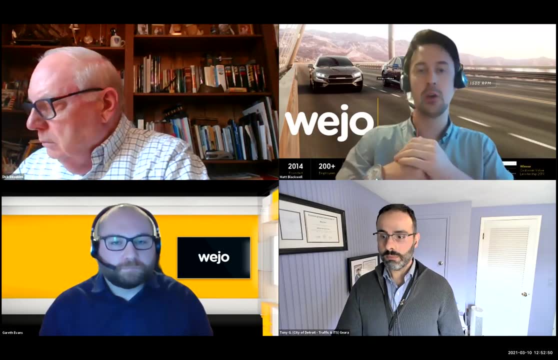 this is a conversation we've had only this morning around the journey intelligence product and how we are looking to to iterate that. so you know, being open and honest in this is that first iteration. we are not going to be looking at journey types. however, what we have been able to do is to 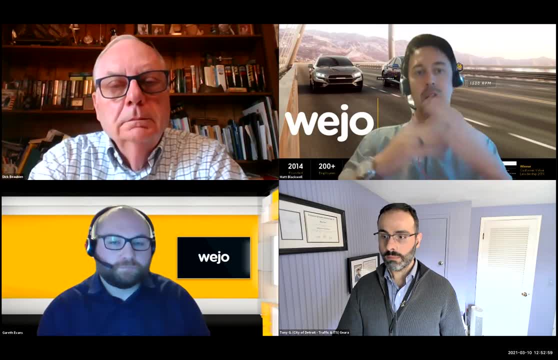 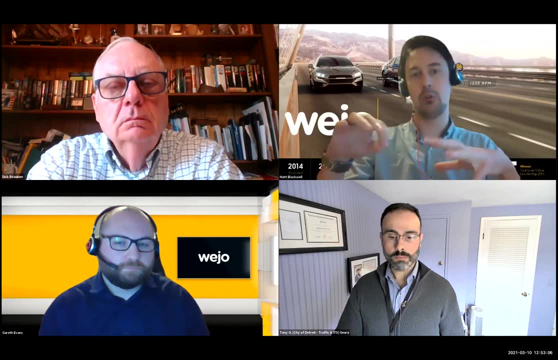 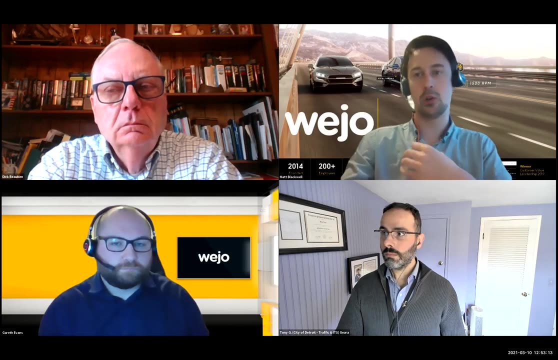 actually bucket these, these journeys, into types. so, as an example, you know it could be commute, it could be something like: and again, all this is based on actually how proximate that vehicle is to the nearest point of interest. so you know, if we look at something like a journey that ends, 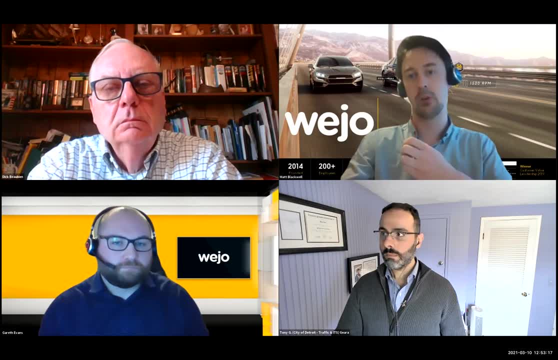 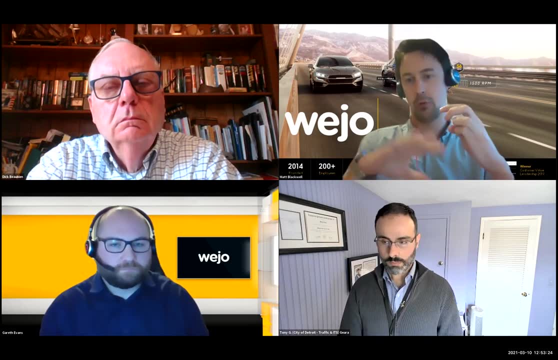 in a residential area, we can assume that that is that is a commute, so we have started to look at how we can segment the journey intelligence product into actual journey types. now, when we start to look at ride sharing deliveries, we can assume that that is a commute, so we have started to look at how we can segment the journey. 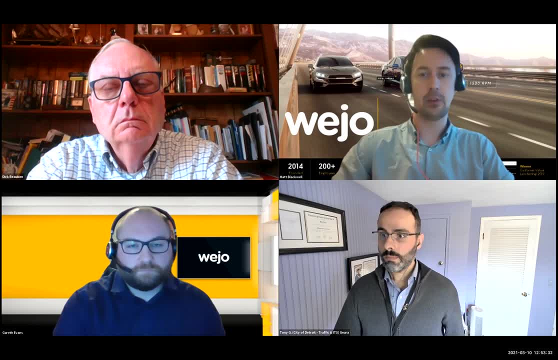 intelligence product into actual journey types now, when we start to look at ride sharing deliveries. and then the second question is around: do you have documentation on the methods and assumptions for various insights you're generating? yes, we do have product overview sheets and yes, we do have schema documents. um, i think it's probably easier rather than me kind of necessarily talking through. 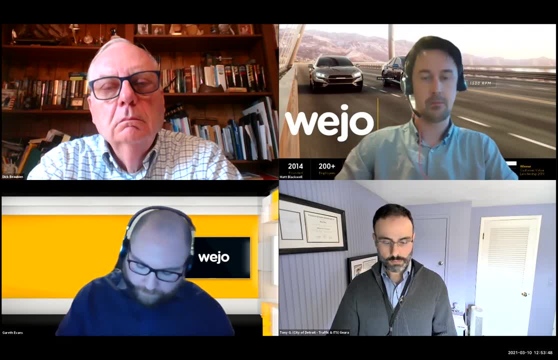 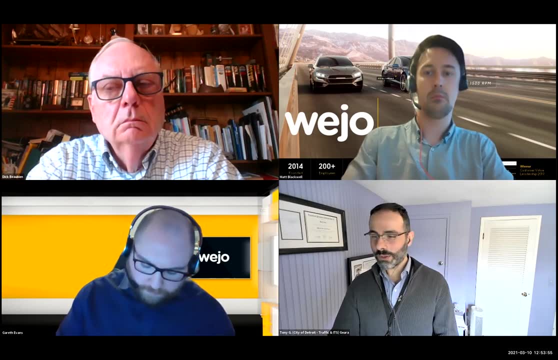 them that we we kind of share those afterwards. yeah, fair enough. um, great, so we have a question for prasad. um, one of my- uh, good buddies at work. um, i'm going to ask you a couple of questions. um, i'm going to ask you a couple of questions. um, i'm going to ask you a couple of questions. 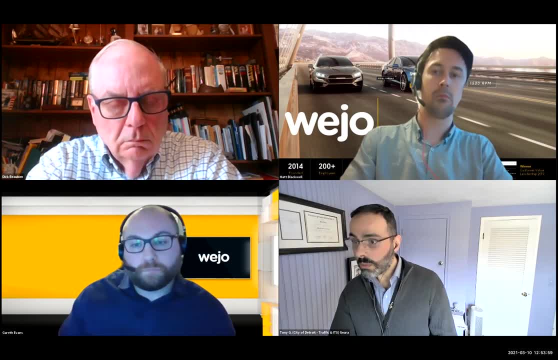 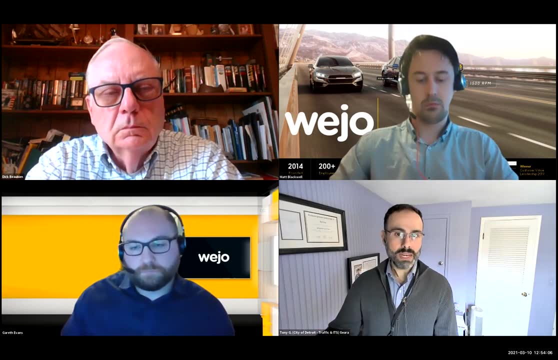 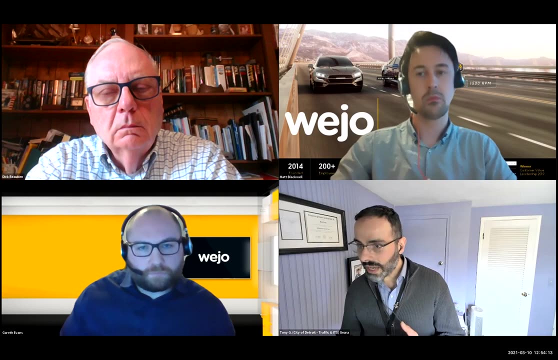 um. can you please talk about your example, or examples of how a public agency used your data and what was the outcome? and i would add to that: how did they go about obtaining it? so through a contract or through um, you know, through a project, etc. so the question again is: how did? how did a? 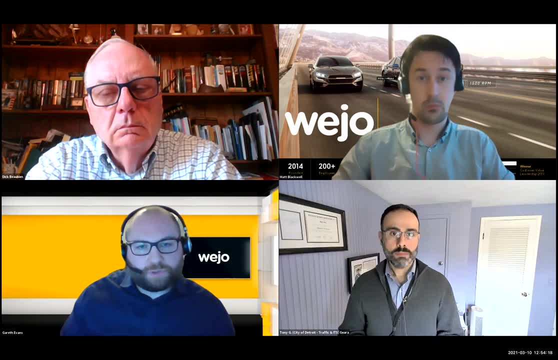 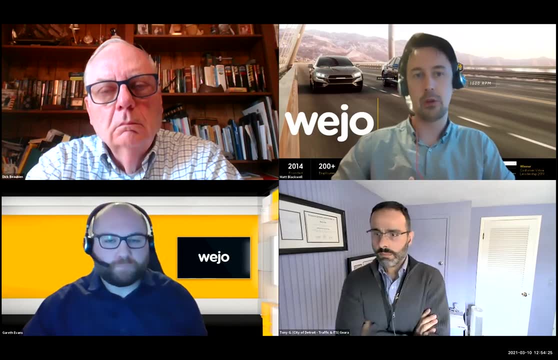 public agency use your data in a practical sense? yeah, do you want to start with the first part and i'll go with the second half? by all means? yeah, so you know, without necessarily sort of naming any names around the, around the agency, i'm going to start with the first part and i'll go with the. 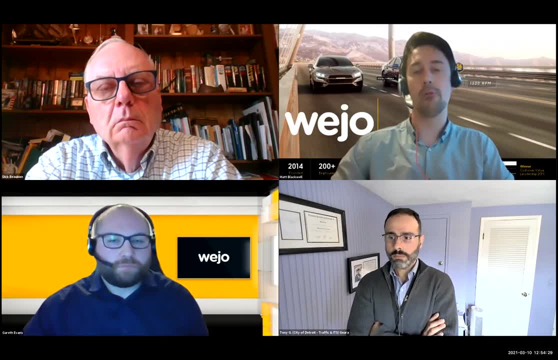 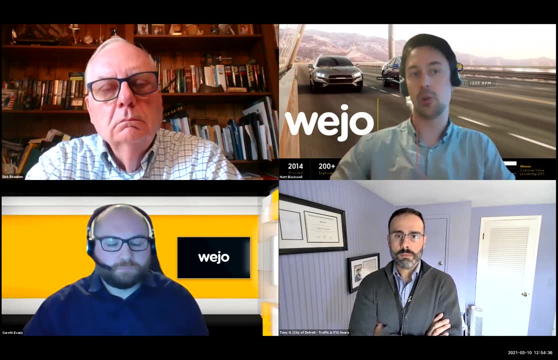 second half, by all means. yeah, so you know, without necessarily sort of naming any names around the themselves, you know, one thing we do, we are very well versed in, is actually working through agencies by proxy. so when i say by proxy, i mean a lot of the major civil engineering firms, for 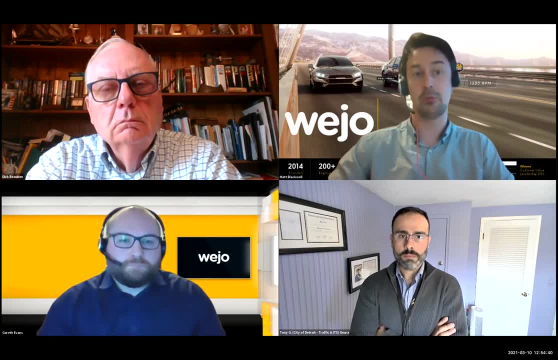 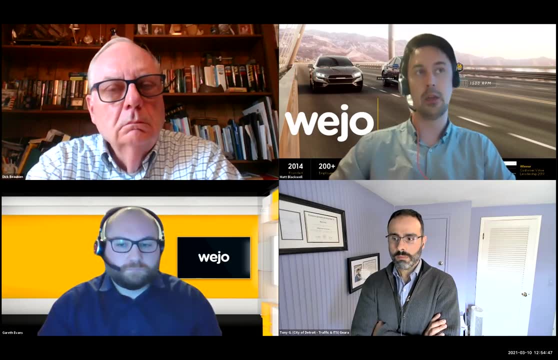 example, will have existing task orders with the agencies and with the municipalities that they will they will use to procure new data sets. now, probably a good example of this would be the the traffic management center um example i mentioned before, where we actually worked with a third party. 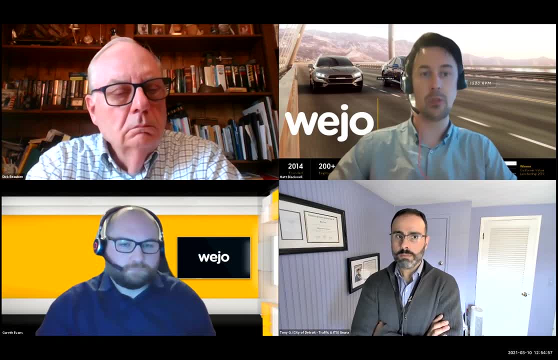 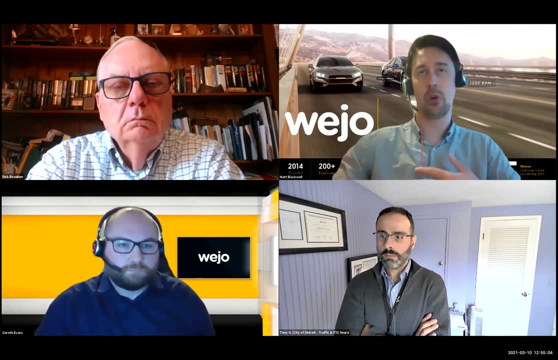 um civil engineering firm and we actually worked with a third party um civil engineering firm and to be able to visualize that data within a dashboard and utilize that real-time or near real-time feed from the weed- your data. so we we have experience of working both directly and also. 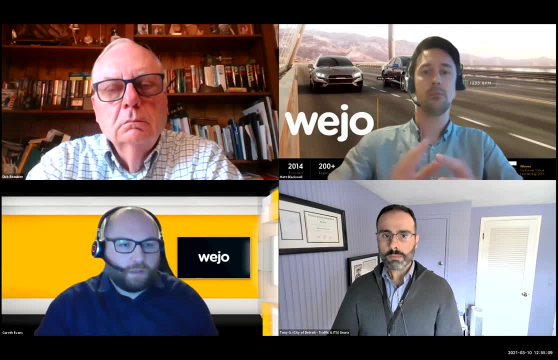 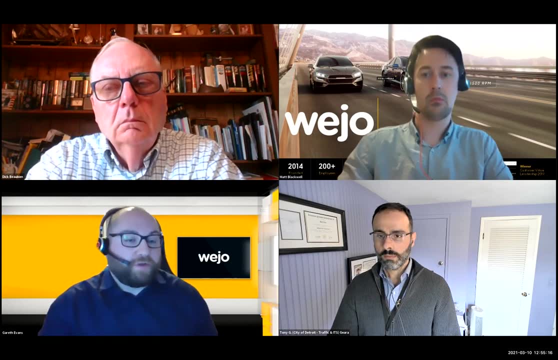 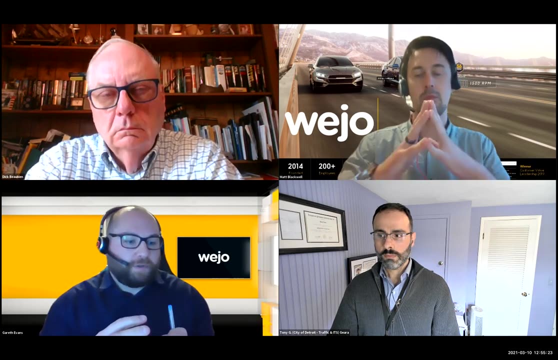 by proxy with a lot of the agencies, yeah, and in terms of of have how it works from a commercial perspective, um, it does absolutely depend on the various projects. so we've worked with some state agencies where you know it's the they want to work on, on um, on basically, they make the decision on. 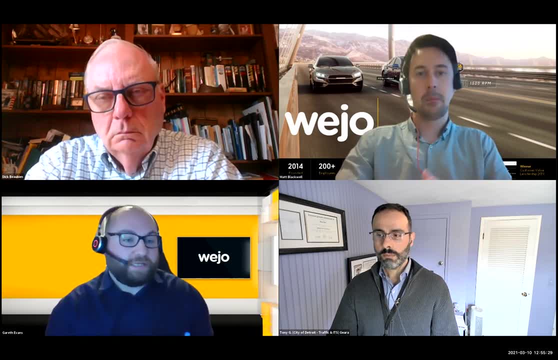 on um on. basically they make the decision on on um on. basically they make the decision on on the historic data that they've seen. so they've purchased a block of historic data from us and they'll run their own analysis and then they- you know, they then may take up the option to then. 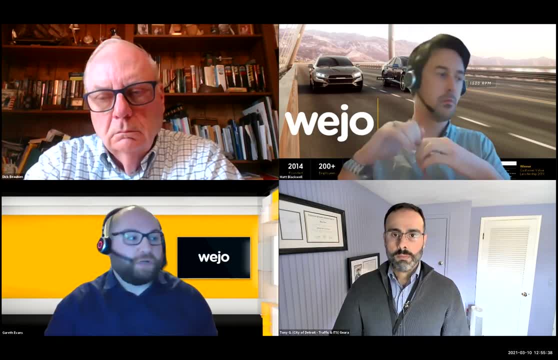 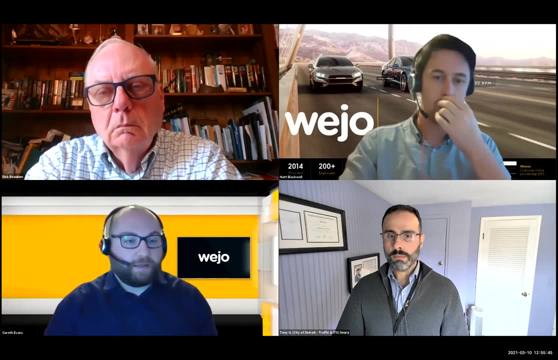 receive data ongoing and then for other agencies it's very much been on, let's say, a live subscription. so they've, you know, they've signed up for six months to get a live data feed of wejo's data into their um, into their other transportation departments um into the various 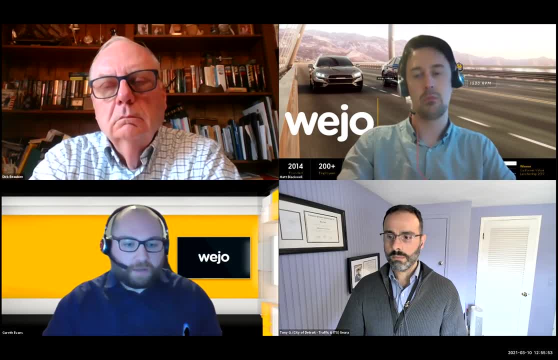 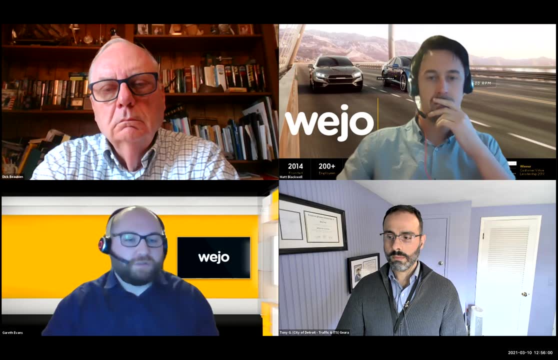 data analytics programs that they have. so this is again, hopefully, the great aspect of wejo: we have that flexibility. it's not a restricted, you know, contract. it's not a case of you have to sign up for wejo for two years. you can only have ongoing data or you can only 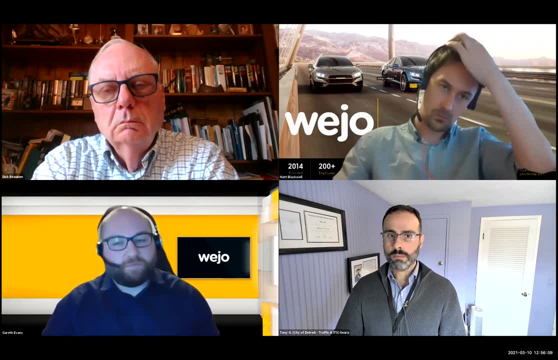 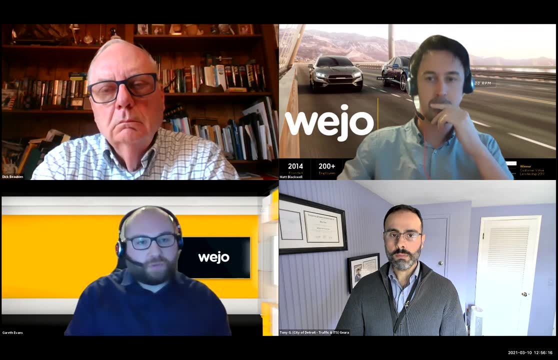 have historic. we're flexible with the needs of of, you know, of anyone that we work with across any marketplaces. you know, if you want a, you know, for the safe, we use detroit as an example. if the last 12 months you know like say that, let's call it the covid data, if you, if the last 12, 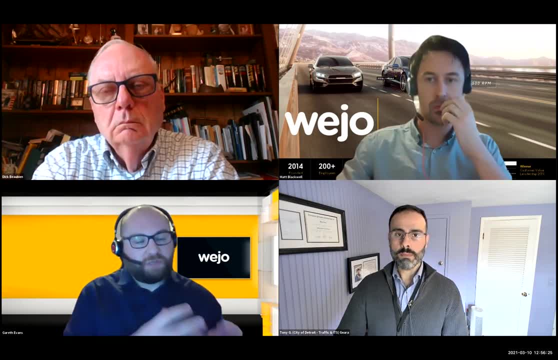 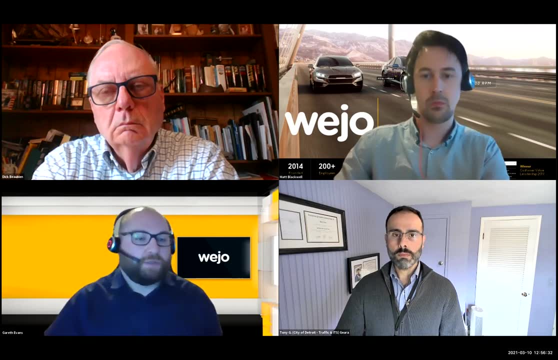 months of historic data would be of real interest for you, and you can utilize it, but then you'd also like six months of ongoing data delivered to you every single day. we can also supply that, so we're not restricted on geography. i'm obviously not restricted on how someone would like to obtain. 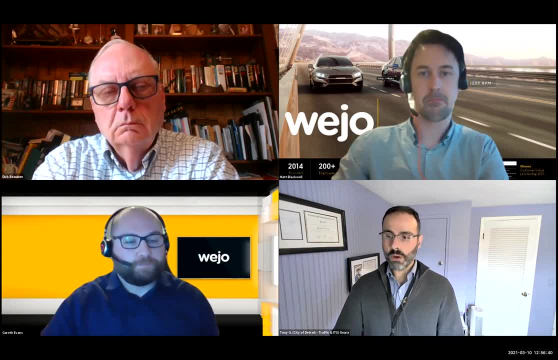 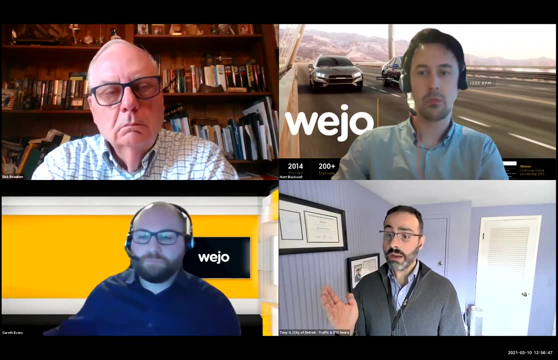 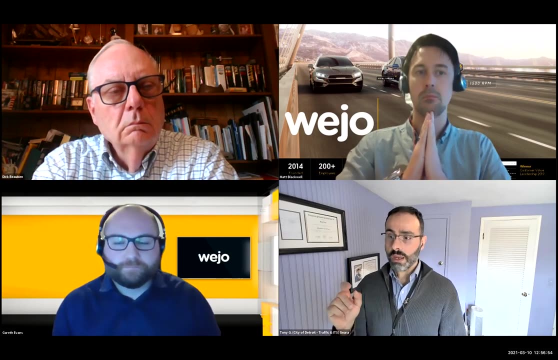 the data from us either. excellent, so i'm going to go back to hassan's email from earlier. um so, he was talking about the latencies essentially. so he asks: i understand data needs 60 seconds to reach the traffic agency. does it reach the agency in the 60-second bin? also in real-time traffic operation scenario, any plans? 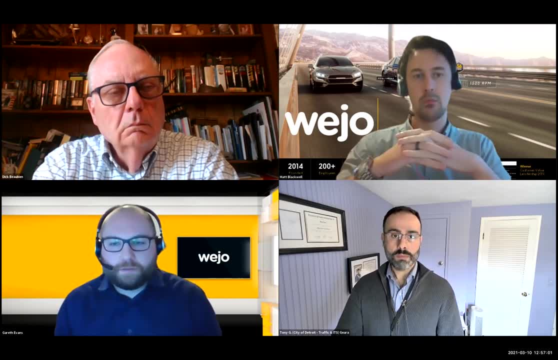 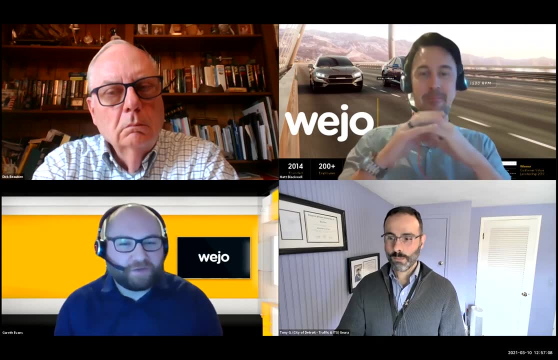 to drive the 60 seconds down to a lower number. so this is i was gonna. this is where i might say some numbers and matt will correct me here, but from what's uh for the latest conversations i've had. so the 60-second sla is is what we have, that's what we commit to and what we commit to our 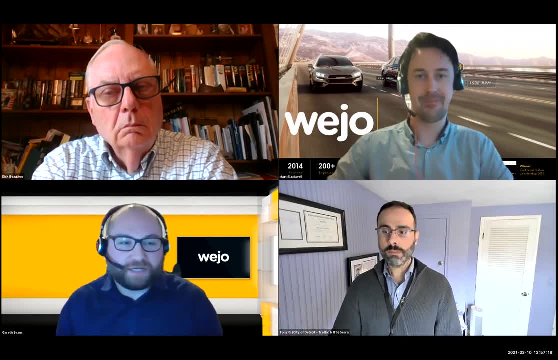 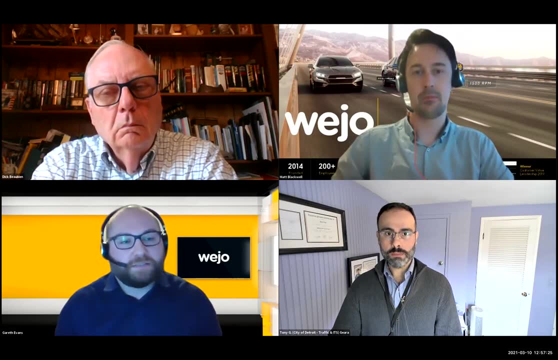 clients to, typically at the moment. so this is where matt is going to start shaking his head at me. but typically at the moment, around about 80 to 85 percent of the time, they're going to send a 60-second sla to the agency within 20 seconds, but we do have a 60-second sla in place. 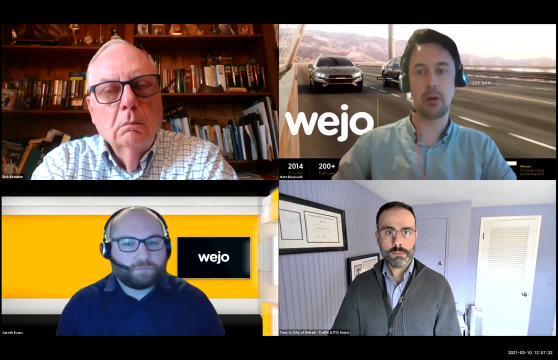 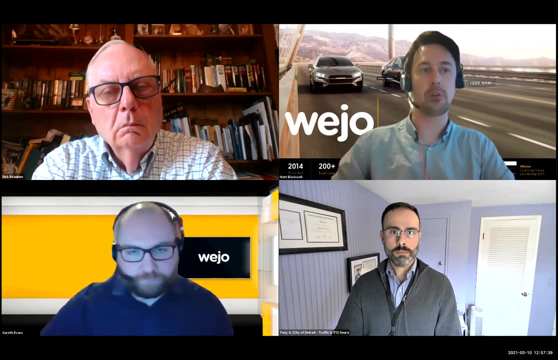 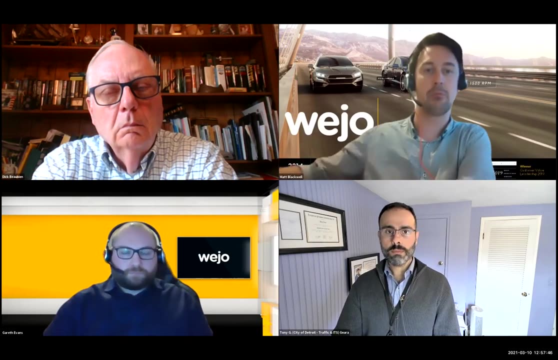 yeah, and the probably just the original part of that question around. does it reach the agency in 60-second bins? um no, so that it's not sent in a long term as a kind of micro batch where it's stored up for 60 seconds and then sent? it's sent as it's sent on a on a regular stream from the. 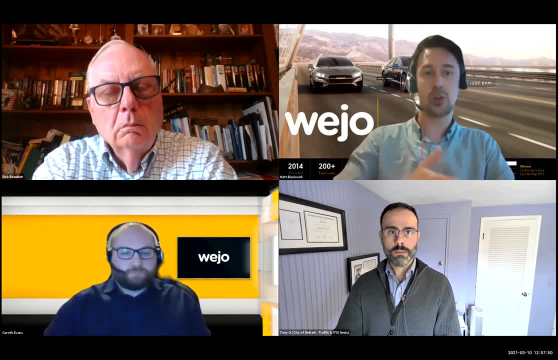 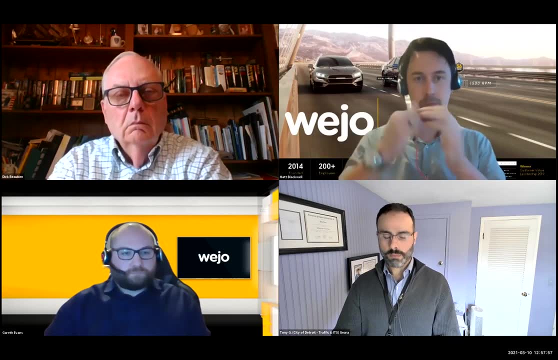 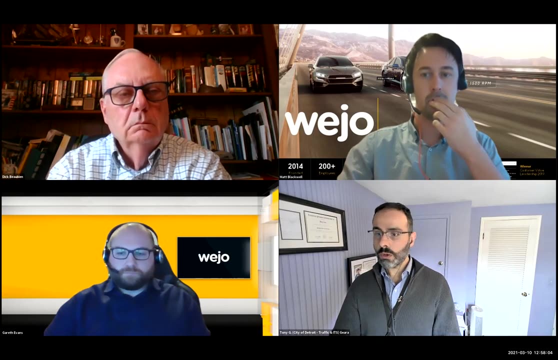 vehicle. so at the point when that vehicle starts its journey, it's captured every three seconds and it sends within 60 seconds of that data point being generated. great, great that, uh, that actually clarifies it, thank you. so, um, next question from john abraham: um, so, he's just clarifying that you know who are you working with in terms of the oems? 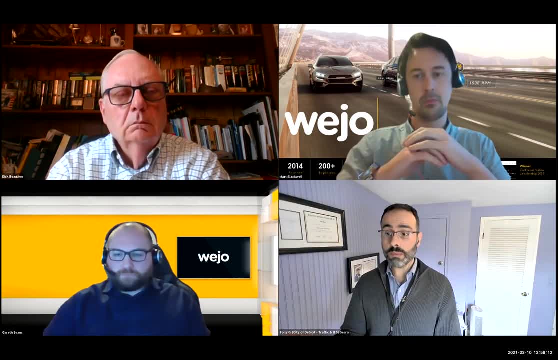 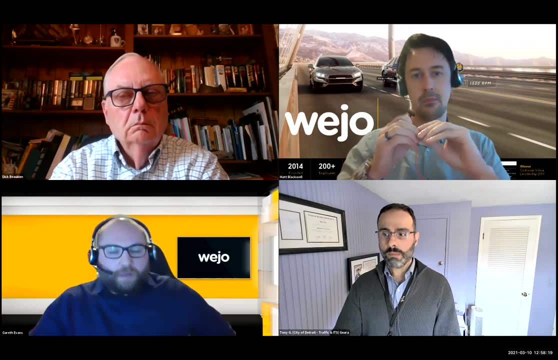 um, i'm assuming your partners include the big three oems in michigan and other major ones as well. yeah, so we thought we we can't name who they are. um, so we thought we can't name who they are on the call. what? what i can say is we work with one of 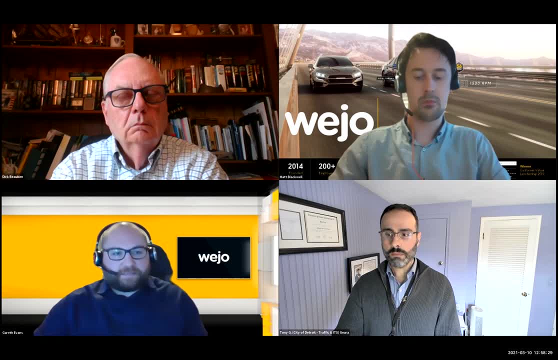 the, the largest car manufacturers in the united states, and the, the other one that we have live on our platform at the moment, is a prominent european manufacturer that has a strong presence in the united states. all right, fair enough, we won't push you more on that, so, um yeah. 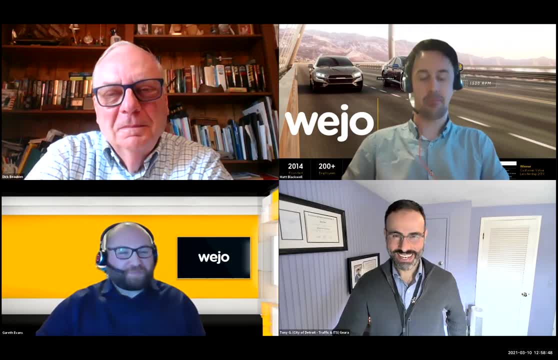 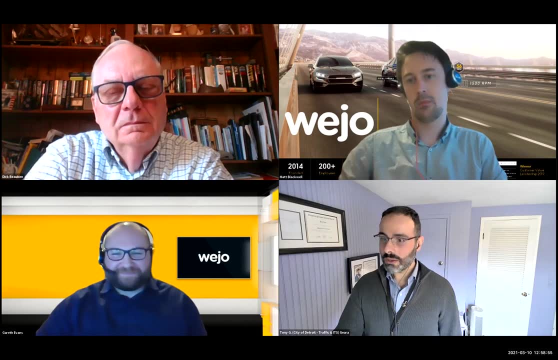 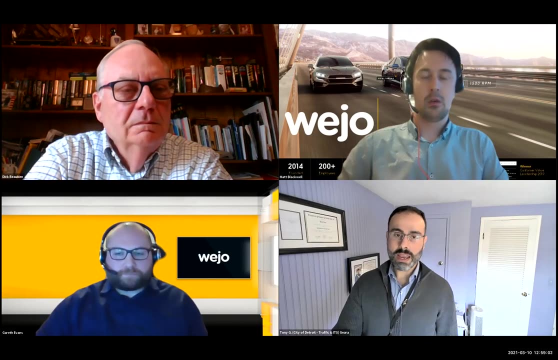 and more to come. that that's the. uh, i'll close it out. sounds good. so, um, uh, yes, again, always ask the difficult questions. uh, so i said 150 000 unique vehicles in detroit. i guess i would be concerned that some roads may not be driven on at all and we kind of saw this or had a. 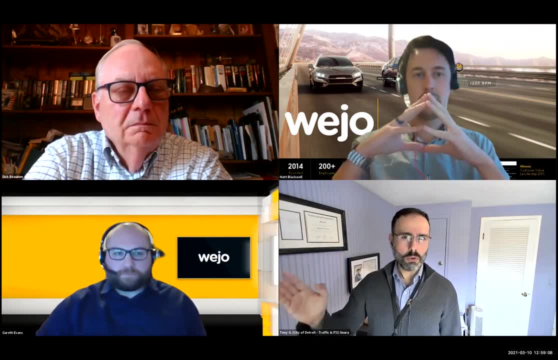 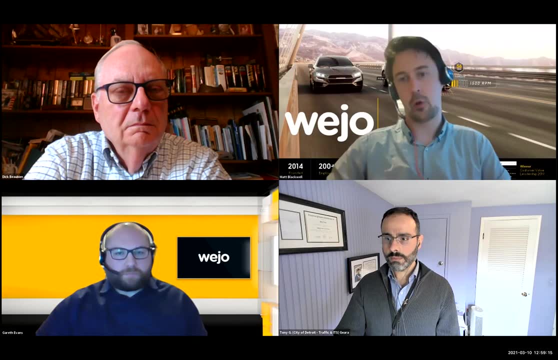 discussion about this when we were trying to find the speeds on our local residential roads, so i'll let you guys speak to that a little bit. yeah, i mean probably. just i think that the question itself is so. i think you said 150 unique vehicles. just just to clarify, it was 150 000 um rather than 100. 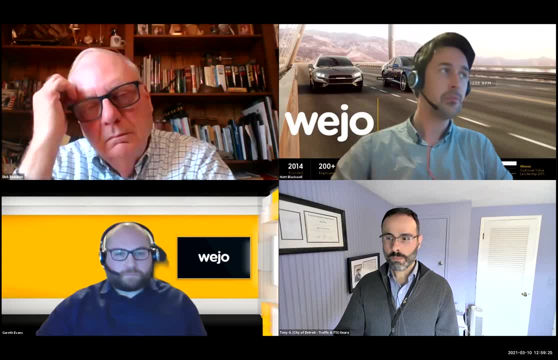 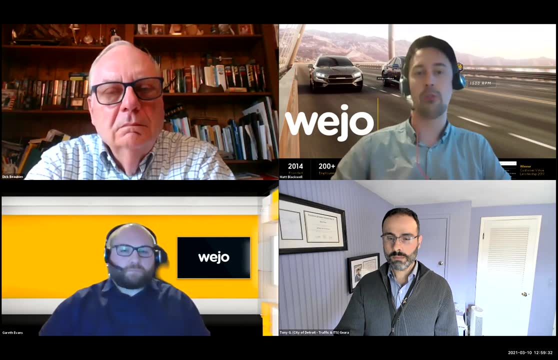 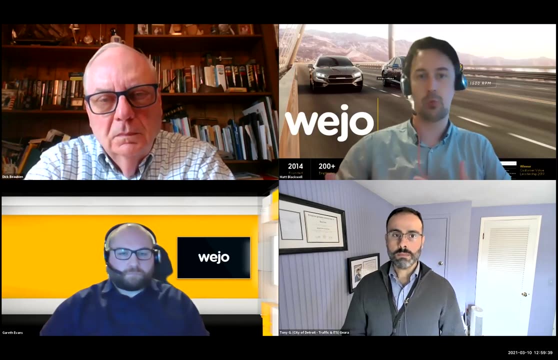 150.. The one thing we would say is: we have representation on around 95% of US roads. So when I say representation, we see at least one snapped data point on a road in a one month period. Now, obviously, when you start to look at rural versus urban, that sway will go slightly. But 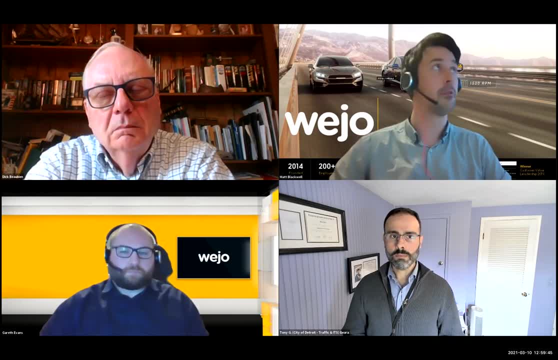 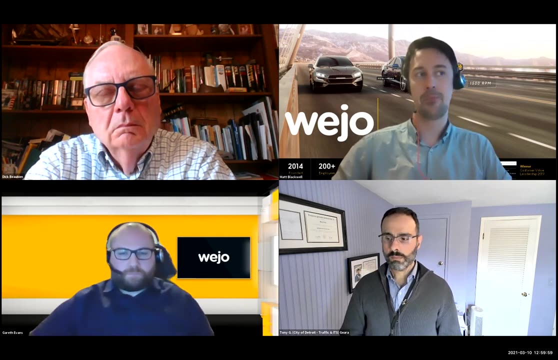 even in some of the lowest areas. so I think, from memory, Petroleum County is- for whatever reason it's- our lowest area of density in terms of the data set, And even there we are able to visualize the road network very, very well. So I think that the key thing here is where you start. 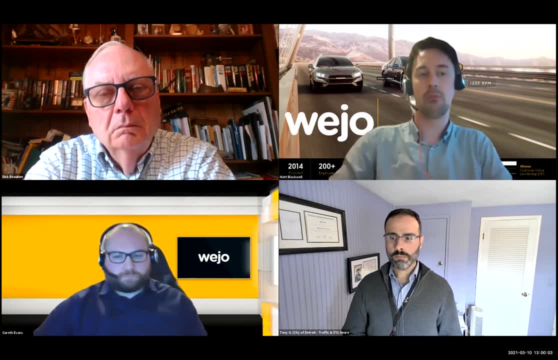 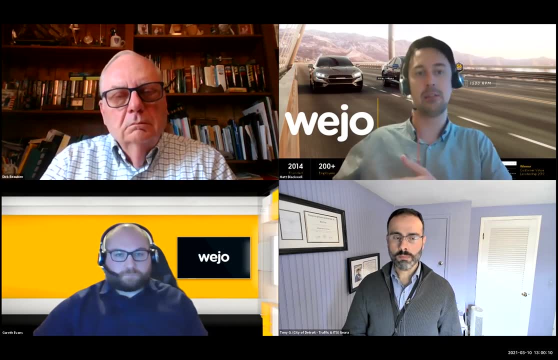 to look at actual physical infrastructure and managing traffic congestion through roadside units. it's not viable to have that at every point during a corridor, Whereas with the data even being able to visualize half a dozen vehicles along an entire corridor is a lot more than it's capable at the moment. 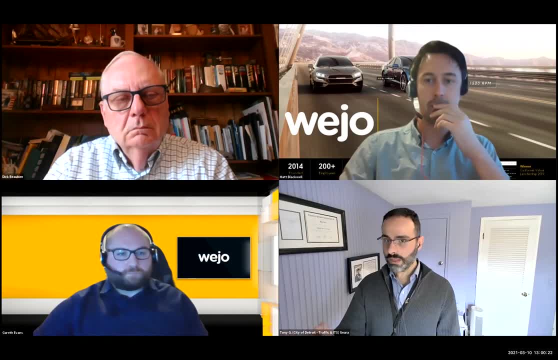 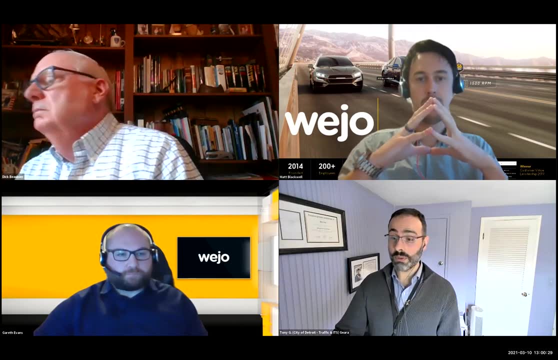 Okay, great, So we have a couple more questions. I do want to remind our attendees that it is one o'clock. Please feel free to stay. We're going to try to answer all the questions And maybe, if you want to type in some more, or if you want to unmute yourself and ask the question, 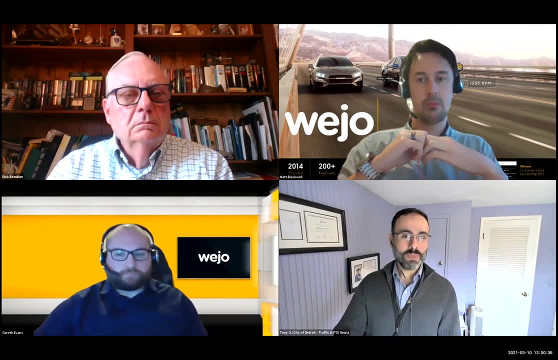 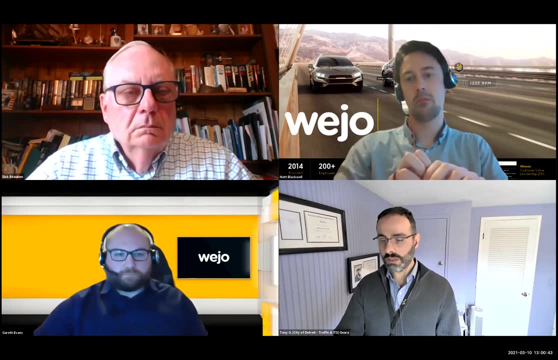 directly. we'd be more than happy to do so. So far we have two more questions, but there may be a couple that will trickle in. Our next question is from Steve Ramius, Dr Steve Ramius, from Wayne State University. From the planning origin, destination perspective. 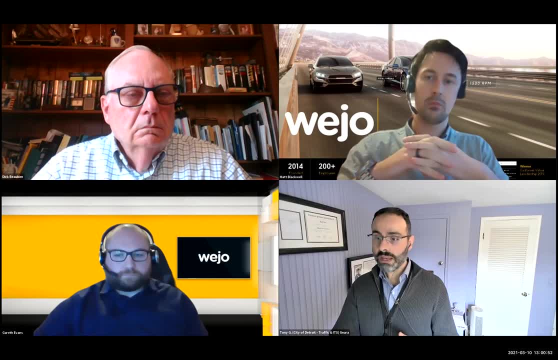 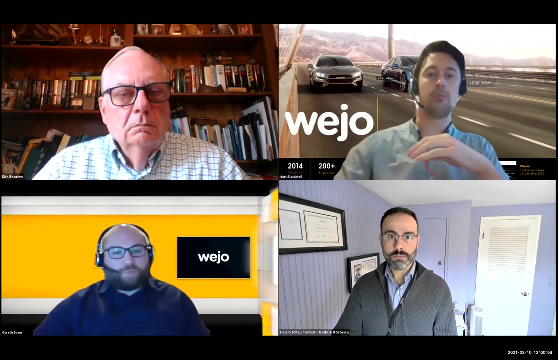 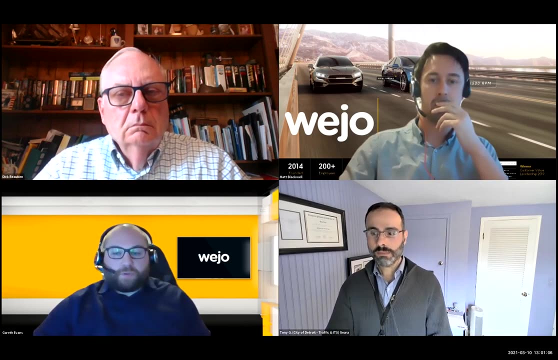 when do the waypoints begin and when do they end? Is any clipping, filtering done at the beginning and ending of the journeys? So that, do you want me to go ahead with that, Matt, or are you happy to go? Yeah, I suppose. for that was it, Steve. I think I asked that question, So that will depend. 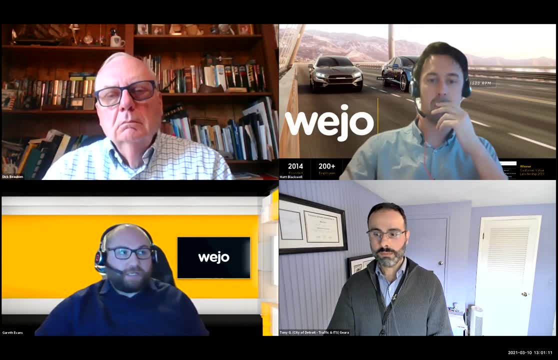 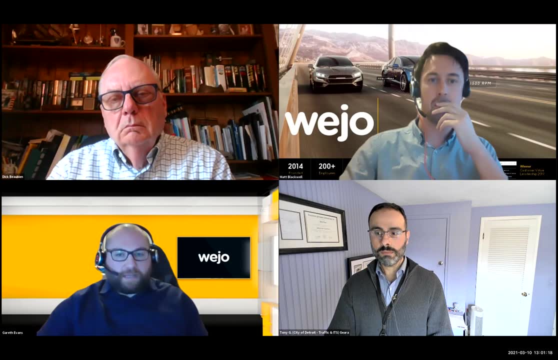 on the output of the data, So as our journey intelligence product, as an example being that is our derivative data set and there's the output that we'll have. So we can go from a zip code or a PLY set, or either or. But we only have one journey, So one. 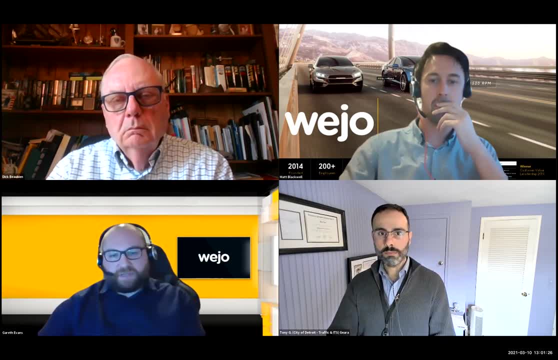 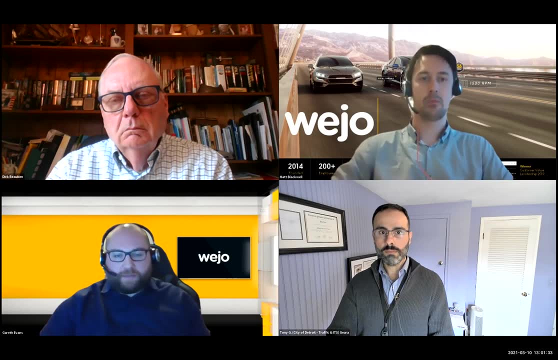 of the things that we can do is we will get down to a zip level of origin and then we can get down to a PLY level of a destination, or either or. What we would be restricted on, that is, if we only saw one journey, for example, in that area, that would be excluded from that data, that data set. So 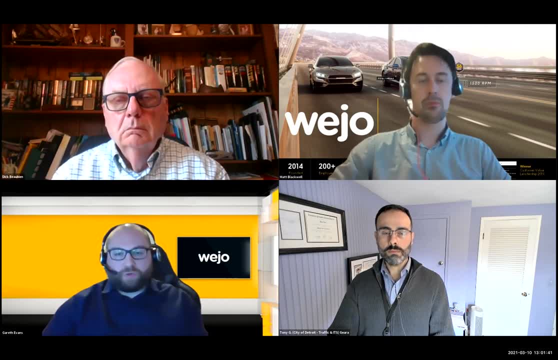 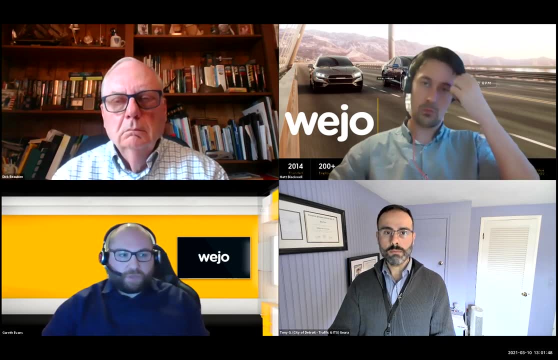 there needs to be at least two vehicles from a zip code or a PLY look: origin or destination When it comes to our raw data, because we have some, you know, an additional legal framework that sits behind the data security of that. that's when we can start to. 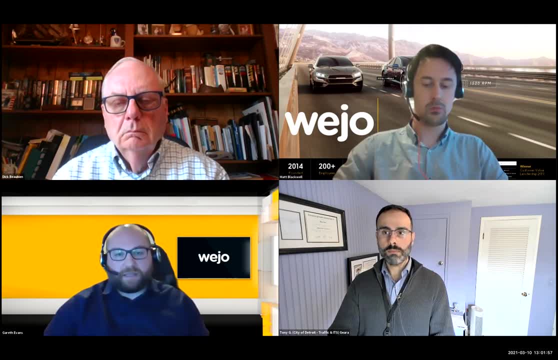 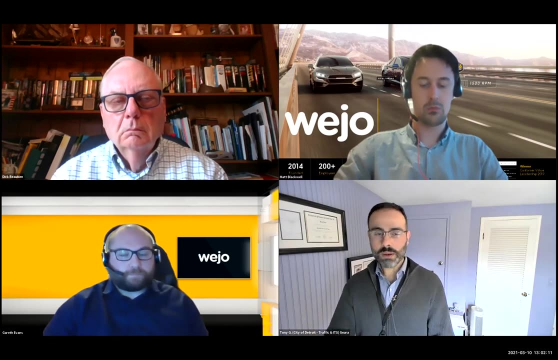 look at the, the origin and destination, to a more of a specific um journey on, journey off um long and long and latitude perspective. all right, thank you, and again i do encourage anyone to raise your hand or unmute yourself and uh chime in if you have any further question or any further elaboration that you would. 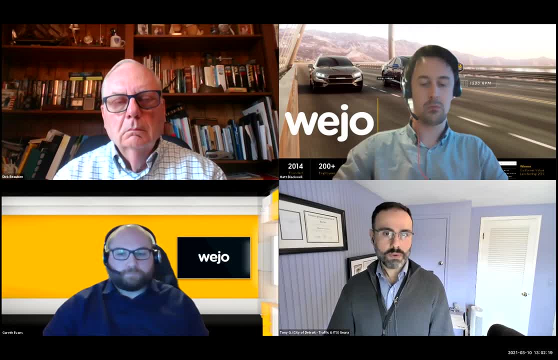 would like to add. so we also have another question from meredith, again from from mdot connected vehicle program: are you, are your customers, primarily engineering firms, local government or state agencies, which is a good question to just understand. you know where is the data being used? yeah, it's a really good question. i would say yes, they make up. 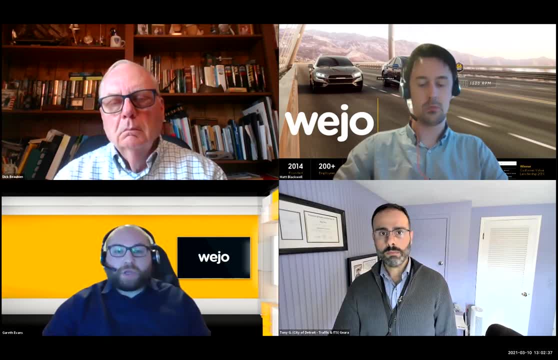 probably of the top, uh, of the top cohort of people that are utilizing our data within there as well, will for mapping and navigation companies. uh, logistic, uh, you know people were obtaining more accurate data from ouija, but, um, yes, i'd say you know they are they. 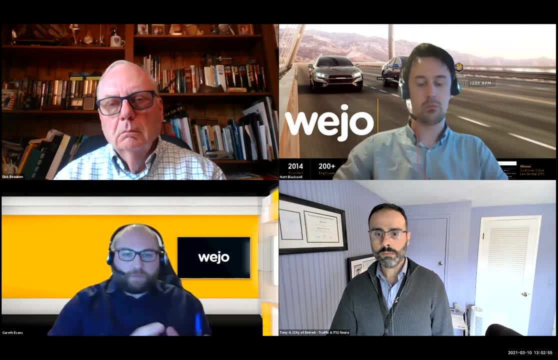 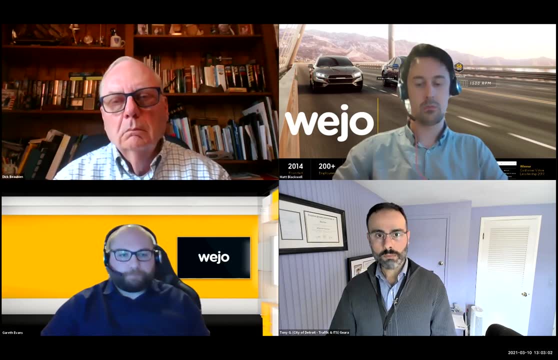 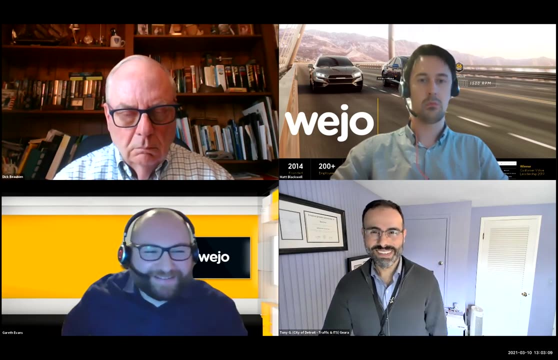 form of the top five to ten. you know that the, the, the, the end users of our data currently. yes, they would absolutely fit in that. in that, uh, bracket, very great. well, um, oh, john, please. one of the reasons i asked about the oems is basically to find out. uh, maybe the the question. 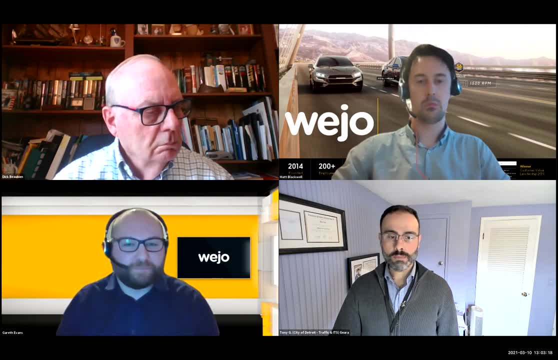 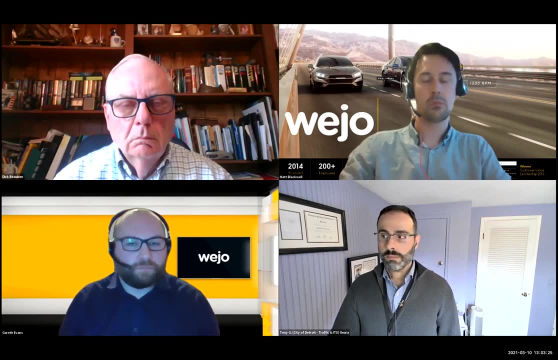 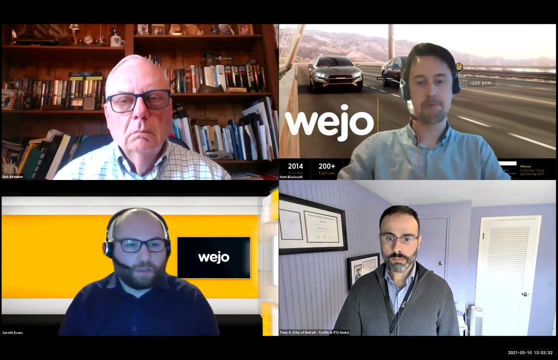 can be rephrased. just ask you: what's the penetration rate, uh, of your data? are you say covering ten percent of the? i mean using ten percent as as the statistically significant sample for your uh stuff, or uh, are you getting, say, fifty percent of uh the vehicles out there? perfectly valid question, and again, matt. 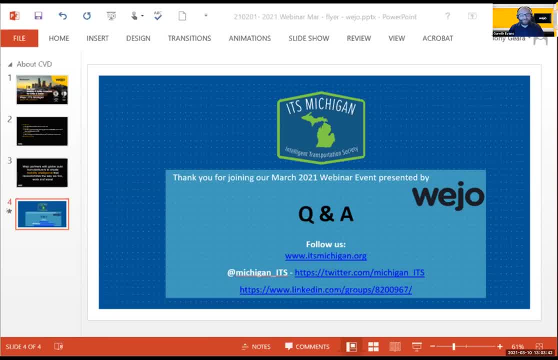 that's his poised. that's his poised uh uh expression. so it looks like matt's ready to go. yeah, i mean typically we, we say at the moment our data represents about one in every, probably 26 vehicles on the road. now, when we start to look at um- and i'll attempt to say this without stuttering statistical- 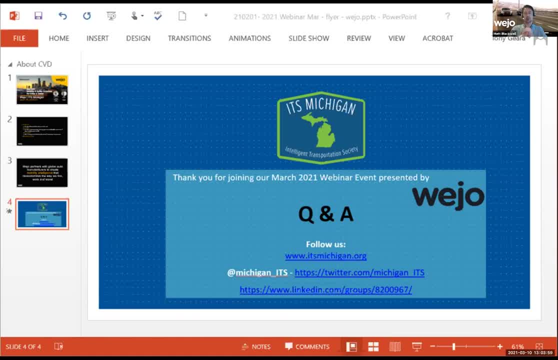 significance we typically, when i've worked with a lot of traffic engineers and its engineers, you know, anything from kind of one and a half to two and a half percent upwards provides enough significance to to accurately model against is the other conversations that i consistently have. you know, i don't. i think it's fair to say that if, unless you're using something, 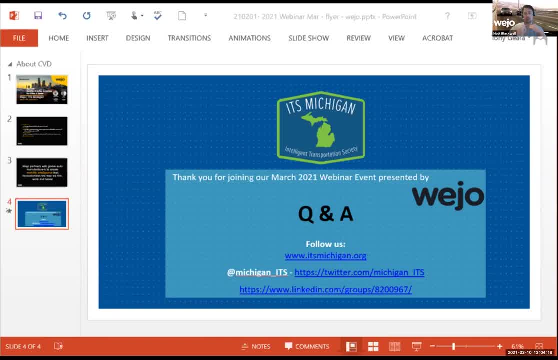 like a roadside unit, and even then, if you're using something like a roadside unit- and even then i'm actually going to say that's a, let's say, a little bit rapid normalize that you could also, you know, um, the only difference between like a roadside unit and a roadside unit is that if we draw 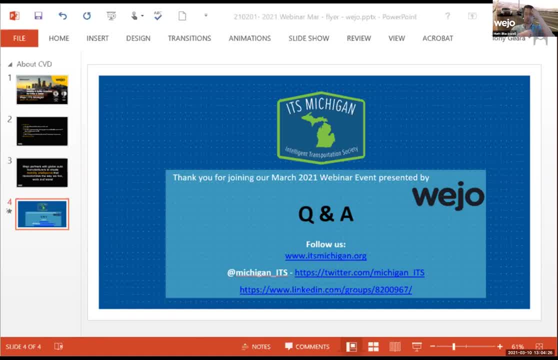 everything from one and a half percent or two of the vehicles that's going to be there. it's not going to be that, it's just a one in every one of those vehicles. so we've got to think, if we, if this is just a one in every one of those vehicles, i'll make sure that it's a one in. 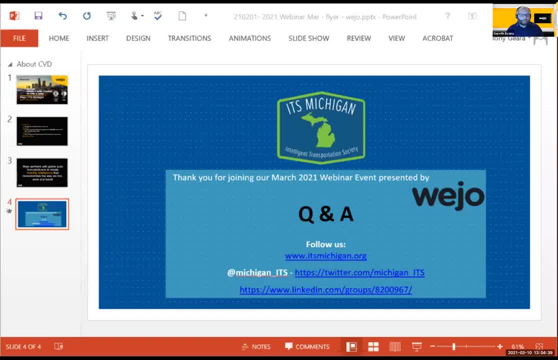 every one of those vehicles so that it's not just that one in any one of those vehicles. and that's the cost of i don't even know those vehicles. do you know? the cost of that is the cost of destruction on board. being who they are, it's their, their vehicle sales and our um, our vehicle car park. 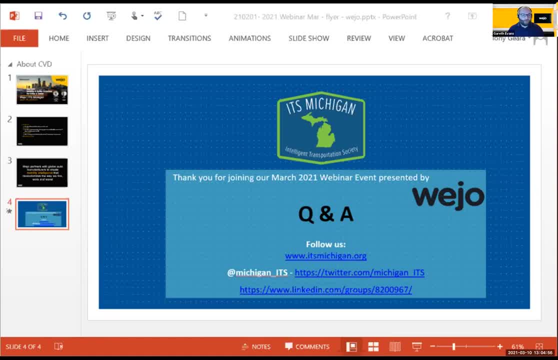 as we call it, matches very, very closely with. you know, the generic car sales across the united states in terms of the distribution you know across between pickup truck versus sedan versus um, two-seater sports car, etc. ev vehicles. that mirrors very, very, very, very closely with with. 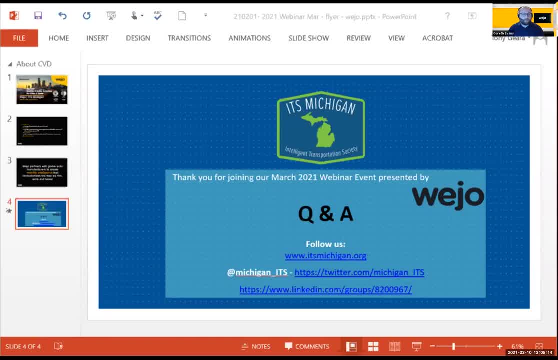 what we see from our um car manufacturers that we have on board at the moment. excellent, um, i do see a number of people still on the call. please feel free to unmute yourselves and then ask any questions. all right, so, uh, frank, were you gonna ask something? 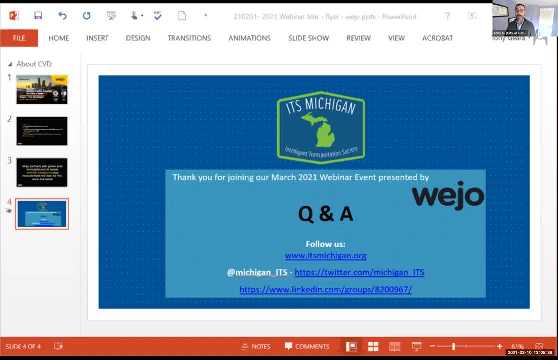 maybe not well again, thank you a lot. uh, garrett and matt, it was a pleasure having you with us. um, i know it's with the time difference. you guys are probably getting ready for bed, or so it's early. it's early for us. it's early for us, teddy, all right, well, thank you very much again. 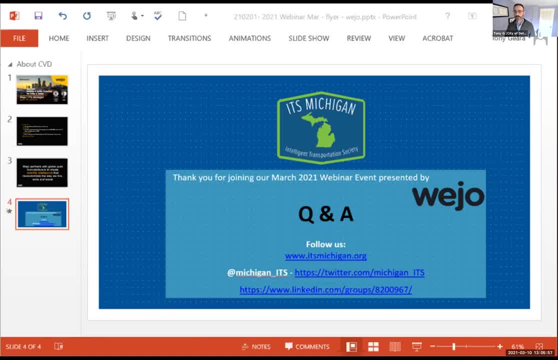 and uh, we'll definitely be in touch. i'm glad that, um, you know, this conversation started off here through its michigan again, yeah, absolutely, thanks, have a great day. thank you very much. thank you, thank you. you.